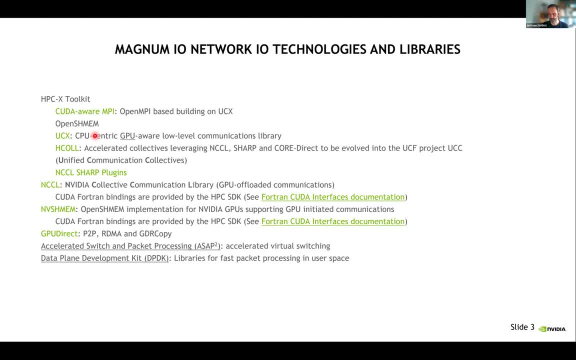 network compute that Bayer-Collector uses. that's being designed to deploy its own hardware in the Android field and it was designed for use with the protectsharp or direct, And this intended to be evolved into the UCF project. UCC, which stands for Unified. 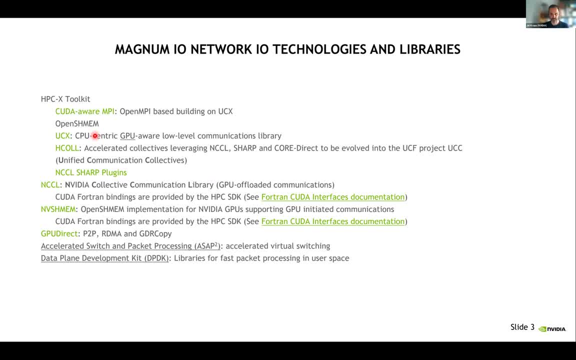 Communication Collectives, So it uses the same umbrella as UCX, and nickel sharp plugins, so that nickel can also utilize sharp for a collector. Then there's a Nickel collectives communications library where GPU offloaded communications Nv-SVAM, an OpenSVAM- implementation. 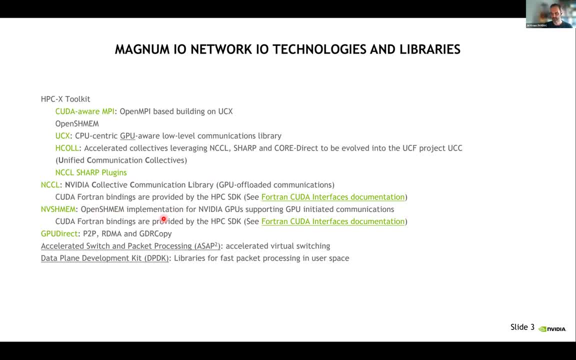 for NVIDIA GPU supporting GPU initiated communications- Next slide. So something, Something else. we have the sytuations, So we use the prat-input application And there are the GPU direct technologies, peer-to-peer RDMA and GDR copy. 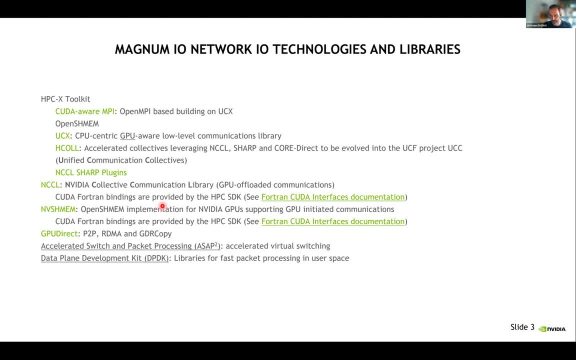 There's also accelerated switch and packet processing for virtual switching and the data plane development toolkit, where it is for about packet processing in user space. Today I will cover in different intensities on the technologies highlighted in green. I will mostly focus on MPI and how. 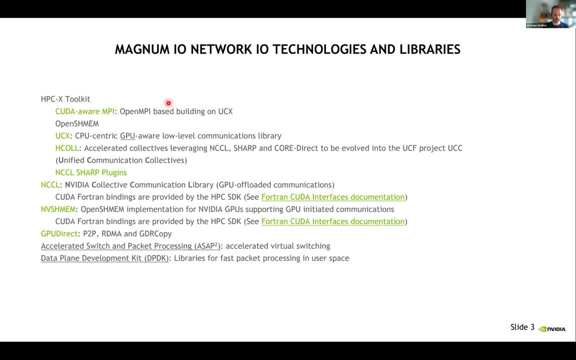 to use that from your application, because I anticipate that this is probably the most relevant for your work- how to use it with tools and how to express communication, computation overlaps and optimization tricks. But I will also talk a bit about underlying technologies like UCX: how to leverage H-COL from MPI. 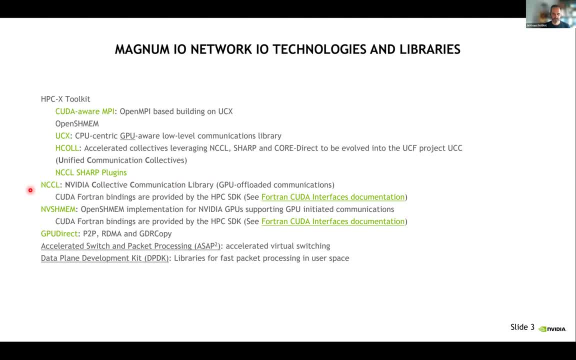 And I want to quickly start my presentation with a quick outlook on how to use NICL and NV-SMEM, because that can be, for some cases, very interesting technologies that you can explore to improve the performance of your application, And both are fully interoperable with MPI. 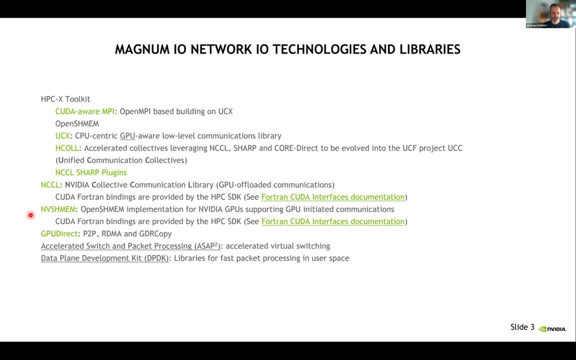 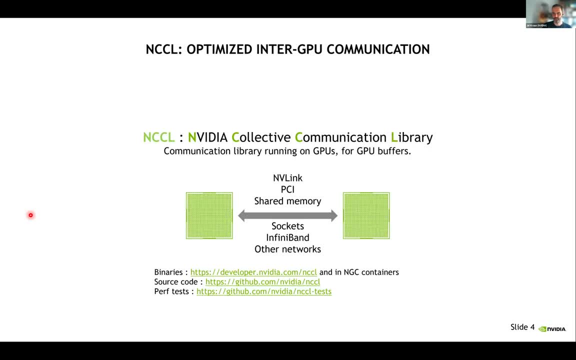 So you could. if you have an MPI application, you could just apply them at places where it makes sense. OK, so let's take a look first at NICL. I'm sure there is your. most of you have already heard about it. 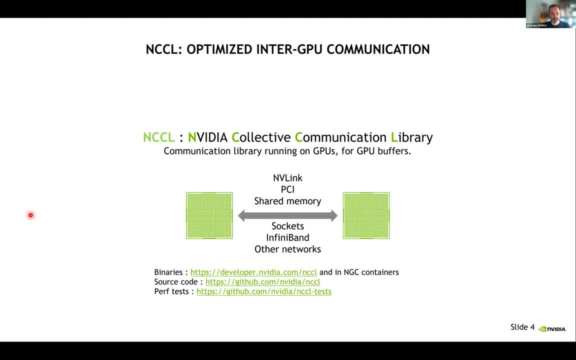 It's a library for optimized inter-GPU communication And the abbreviation actually stands for NVIDIA Collective Communication Library, because the focus of NICL is really collectives, like already used and so on. So I would say, when it comes to a GPU accelerated system, 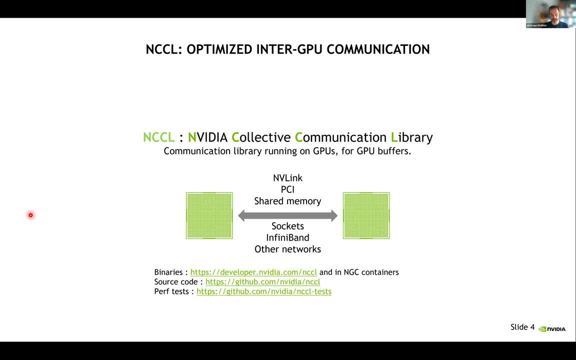 it supports all the connection that's relevant. It can move, If available. it can leverage. It can be linked efficiently, If available. it leverages PCI Express efficiently, If needed. it can communicate over shared memory. It can leverage RDMA networks like InfiniBand and also. 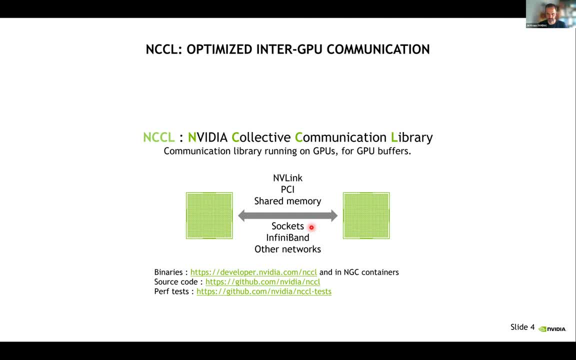 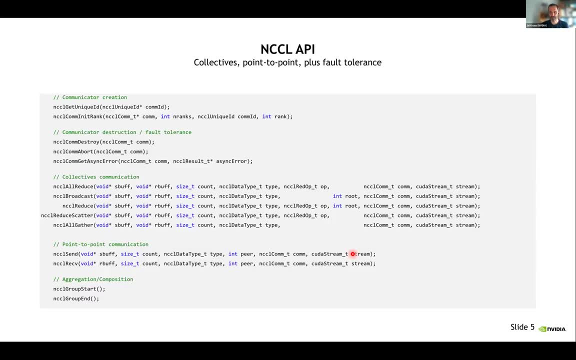 other networks And, if needed, it can even work on sockets on any network. So a brief look at the NICL API, which is probably, if you know, MPI, should be quite familiar with you. So you create a communicator which requires some out-of-band communication. 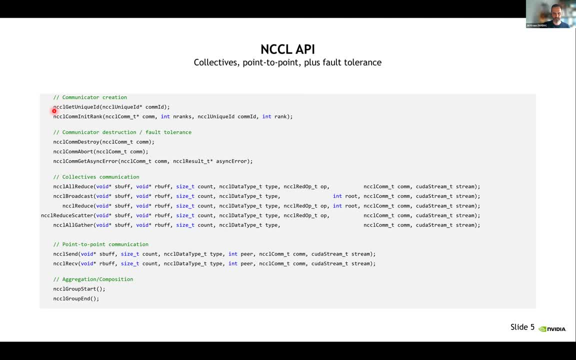 So the process is usually: root rank creates a unique ID which is broadcasted to all other ranks, And then all the NICL ranks call NICL comInitRank with that unique ID And then this communicator can be used to carry out communication. 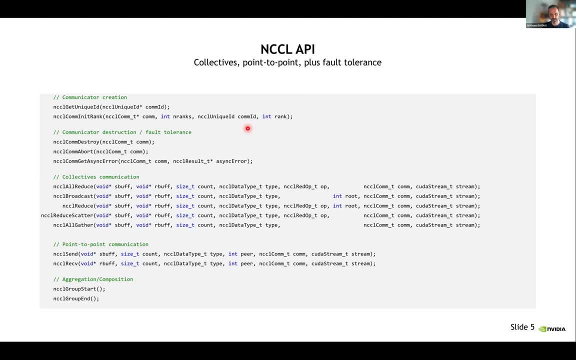 This communication is CPU-initiated but fully executed by the GPU, So the communication is supported. The communication is submitted into CUDA streams and therefore asynchronous with regard to the CPU launching that operation, but bulk synchronous with respect to the stream, So every compute work launched in the same stream. 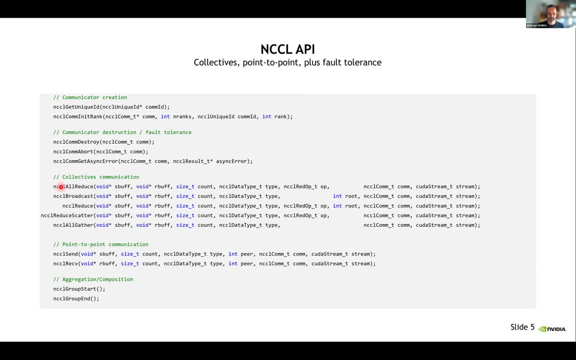 will finish before a NICL operation has started and no other GPU work will start submitted to the same stream that before the NICL operation has OK, Completed. So there are collective communication routines- just a selection here which you can see- which are modeled closely after MPI collectives. 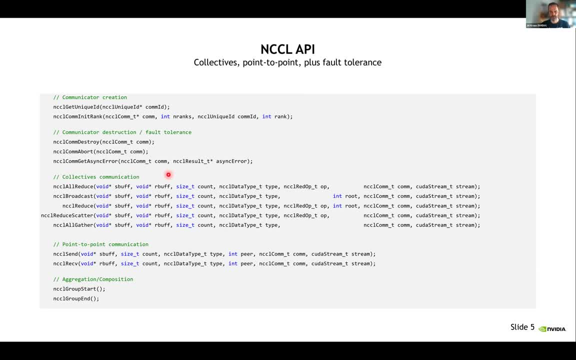 so should be familiar to most of you, hopefully, And a relatively recent addition is also added point-to-point communication APIs, which are very similar to MPI point-to-point, which can be used to express all the communication patterns not directly expressed by a collective. 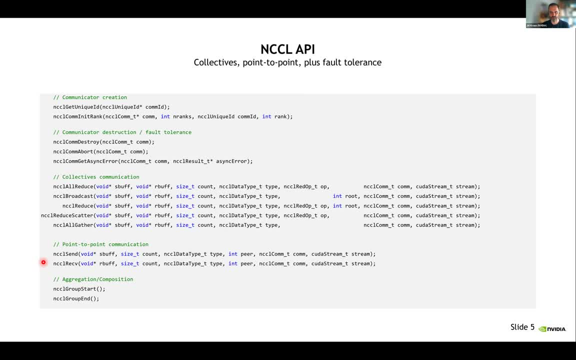 So, yeah, I'm just using send-receive. So why is that potentially interesting for you? Because in some cases you can, as you will later see in examples. you can organize your compute and communication more efficiently if the communication can follow stream cemented. 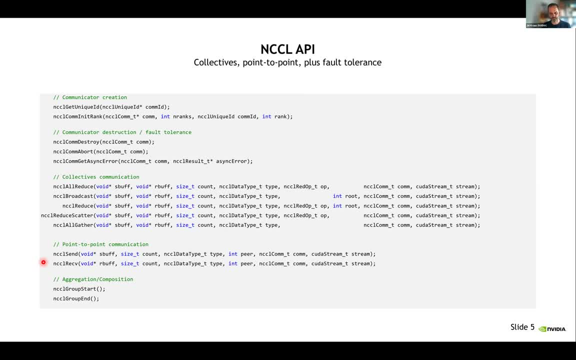 so that you can prepare a communication step that should follow after a kernel, while the kernel runs. That is something that OK, OK Nickel allows you to express, because you can launch the kernel while that runs. you submit to the same stream the nickel operation. 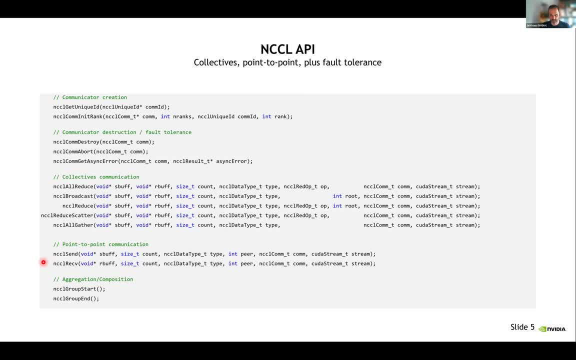 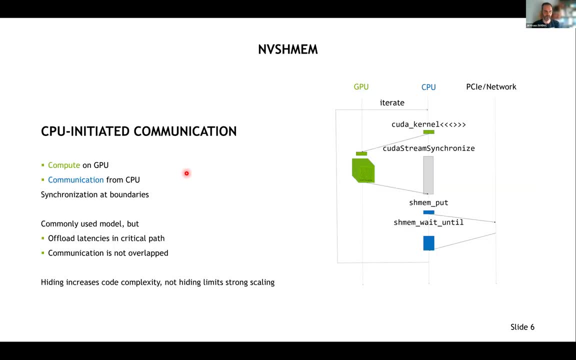 for the communication that should start immediately after that has finished. The other technology I want to touch on before diving into MPI is NB-SMEM And for motivation. so if you're consider, for example, MPI and CPU-initiated communication, we have the mode of the CPU launches. 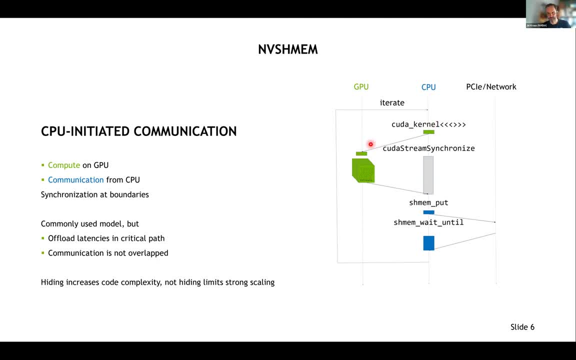 the CUDA kernel then control transitions to the GPU. The CUDA kernel is executed, The CPU synchronizes the CUDA kernel and then the CPU carries out communication on the data modified by the GPU kernel. So we have two times a context switch from the control flow. 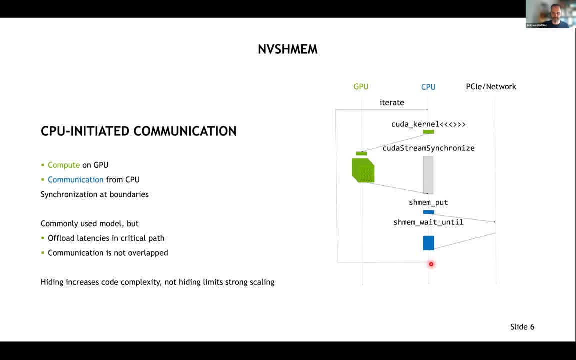 going from the CPU to the GPU and then back. then probably in the next iteration again. So we are synchronized. We always need to synchronize in the communication and compute boundaries which is very commonly used, And this is also the model that you're. 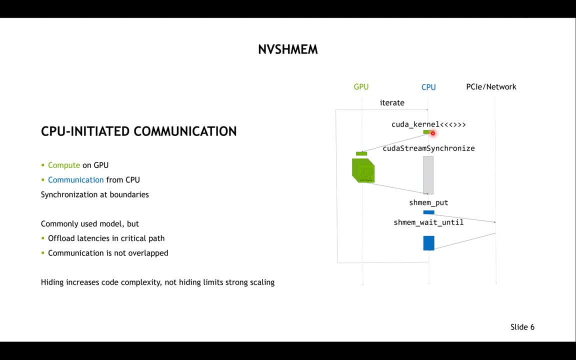 doing with MPI when you combine it with different programming models, as you will see later. But the problem is that it puts these synchronization and launching kernel stuff on the critical path of the application And you don't get overlap between the communication and the compute. 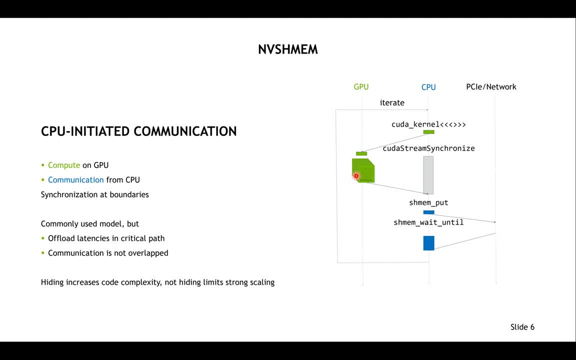 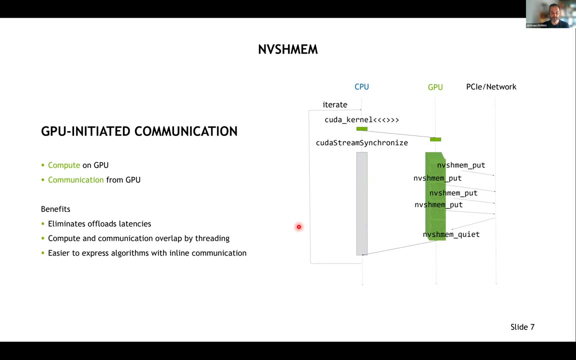 So not the maximum efficiency. You can get overlap, as I will show later by the example of MPI, But it definitely adds complexity and also some overheads. With NVHRAM you get enabled to do GPU-initiated communication so that you can do the compute on the GPU. 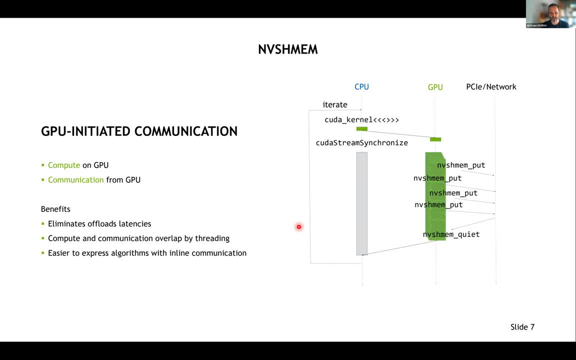 And as soon as data is computed you can initiate communication on it. So you would launch a kernel That computes and issues, for example, put operations, And that minimizes the offload latencies because you have to launch fewer kernels, have to synchronize less often and there 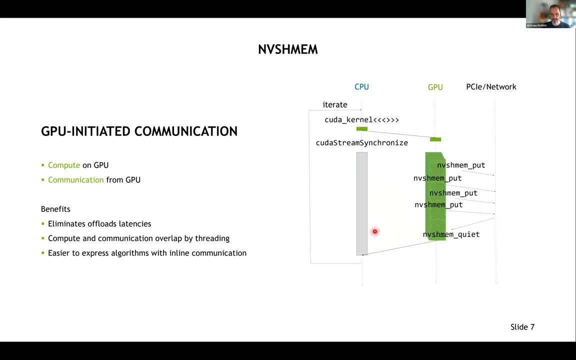 is no context switch between the CPU and the GPU. It also in case because this communication can be relatively fine grained. it gives you communication computation overlap by threading. So you get the same benefit of latency hiding for inter-GPU communication as you get of latency hiding. 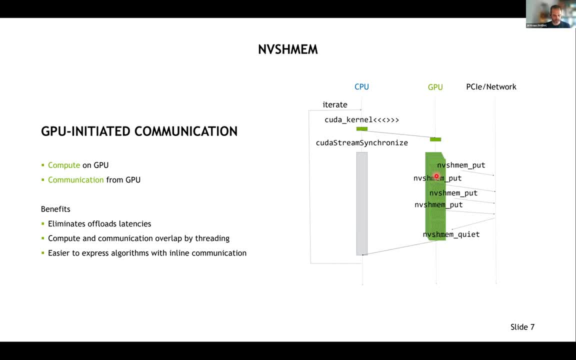 with just regular memory accesses from the GPU, As you've been introduced before. if you use a GPU, you're vastly oversubscribed. You're each shared multiprocessor in the GPU with many threads, so that if one thread waits for data, another thread computes. 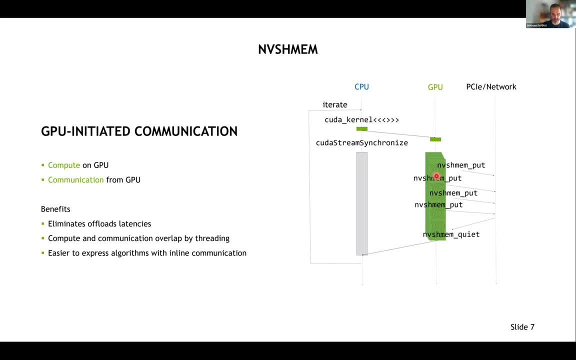 And with NB-SMEM and GPU-initiated communication. the same works there, And sometimes it's easier to express algorithms with inline communication. Since that is a bit far away from MPI, where I assume most of you are familiar with, I want to show some brief code examples how it looks like. 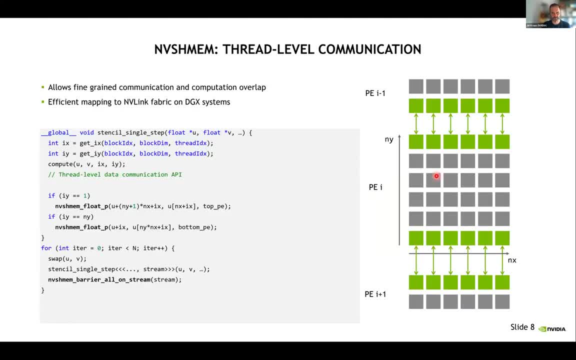 So the most fine grained way to communicate with NB-SMEM is thread-level communication. So as soon as a thread has computed a value and it knows a neighbor needs it because it's computing something on the boundary, the thread just puts that single value to the neighbor that needs it. 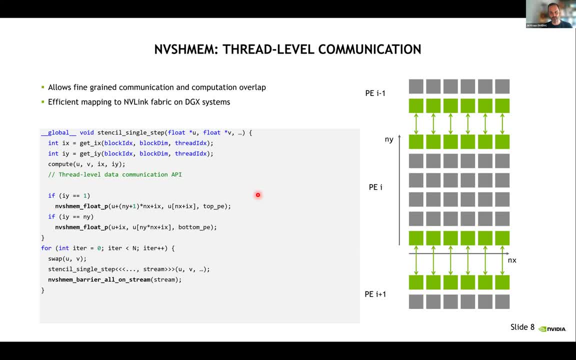 So we get a very fine grained communication And if it's running over, and if that communication happens over NB-Link, it's also running very efficiently because, like memory, this will effectively be mapped to load stores And the load stores will be automatically coalesced. 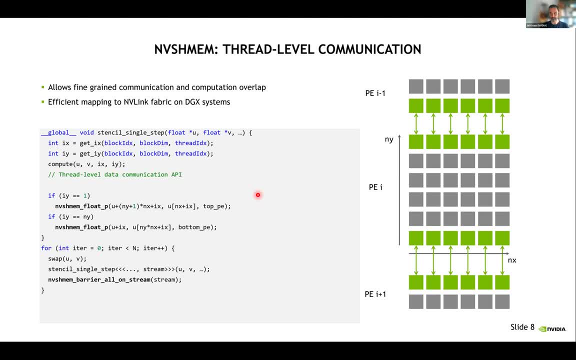 like memory accesses in the GPU. On networks like InfiniBand this is a bit too fine grained because for every individual request we would need to generate a network packet, which has too large overhead for very small packages. So it's also possible to cooperatively send large. 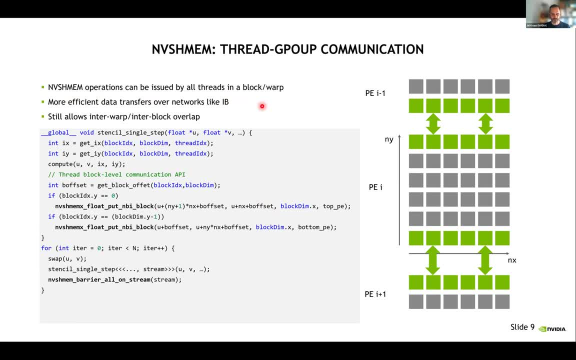 larger blocks of data And that works more efficient over networks like IB. In this case again, compute is the same and you don't need to leave the kernel. But now you just see: hey, am I a block that has data to communicate? 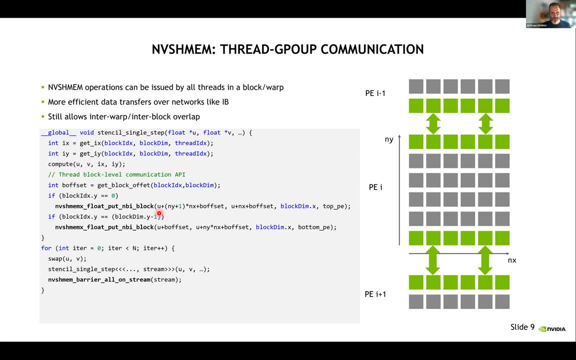 And then all the threads in the block call into such a cooperative thread group communication API to send- hey, immediately after it's computed, the data of the whole block to the receiving PE. So that's a benefit that gives you a transparent GPU communication computation overlap due to threading. 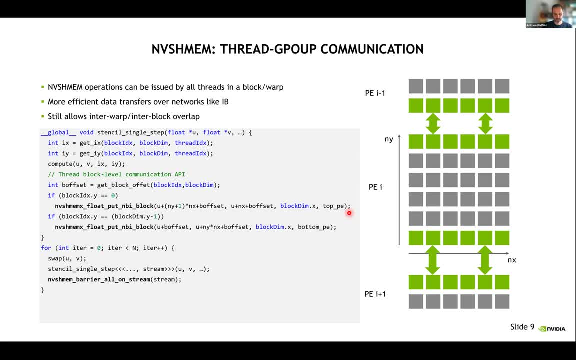 It also minimizes the number of GPU kernels you have to launch and centralization points. so just moves CUDA API out of the critical path. So already very good. but with GPU-initiated communication you can even get one step further and that is move also the iteration, the synchronization. 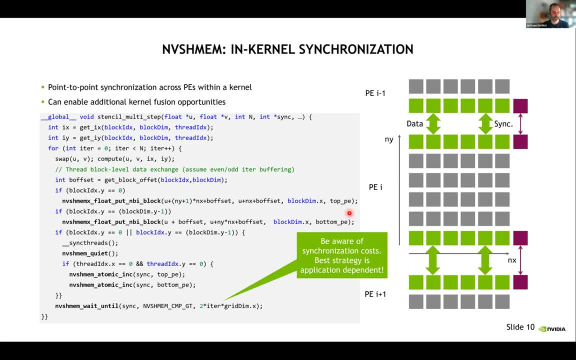 into the kernel and therefore, for example, an iteration. This sometimes can be very powerful because it allows you to merge kernels which are interleaved with communication, which would not be otherwise possible, And by merging these kernels you might be able to keep. 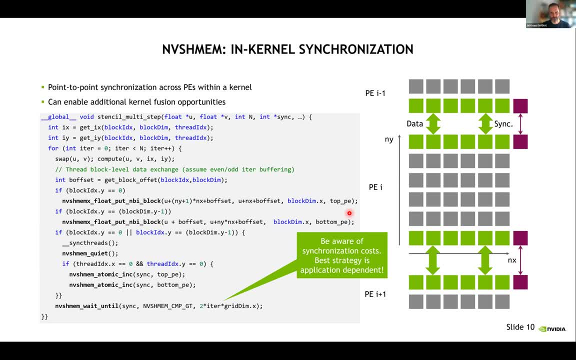 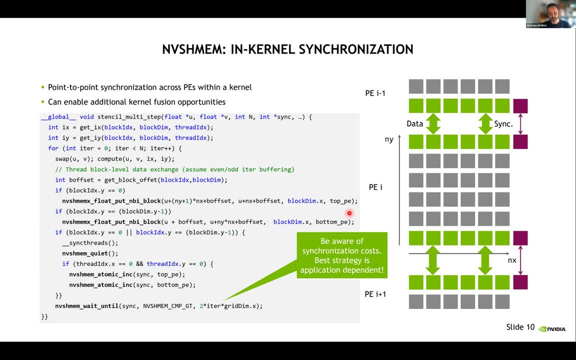 to the GPU's global memory, or you don't need to write shared memory out to the GPU's global memory from one iteration just to reread it in the next. So that can sometimes, if it's applicable, be really significant performance improvement. 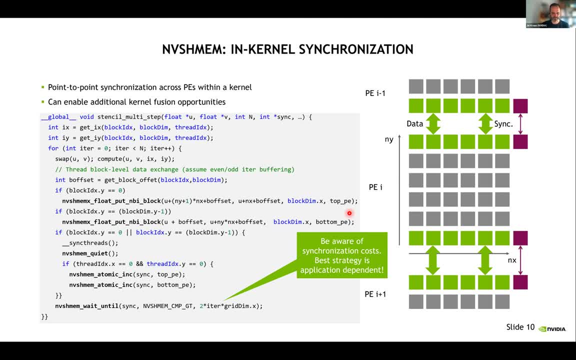 not so much because of more efficient communication, but because of the fact that inline communication allows this whole state closer to the recently process for a longer time. Communication used here is the same, it's just that pointing out that you can put the full kernel there and that NB-SMEM provides API to synchronize. 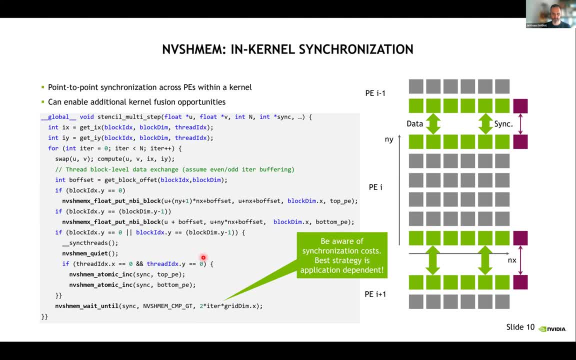 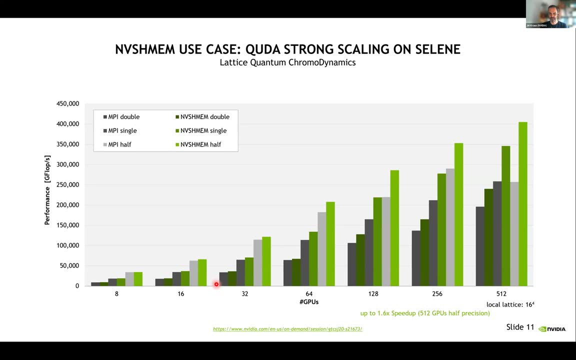 between processes. Just pointing out here: the right synchronization strategy largely depends on your algorithm and also the system you're looking at. Okay, so before jumping to MPI, a motivating example for NB-SMEM. I've chosen CUDA, which is a library for algorithms less relevant in lattice QCD simulations and with this field, strong. 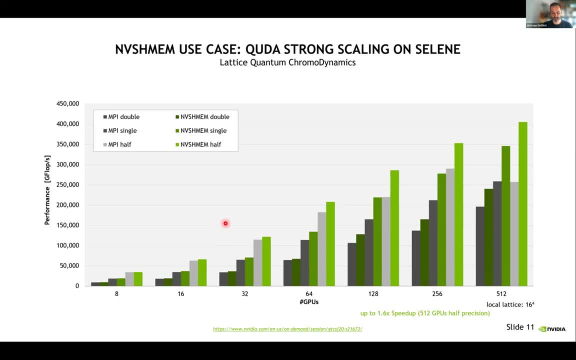 scaling is very important and here this is a benchmark executed on the CELINE supercomputer at we have at NVIDIA, and we scaled from 8 to 512 GPUs, with a local lattice size of 16 to the power of 4 in case of 512 GPUs, and compared MPI to NB-SMEM in different precisions and 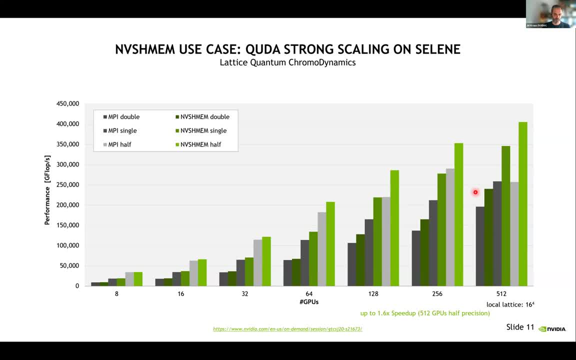 so the smaller the data type used, the more latency critical the application becomes and the more communication bound. So we see here that NB-SMEM greatly reduces, helps to reduce that overhead and achieve better communication computation overlap because we see an up to 1.6x speed up at 512. 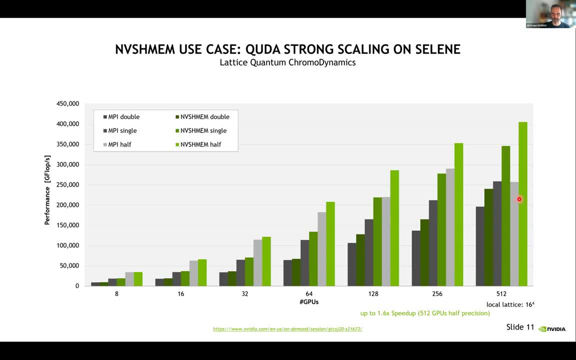 GPUs with half precision when comparing MPI and NB-SMEM. and yeah, as a reminder, there's no need to rewrite your whole MPI application to NB-SMEM or NICL. it's fully into operation and you can just apply it all the places where it makes most sense. 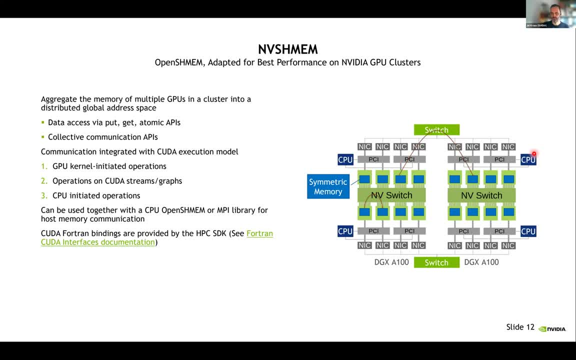 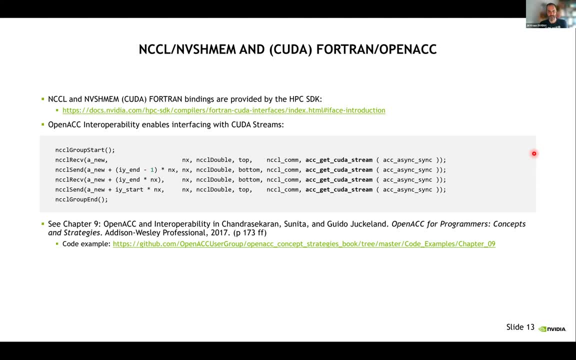 Yeah, I'll keep that here as a summary of NV-SMEM for further reference, And also want to point out that, yeah, the nickel and NV-SMEM, they are fully- yeah, as I said already, fully- interoperable with MPI. There exist Fortran bindings for both. 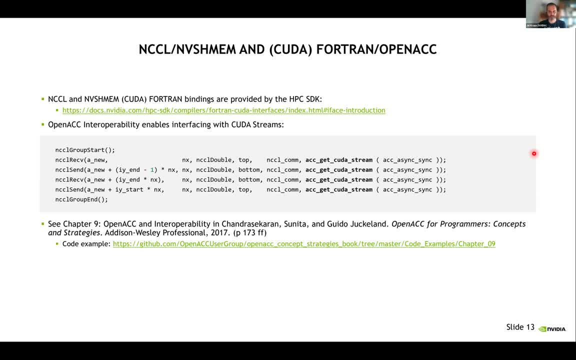 which are provided with the HPC SDK And if using the host APIs, and it's also interoperable with OpenACC, because you can, using the OpenACC interoperability API to get a CUDA stream for an OpenACC SMQ and you can use the OpenACC API to get a CUDA stream for an OpenACC SMQ and you 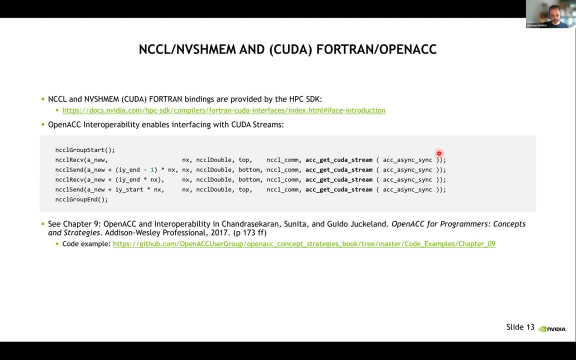 can use the OpenACC API to get a CUDA stream for an OpenACC SMQ or set a tie otherwise created CUDA stream to an OpenACC SMQ, and therefore you could also use nickel in parts of OpenACC applications the same way, almost the same way as you can. 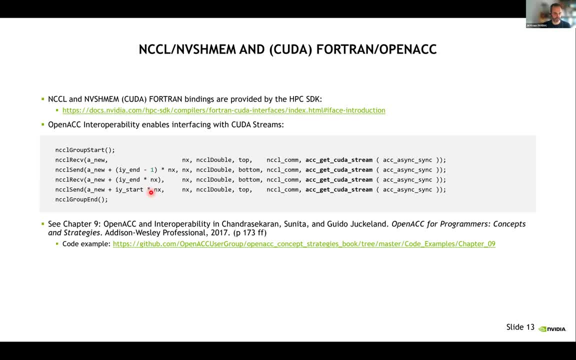 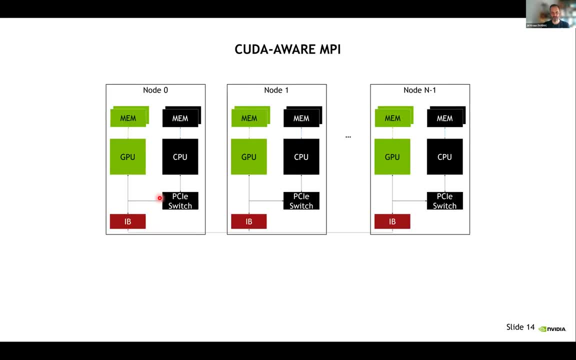 use the CUDA-aware MPI in the OpenACC application. Okay, now to the main part of my talk today. Okay, now to the main part of my talk today: CUDA-aware MPI. So I assume you're all here because you want or need to program a cluster with multiple nodes and possibly multiple. 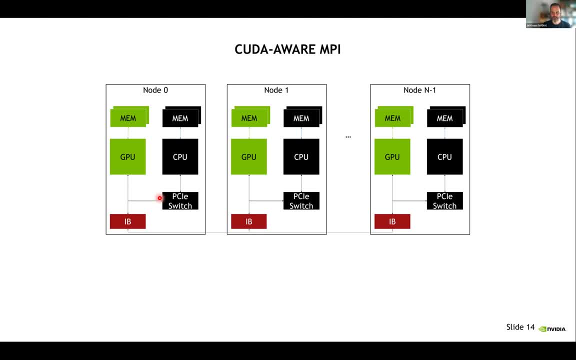 GPUs per node and need to use that to solve larger problems, for a given problem faster and so that all these GPUs work together on the same problem, And for that, at some point, this GPU needs to need to exchange. So let's get started. So, let's get started, So, let's get started. 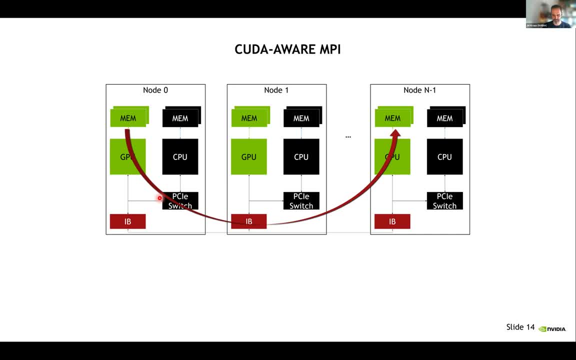 data, so that you're really coordinating on solving the problem and just not solving many similar problems totally independent of each other. And yeah, usually what I say here is: if you know GPU programming with CUDA, OpenACC, standard language parallelism and you know MPI, 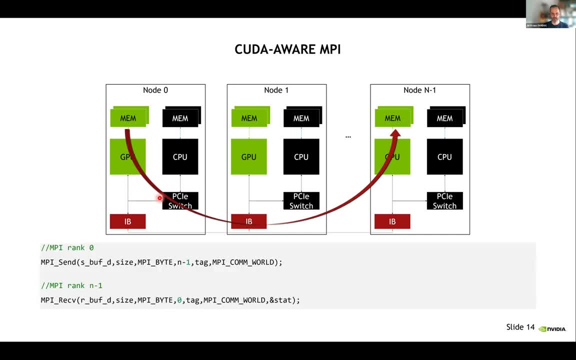 then I don't have to tell you much more. Just use a CUDA-aware MPI and things work as expected. So if you use a CUDA-aware MPI and pass a device pointer to the MPI, the MPI knows how to handle that, Move data in the most efficient way from the source buffer to the destination buffer. 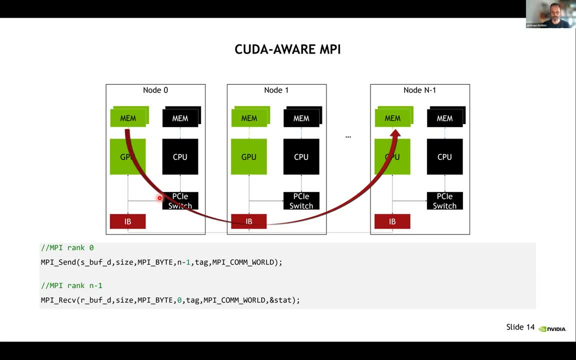 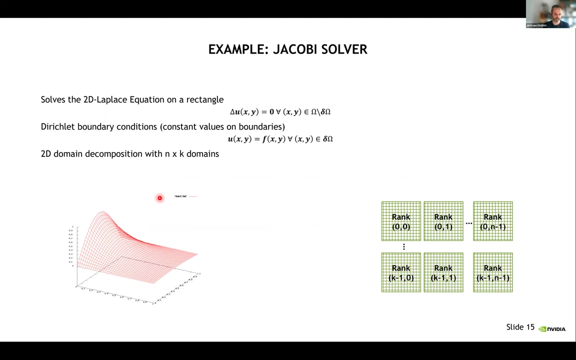 and things work as expected. Yeah, of course I'm not ending the talk here, because there are some things, tips and tricks to share and probably some internals to understand, to better reason about the performance behavior of the applications, To get everyone on the same page and set the stage to avoid losing some who might not be that. 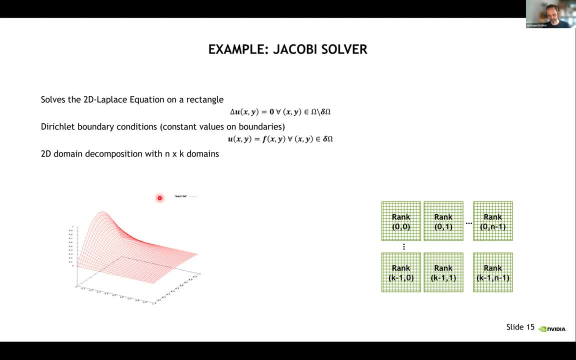 familiar with MPI or new to that. this is not an MPI tutorial, but I want to try to capture your anyway. Let me give a very simple introductory example that hopefully allows you to follow the rest of the talk. You're not that familiar with it. 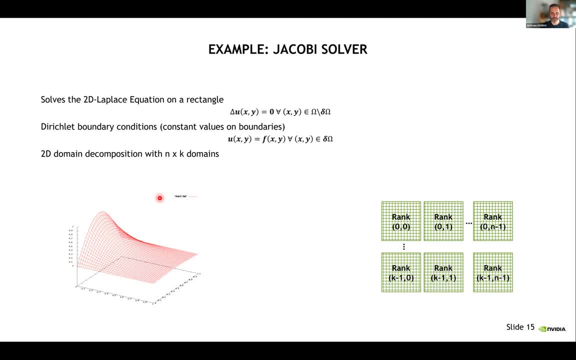 For that I'm using a Jacobi solver which, in case you're interested in the math but not necessary, It's also a 2D Laplace equation on a rectangle and I'm using directly boundary conditions, so constant values on the boundaries. 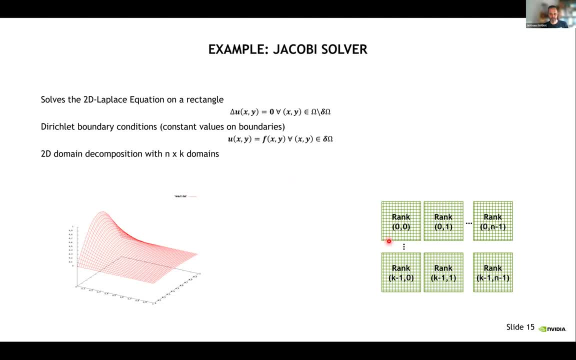 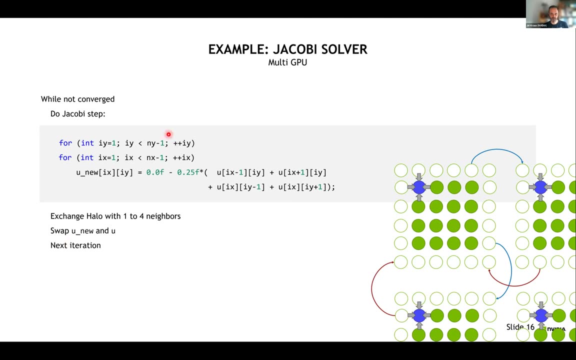 For the examples. here I'm using a 2D domain decomposition, so I'm cutting the domain in rectangles with n by k domains. So how does the implementation look? We have a while-not-converged loop and in every iteration of the loop, every ring. 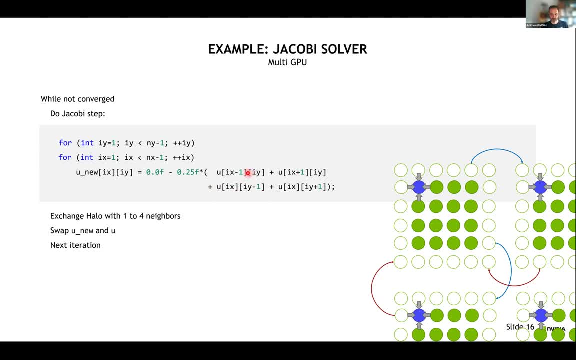 applies a so-called stencil to an array u and stores the result to u-u. So that means for the interior part of the domain, so leaving out a boundary, which is necessary because the operation effectively calculates the average of four neighboring points and stores it here. 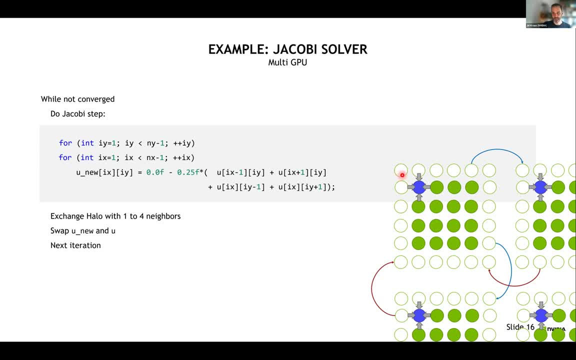 so we cannot do this. for the boundary values, We iterate over all interior points of our domain and then, because the domain is distributed across all GPUs and cut into these pieces, we need to make sure that the updates we have computed are visible to the other processes participating in our job execution, And for that we use so-called 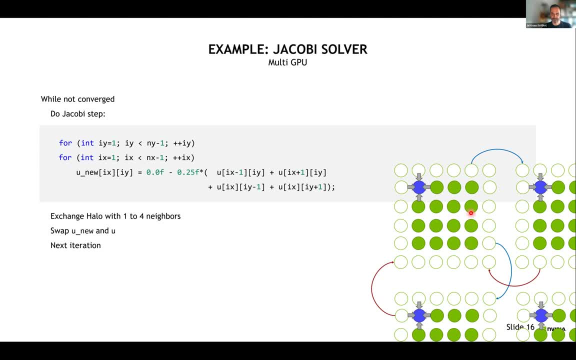 halos, which means the last interior row of each process and the last interior row, last interior column, first interior column, first interior column and last interior column, and so on. The first interior row is replicated to the right, bottom, top or left neighbor And then. 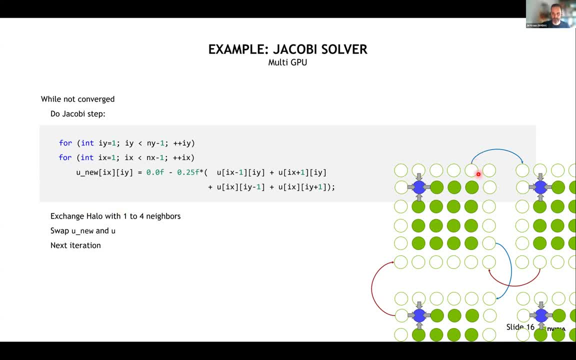 after each iteration we need to send this row to this replication, which is the boundary of the other one, so that it has up-to-date data in the next iteration and really threats us cooperating. Then we swap the roles of u-u and u-u and start the next iteration. 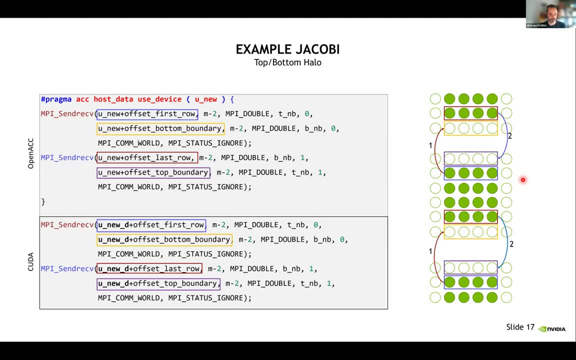 And with how that does that look like with OpenACC and CUDA? I'm using here for brevity on the slide: MPI: send- receive. In most applications you would probably use non-blocking MPI like I receive. I send- wait all patterns, but this is just to keep the 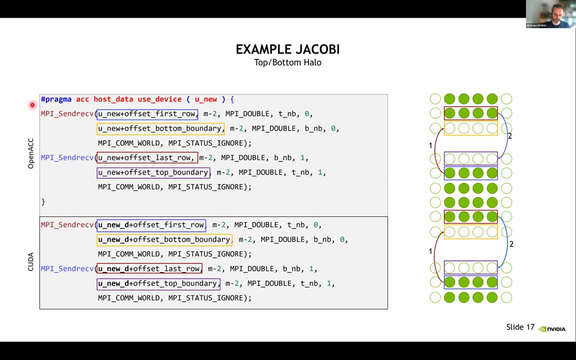 slide a bit more brief. So in case of OpenACC, because we compute on the GPU, we need to use a pragma-acc-hostdata-use-device to pass the right data to the MPI library. That is necessary because from the OpenACC compiler's perspective, the MPI call is a CPU call and usually 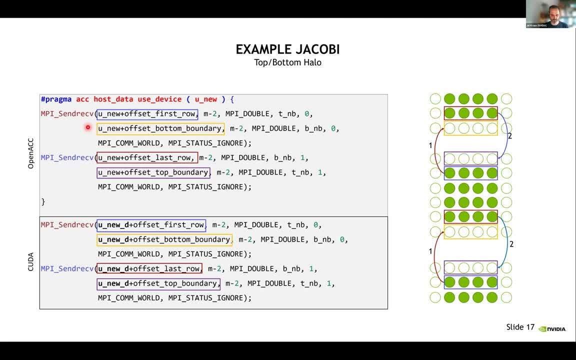 an OpenACC compiler derives from context, It should use the host representation, so CPU representation of the symbol, like u-u, or the device representation. Since we have modified with the previous kernel the data on the GPU, we want to use, of course, the device representation, and that is what we tell the compiler by using pragma-acc-hostdata-use-device. 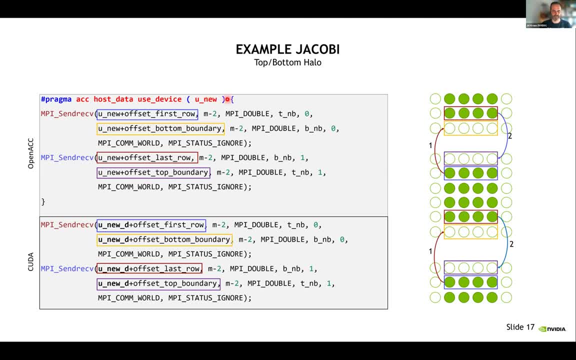 that in the following structured block the device representation should be used even if we are calling into CPU. And then we have two send receives for top and bottom halo exchange. The first one sends to our, our top neighbor and at the same time receives from our bottom neighbor, the first row modified. 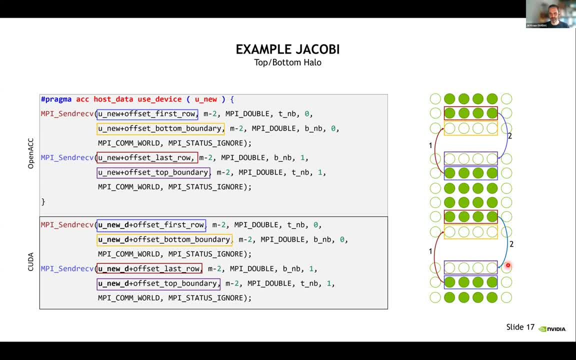 and to the bottom boundary. The second call sends to our bottom neighbor and at the same time receives from our top neighbor, the last row, representing the top boundary. In CUDA this looks exactly the same, except that there we have a direct pointer to the data we have. 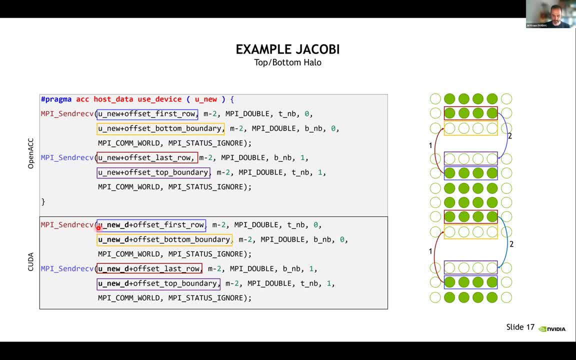 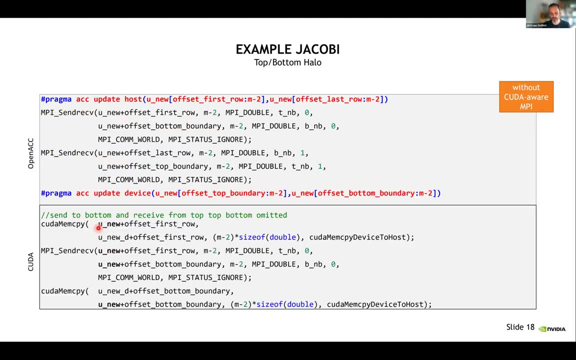 modified on the GPU. In contrast to that, if you would not use a CUDA with MPI- so the MPI is not able to handle device data directly- we would first need to copy the data from the GPU to the CPU, then exit, which would be the CPU. 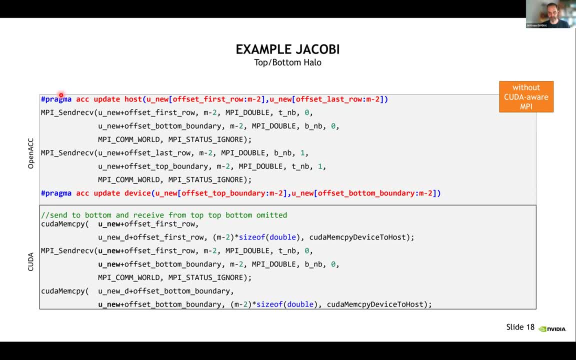 This would be done in OpenACC with a pragma ACC update host. Do our communication and after the communication is finished- because then the communication data is in CPU memory- copy the data back from the CPU to the GPU before the communication computation can continue there. 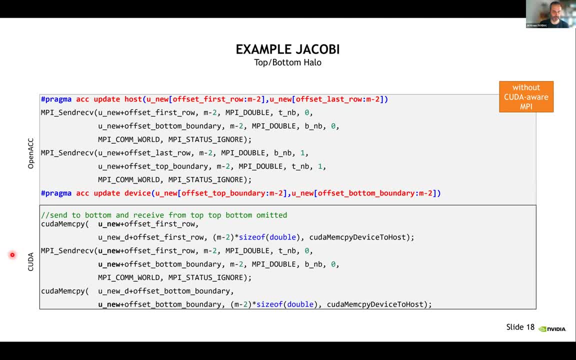 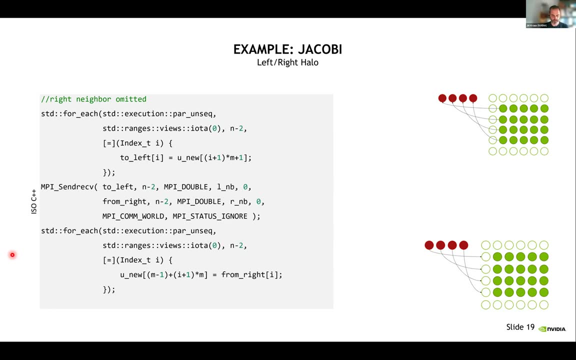 Conceptually with CUDA we need to do the same, but it just looks. we don't use a pragma but an API call. Okay, CUDA with MPI also works with standard language parallelism, for example BOTRAN do-concurrent or C++ did-par. 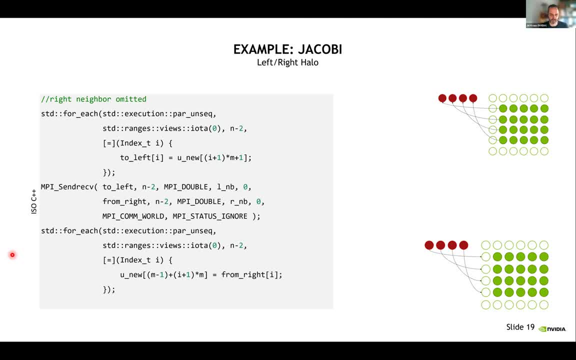 And these implementations available with the HPC SDK rely on unified memory, so there is no need for any data clauses or copying, because every pointer you use is unified memory and therefore usable on every processor in the system, And it just migrates where it's most used. 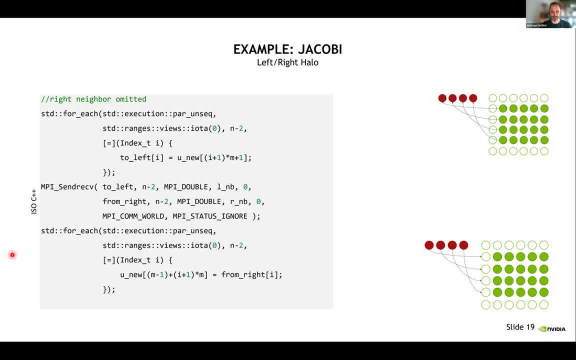 And to showcase that I use the left-right hero exchange, where we usually, because sending individual elements is very inefficient, so we usually need to pack to a larger communication buffer, which we, in case of ISO C++, could do with this for each parallel loop for packing. 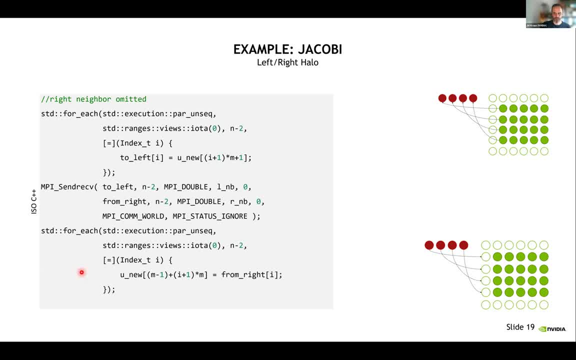 Then we do our communication And then we need to do unpacking after communication is finished. Yeah, As said, because we're using unified memory, there's no data clauses, no copying required. The CUDA-aware: yeah, all current version of CUDA-aware MPI implementations are aware. 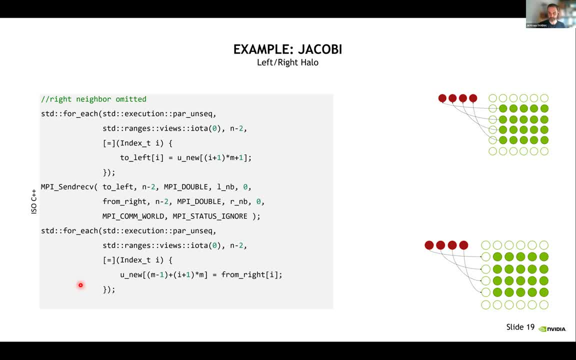 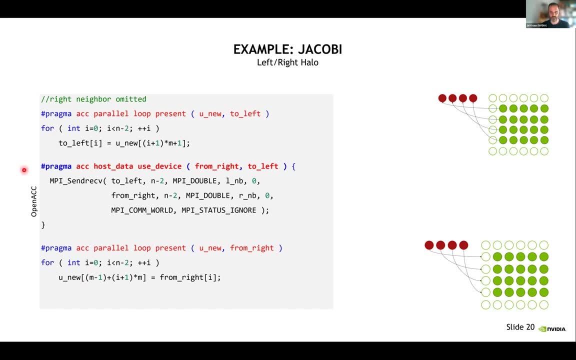 of unified memory and know how to handle it With OpenACC. conceptually, we need to do the same, Just that. of course, again, we need to use the host data use device directive to pass the write Write data into And we want to do the gathering and scattering of our non-contiguous data in GPU memory. 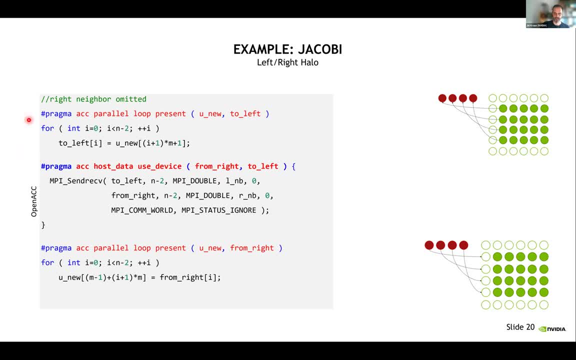 So they do that with OpenACC-generated GPU kernels. Same, of course, CUDA. Just there we use kernels instead of relying on the compiler to generate them. Okay, So there are two more things, One which I want to mention, which are a bit different to just using MPI. 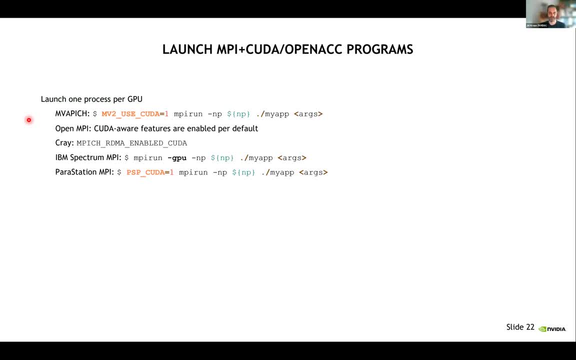 One is launching MPI as CUDA OpenACC programs, And I'm pointing that out because some CUDA-aware MPI implementations require you to enable CUDA-aware features at runtime. Of course, if you're built in from source, they need to be configured with CUDA features. 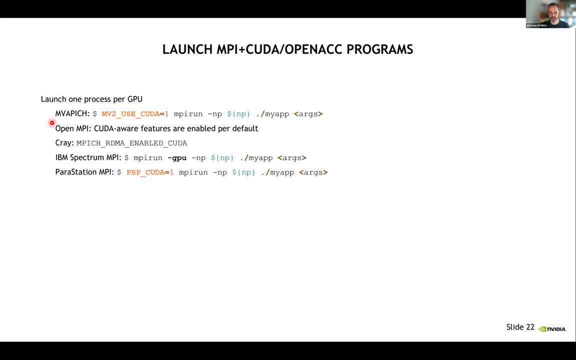 But if there are, you still need to. So OpenMPI As a CUDA-aware feature is enabled by default. MVA pitch needs to set this environment variable gray also an environment variable. IBM Spectrum MPI has a switch to the launcher. 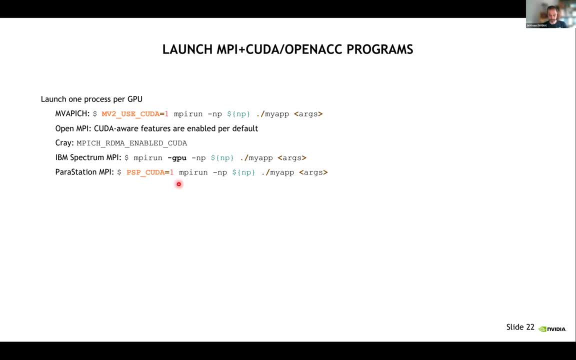 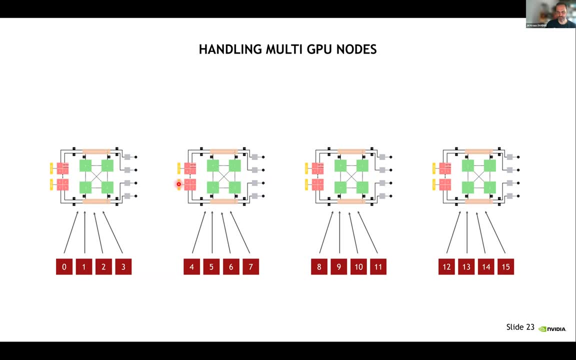 And PyroStation MPI, also MPI variable. The other aspect is handling multi-GPU nodes. So, for example, consider we have four nodes with four GPU each and launch one MPI variable. Okay, All right. So if we have four nodes with four GPU each and launch one MPI variable, we would end. 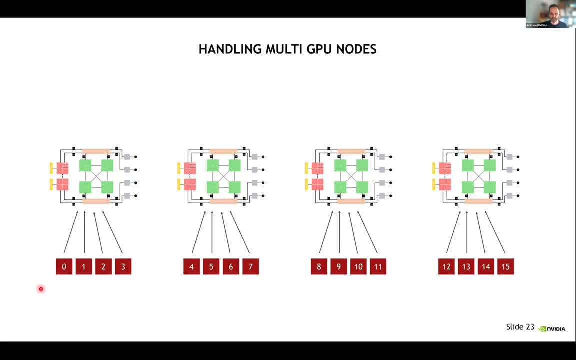 up with 16 processes, zero to 15. And let's assume our job scheduler distributes them consecutively on each node. So first node has zero to three, second node four to seven, and so on. Now, if you don't do anything with handling GPU affinity, so no CUDA set device, no ACC. 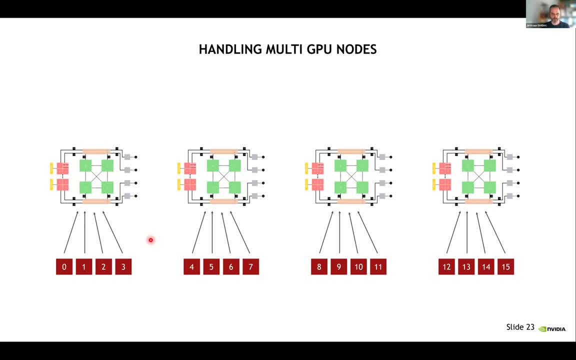 directive to select a device. they would all just pick device zero. So on every node you would oversubscribe GPU zero and leave GPU one, two and three idle. The question now is how to select a device, especially on the second node, because there's 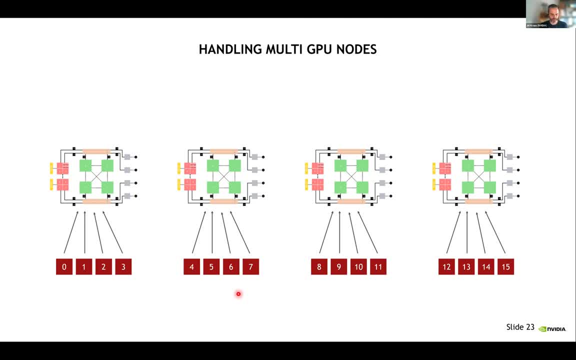 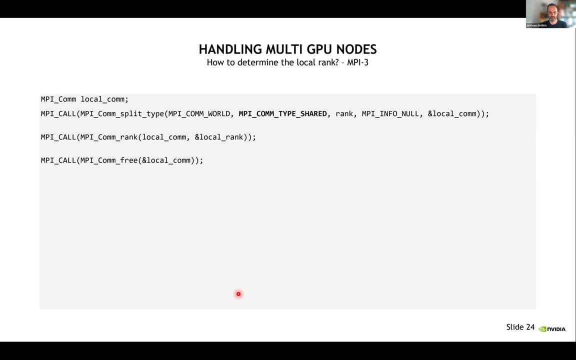 no device. four, and how to come up with the right device ID to choose. So what I usually propose is determine a local rank, which can be done by using MPI. com split type using the type com type shared. Com type shared gives you a communicator where all MPI ranks in. that communicator can. 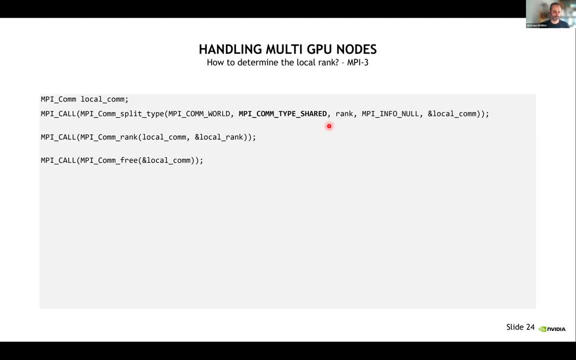 communicate via shared memory And that effectively means that it's all MPI ranks running on the same node. So we create such a new local communicator query, that local communicator for a rank, and then we no longer need that, so we can immediately free it. 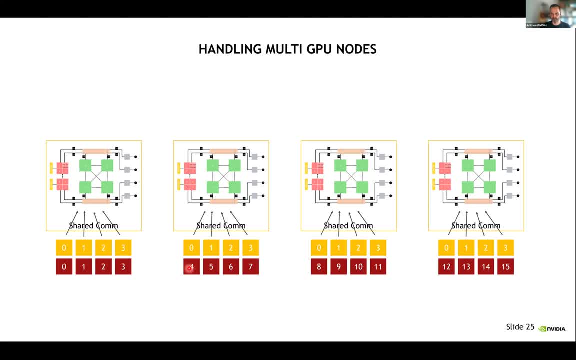 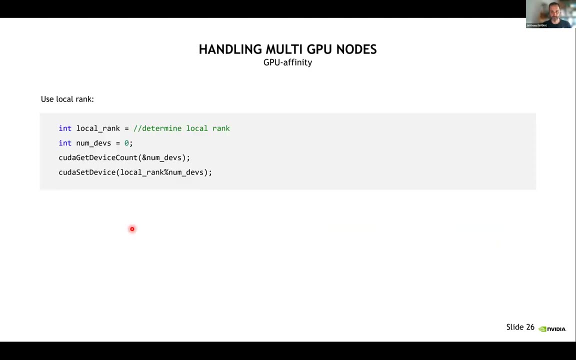 So visually that means we have still our MPI com world with ranks zero to 15, but we now have split it up into four per node communications with rank zero to three And we can use these local ranks to call CUDA set device to select the right rank or 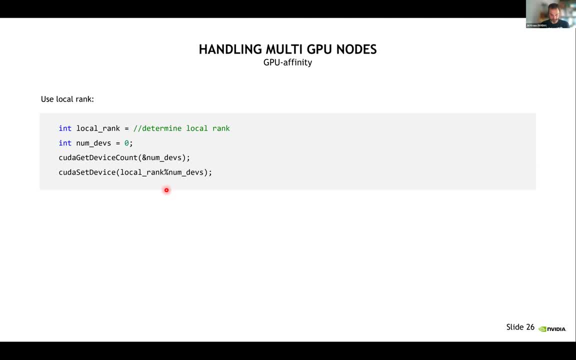 the equivalent OpenACC directory. So what I have also added here is querying the number of visible devices and do a model operation. That's done for two reasons. First of all, as I introduced later, in some cases it might be worthwhile to launch multiple 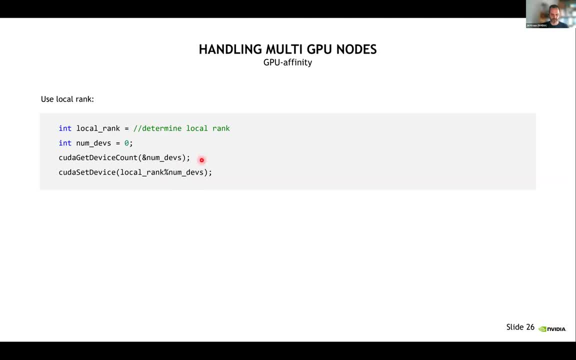 MPI ranks for GPU. So that would be supported then by that. So because you might have more MPI ranks per node than you have GPUs. And secondly, there are some MPI launches or you might use a launcher script to handle the GPU affinity externally to the program so that nothing like CUDA set device is needed. 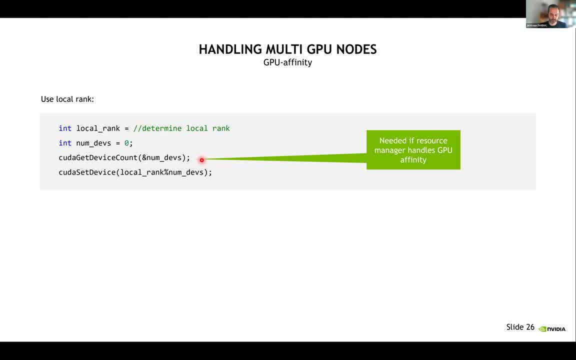 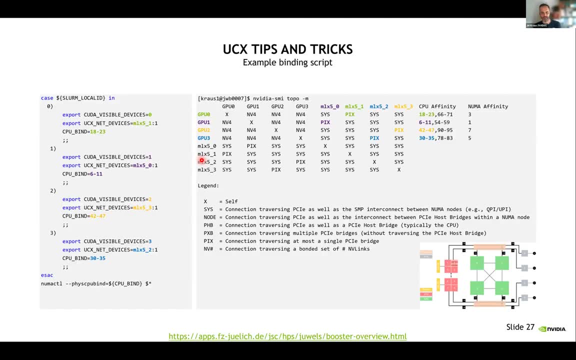 here Related to that external resource managing, external GPU affinity handling. conceptually it does something like I've shown in this script on the live side. So I've shown here the node topology of the node of the Jules Booster, a system at JFC. 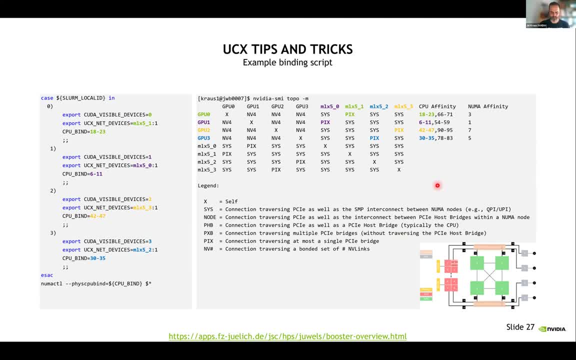 in western part of Germany, where I'm from, With 936 GPUs Nodes and four A100 each, And how to map this topology to a good job execution with using a launcher script that just sets environment variables so that your application don't need to handle GPU affinity. 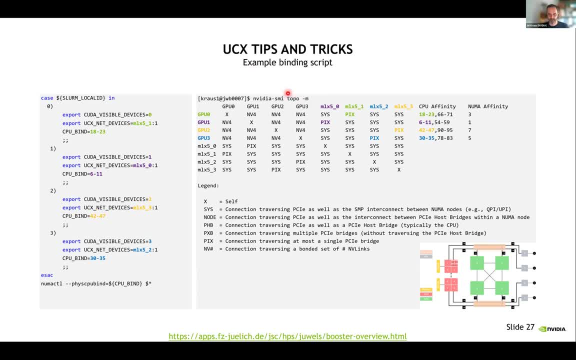 To determine the right values. what I want to point out here is the tool nvdsmi-topo-m. nvdsmi is the tool to manage GPU affinity. Right Yeah, So you can see here the GPUs in the system, and the topo suboption provides your topology. 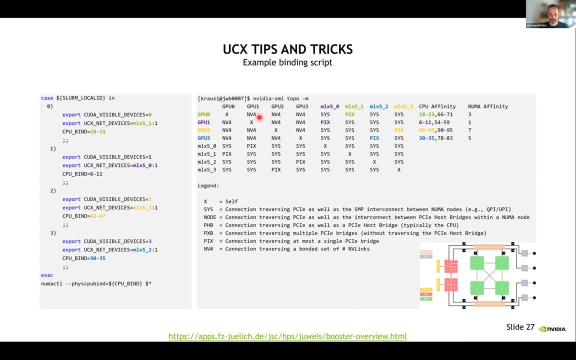 view and gives you this connection matrix saying you how GPUs are connected with each other, if they're connected to any link, and how they are connected to the network adapters in the system and which are the local CPU affinity. So, based on the information provided here, using environment variables set by the launcher, 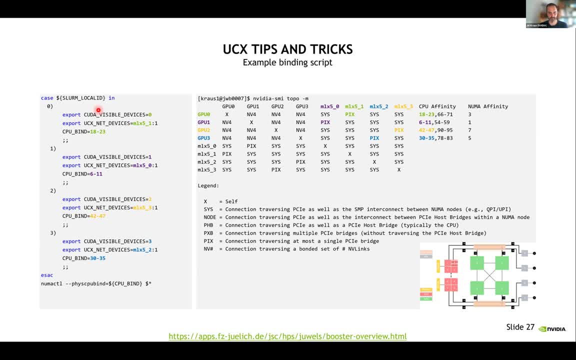 on the system. In this case it's Slurm, And I use Slurm local ID, which corresponds to the local rank returned by the MPI calls I have shown before. If I'm rank zero, I want to use GPU zero because GPU zero has a fast single PCI express. 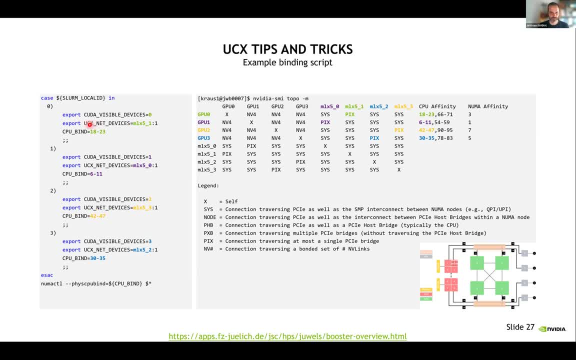 switch connection to the Mellanox adapter one. I set UCX net devices to Mellanox adapter one And the closed CPU cores are 18 to 33. So I set CPU by two. I do the same for rank one and GPU one, rank two and GPU two, and so on. 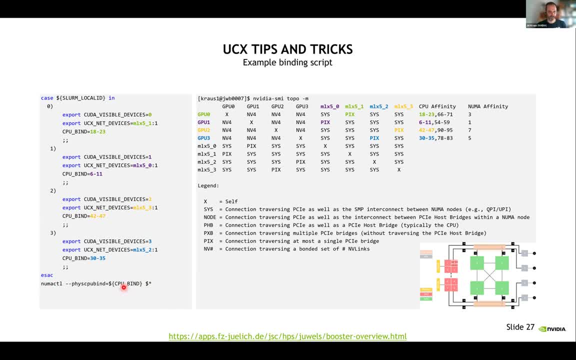 And then I just use NUMA CTL to bind to the correct CPUs- the environment variable takes care of the network adapter and the GPU- and then launch my application. So that could be part of a script where your job execution is just prefixed. First of all, I wanted to point you out as a trick to optimize performance of your application. 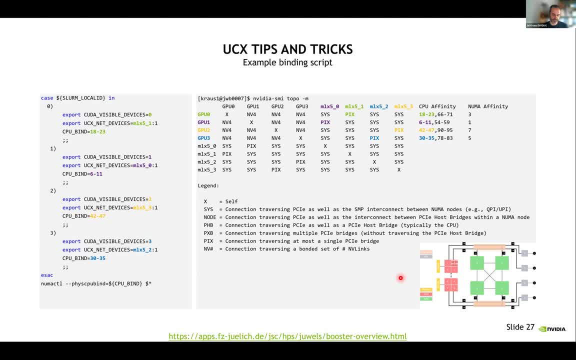 But also because actually on some systems the job scheduler automatically does this. This is, for example, the case for the Jules Booster system. There, if you launch a job with SRUN, it will automatically set put a visible devices. 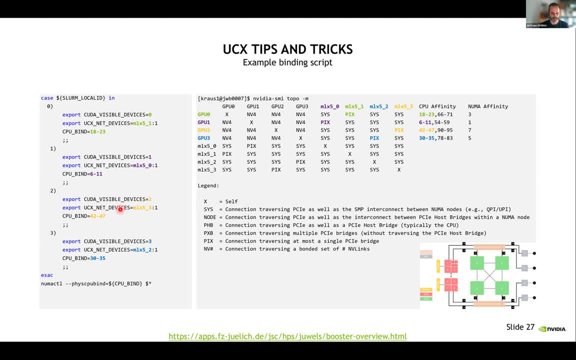 and bind your processes so that you're effectively using the system. Okay, That is, I would say, really just to get started, And then all you need to know to run, use MPI to program multiple GPUs and multi-GPU system. The remainder of the talk will explain you some fundamentals: how things work internally. 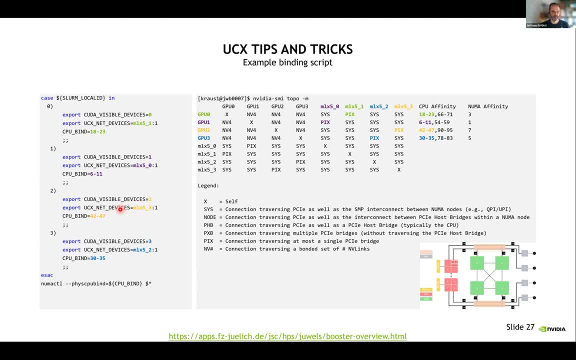 and why things work and how to use tools to allow you to analyze and optimize the performance of MPI plus CUDA, OpenACC standard language. Thank you, Thank you, Thank you. It is really useful for you know real-time language, pounds and codes and, yes, reason. 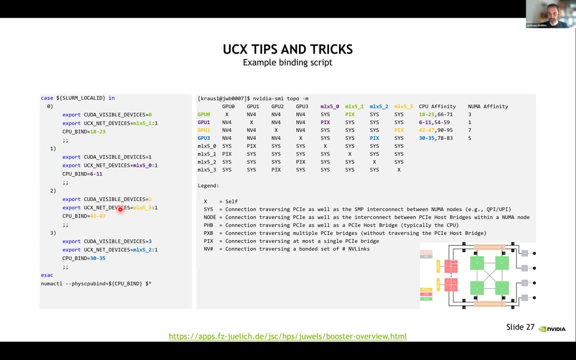 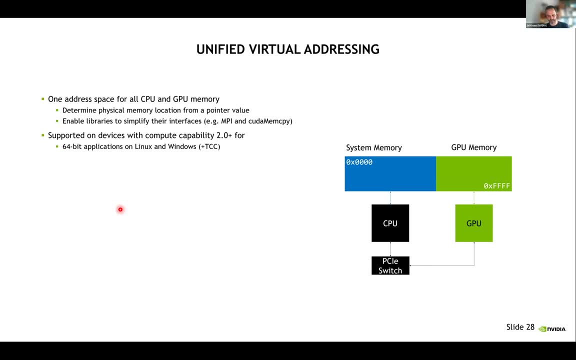 about performance behavior. First, why does it all work? How does the CUDA and WNPI know that the pointer is a GPU pointer? It needs to be differently handled, differently to a CPU pointer. The enabling feature for that is Unified Virtual Address, Not to confuse with unified memory, which is also sometimes abbreviated as UVM Unified. 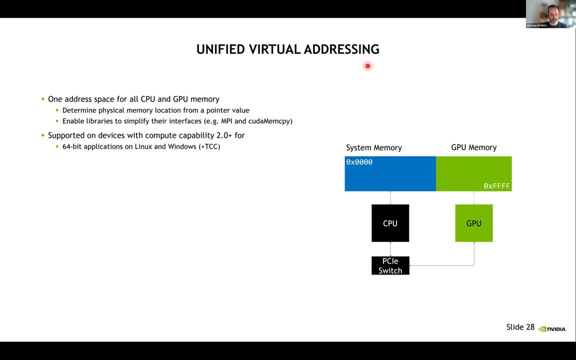 Virtual Memory. Not too confusing really. Yeah Yeah, Because the plain words are better-aaa-ish. There's stuff for good. Please dig into the shebang. unified memory or managed memory. it's unified virtual addressing, So the memory that's. 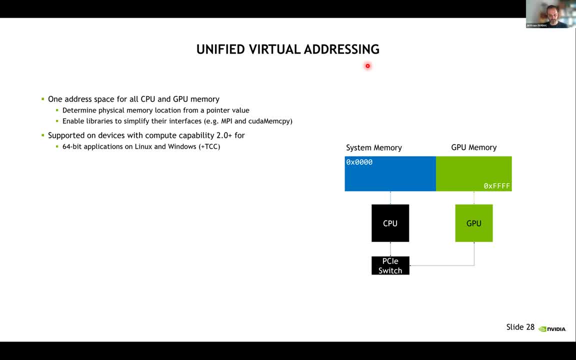 for example, allocated with CUDA analog, is pinned memory on the GPU. it cannot move, so the virtual to physical address mapping stays the same, but it's still part of a unified virtual address space. So what does it mean If I have unified virtual addressing all the memory? 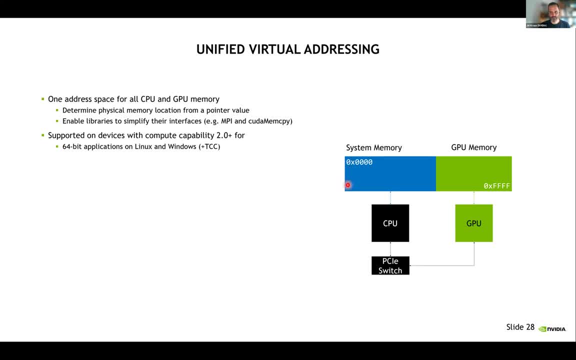 allocations of the processes are put into a continuous address space and a certain part of the address space is reserved for CPU allocations. a certain part is reserved for every GPU, and that allows that you can determine the physical location of a pointer by its pointer. 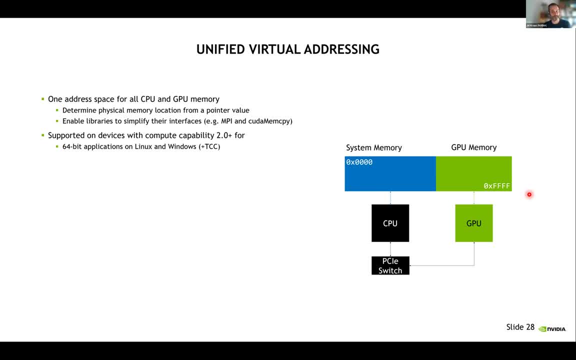 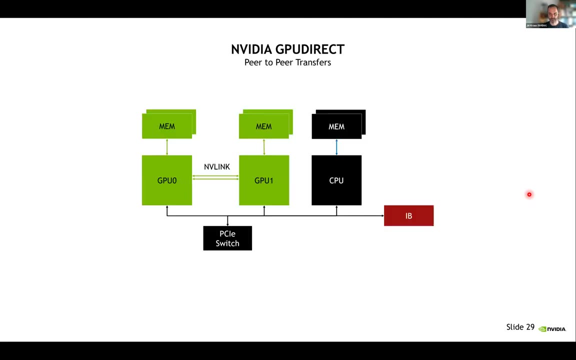 value and allow a library, like, for example, a CUDA or MPI, to query a pointer where it points to and then take the right decision to move the data. Other relevant technologies are GPU direct, because they allow to move data faster between GPUs. I want to touch on the two important ones. peer-to-peer, which allows to move data directly. 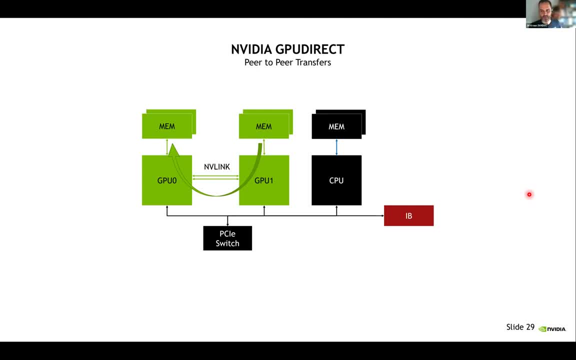 from the memory of one GPU to the memory of another GPU in the same node, over and delay, without any intermediate staging in CPU memory or even CPU involvement. And then there is GPU direct RDMA, which allows a non-GPU device to directly read and write. 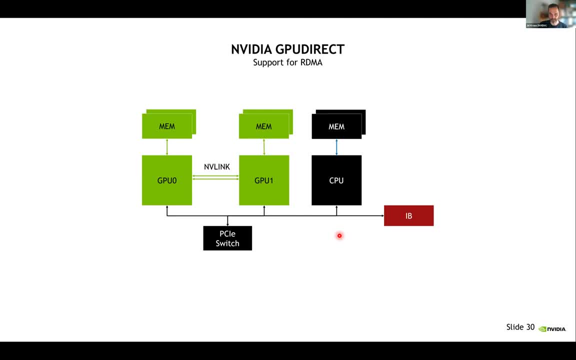 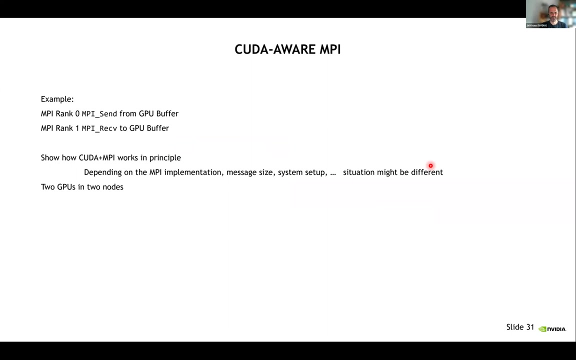 GPU memory over PCI Express. This can be leveraged by network adapters to directly read or write GPU memory and send it over the network without intermediate staging in CPU memory or CPU involvement with the transfer. To highlight the performance effect of this, I've chosen a very simple example. 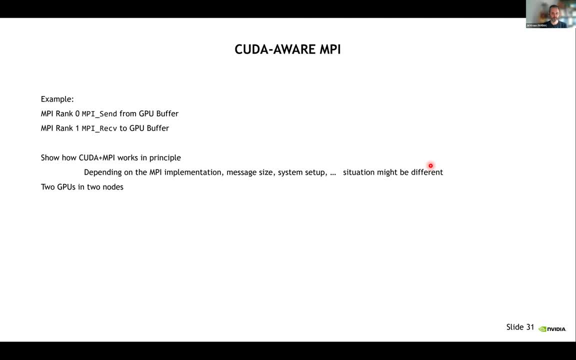 where MPI rank 0 does an MPI send from a GPU buffer and MPI rank 1 does an MPI receive to a GPU buffer and they're matching from a communication. This is to show how CUDA plus MPI works in principle. depending on your memory, This is to show how CUDA plus MPI works in principle. 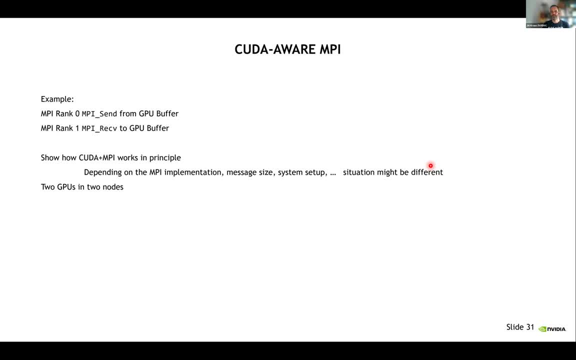 depending on your memory. This is to show how CUDA plus MPI works in principle. depending on your memory, When you're running your MPI implementation, your system set up your message size. the situation might be different, But still, I think it will help you to understand. 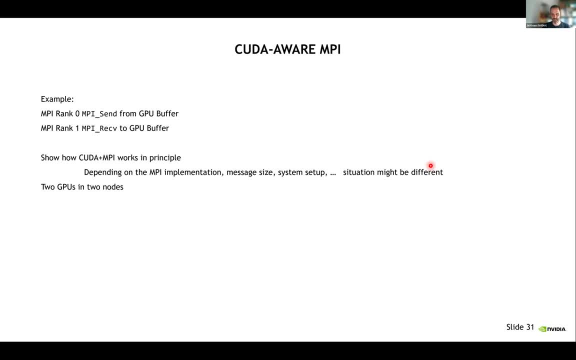 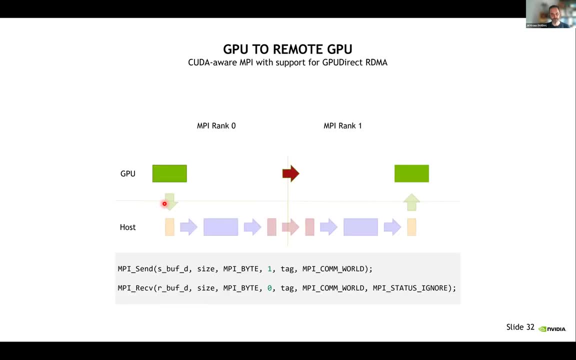 the performance behavior of MPI communication between GPUs better, And we are looking at two GPUs in two modes. So first we look at the case that we have a CUDA with MPI with support for GPU direct RDMA. In this case we call MPI- send on the source buffer in GPU memory and we call the source buffer in GPU memory and we call the source buffer in GPU memory. 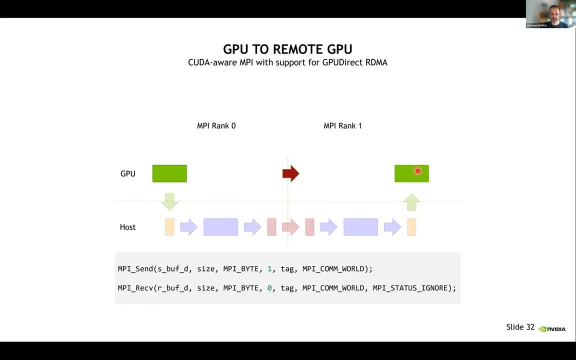 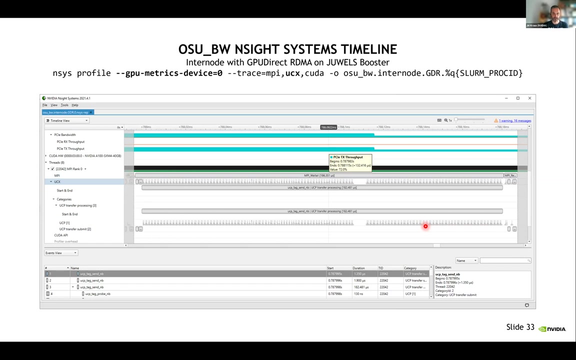 GPU, memory and MPI received on the destination buffer. also, a GPU And MPI takes care to directly move data over the network from source to destination buffer without touching any intermediate buffer on the CPU. If we analyze that with inside systems and create an application trace and look into that. 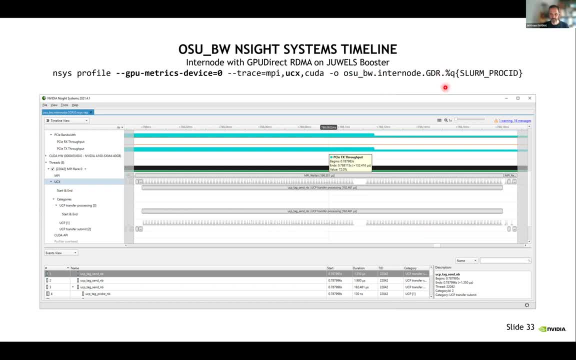 I've done this for the OZU bandwidth, So I've done a benchmark and also sampled GPU metrics to see activity on the PCI Express bus. What we see is first that we don't see any GPU activity because all the transfer is carried out. 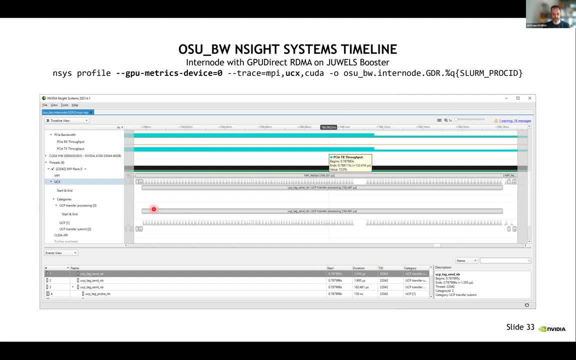 by the network adapter. So these are the direct reads from the network adapter. So we don't have any CUDA API faults, We don't have any GPU activity, But we see PCI Express activity because these are the network adapters from GPU memory to move the data. 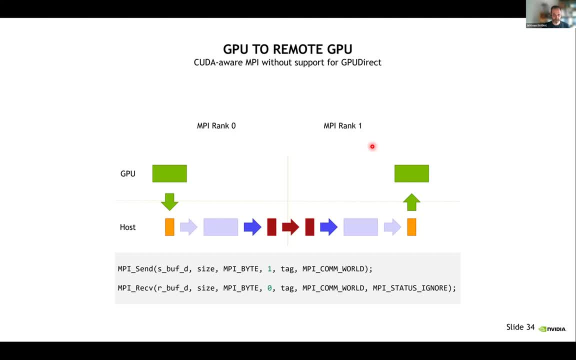 In contrast to that, if we have a CUDA-aware MPI without support for GPU direct, we call MPI the same way, because the MPI knows how to handle GPU data. However, because it can't move data directly, it needs to stage between intermediate buffer and CPU. 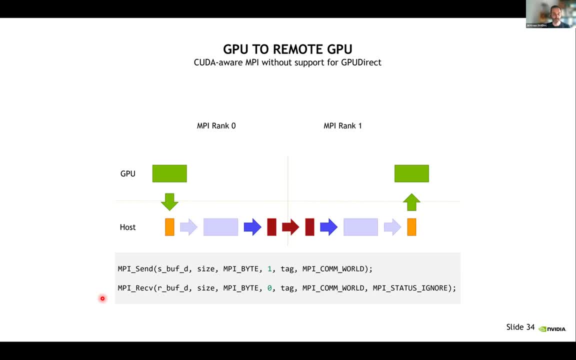 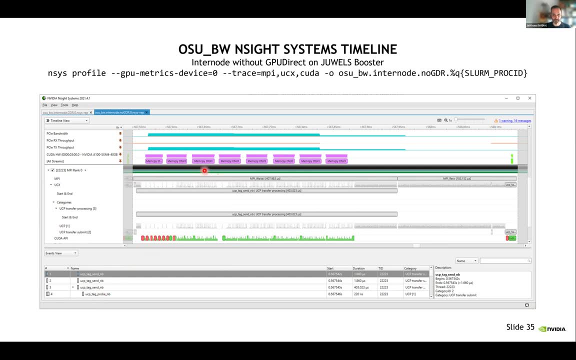 memory to move data. This can also be seen in the same profile. Now we have a pipeline executed. We have multiple chunks of device-to-host transfers, because before sending data on rank 0, data is copied from device to host and then transferred over the network in chunks. 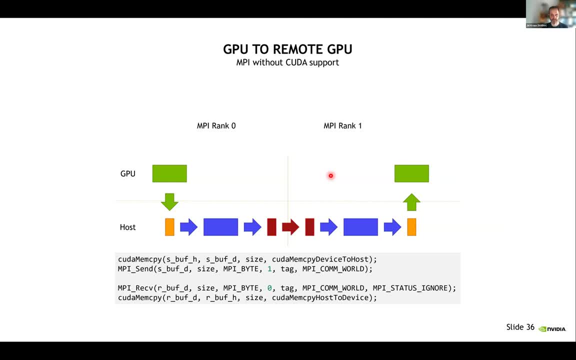 Last in a steep contrast. also, if we have an MPI without CUDA support, so need to copy manually in the application side from the GPU to the CPU. OK, So we can see that the data is being sent to the CPU before starting our communication and copying. 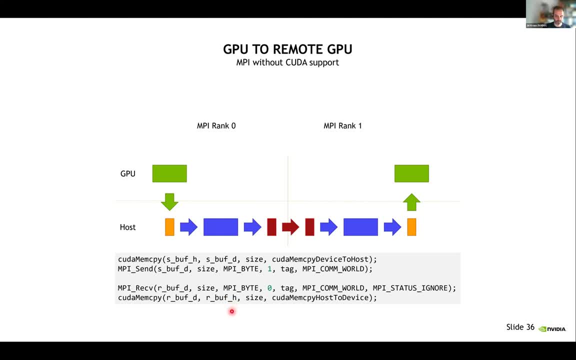 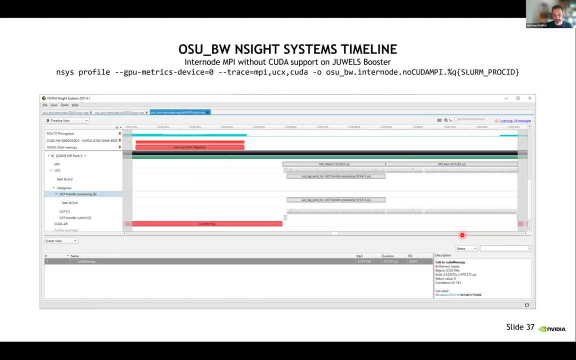 from the CPU to the GPU after we have received data. Of course, there are more intermediate copies involved, But also the pipeline stalls after moving data to the CPU and after moving data with MPI. So we have more steps and pipeline stalls, And this is the same for internal transfer. 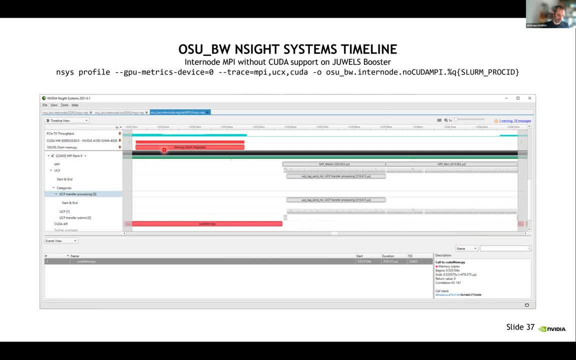 So we have a large device-to-host transfer and then the network transfers. So we now have not a relatively efficient pipeline of device-to-host mem copies and network transfers. We have one large device-to-host transfer and then the network transfers. This is just the source rank. 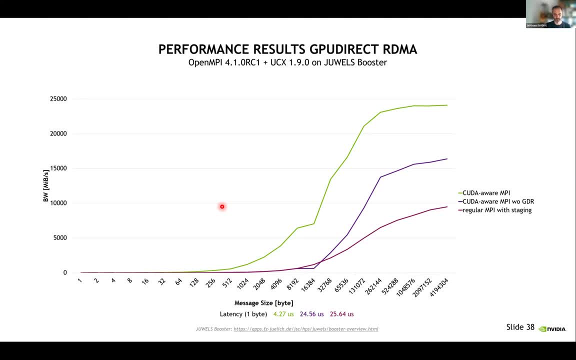 This can be also seen when looking at performance. So when I look at the performance of internode transfers with a regular MPI, we see we are limited by 10 gigabytes with a CUDA WMPI without using GP-Direct RDMA. 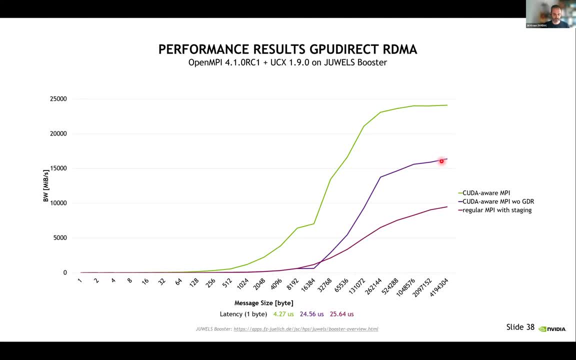 we get almost twice the performance because we can execute in the pipeline. But we are still limited in performance by executing the staging pipeline And we can really saturate the available network bandwidth if we can use GP-Direct RDMA. This has also a significant effect on latency. 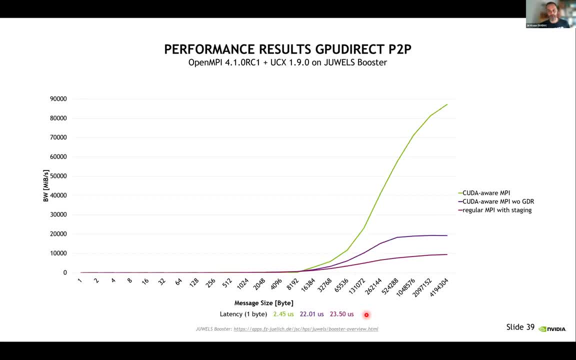 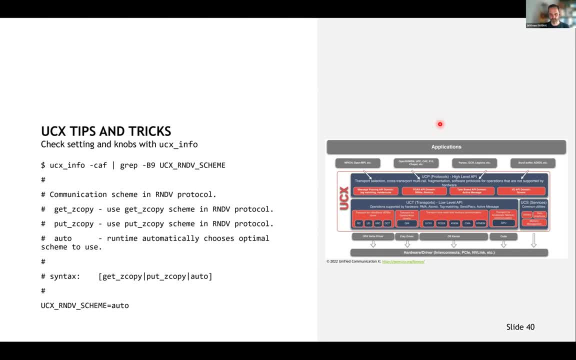 Closing this internodes one with a short collection of UCX tips and tricks. And why am I mentioning this? Because you might wonder: what is UCX? That's a communication framework not intended to be used by application developers directly, like you. 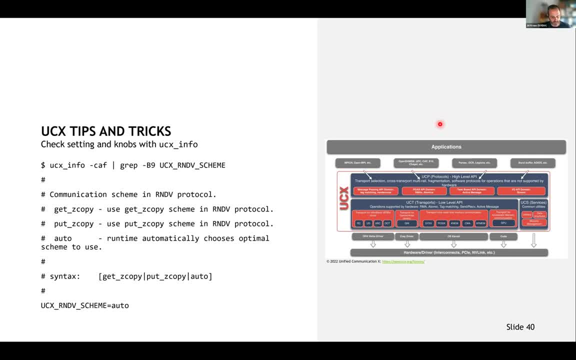 but to be used by communication libraries like MPI. So many MPI implementations built on UCX to implement the actual data movements. Therefore, actually, the data movement I've shown you is, while you call MPI, it's not executed by MPI, The buffers are just passed through to UCX. 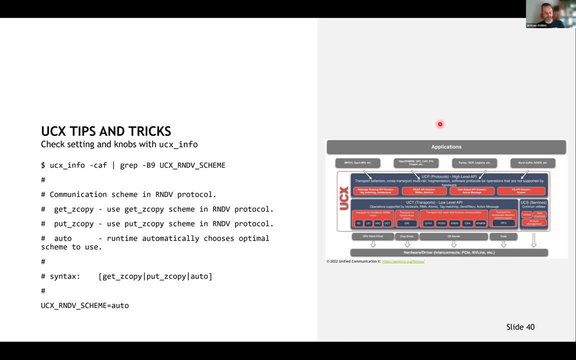 And then UCX moves the data. So that's important to know, because when you want to kill performance, you don't need to look for MPI parameters, You need to actually look for UCX parameters And to find you on things like protocols, thresholds. 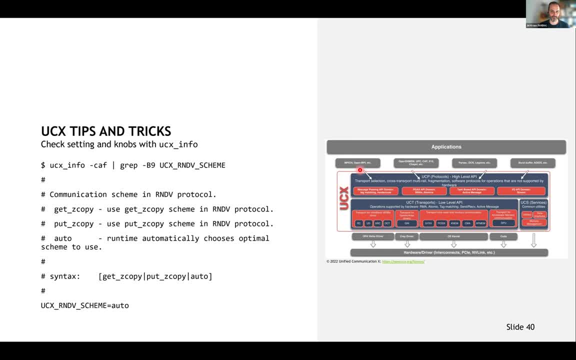 to switch between protocols and so on. UCX interprets a lot of environment-level labels. So the first tip I want to show you is that this points you to the fact that UCX is used and, in many cases, that UCX exposes environment. 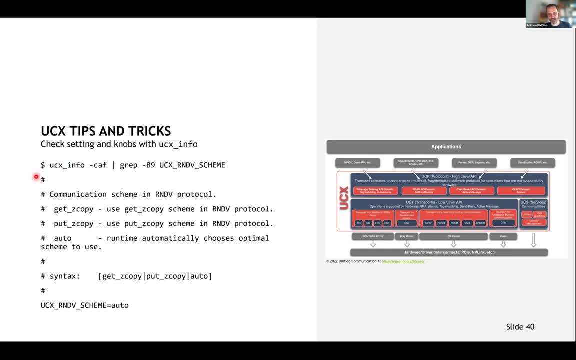 variables to influence its behavior. And the second one is that you can use the UCX underscore info program that comes with every UCX installation to query which environment variables are interpreted and what are their default values. For example, the rendezvous scheme, when you look at the output, has a lot of variables. 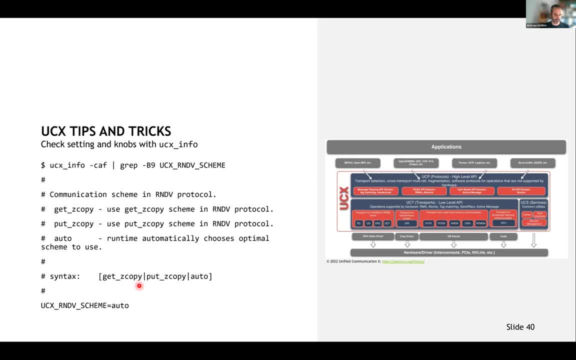 And you can see that the environment variables are interpreted and what are their default variables. For example, the rendezvous scheme, when you look at the output, has a lot of variables. It has three different roles: auto, a GET-based protocol. 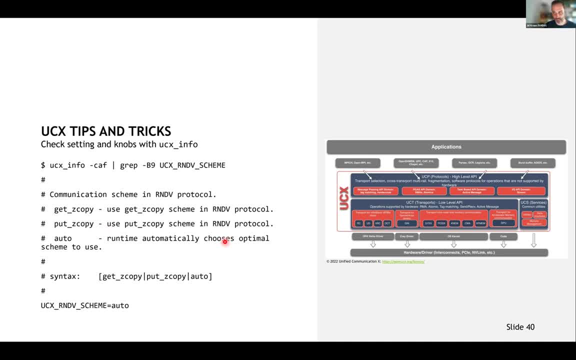 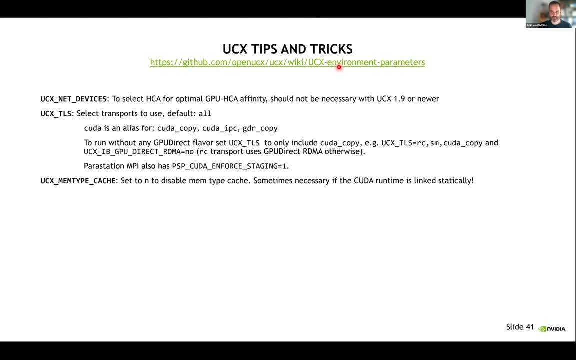 a PUT-based protocol and here is also some explanation. You can also find some information about this environment parameters on the UCX wiki, on GitHub. And three I want to point out. One is you have already seen UCX net devices, which 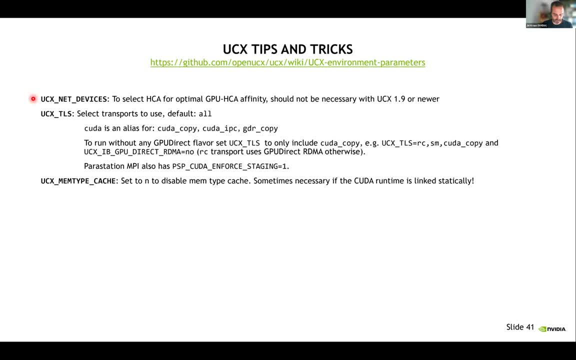 is a list of network devices that the processes with that environment-level set are allowed to use, which is sometimes helpful to tune performance. There's always work to improve the heuristic to select the right device, So depending on the UCX version you're using and the system. 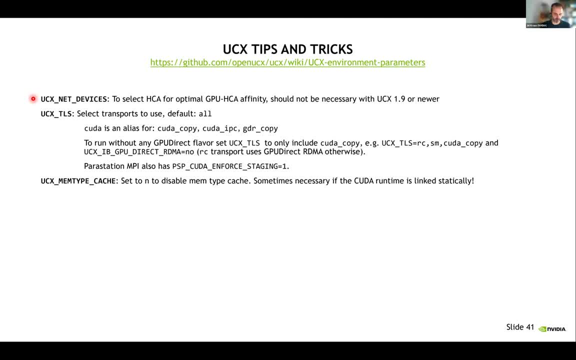 you're on. that might help performance or might be effectively no-op, because the UCX internal heuristic already does the optimal thing. Then for debugging there's UCX memtype cache. So querying where a pointer points to comes with some overhead. And to amortize that overhead UCX maintains a cache. 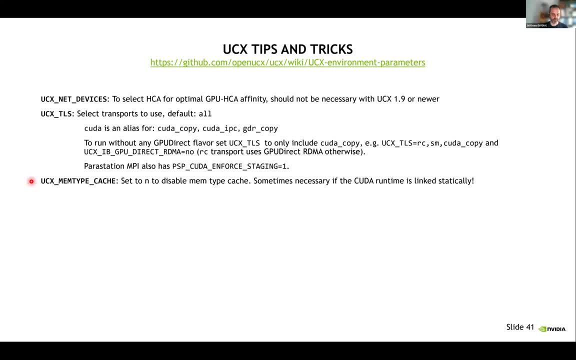 where a pointer it has already seen points to it. It's a CPU memory, It's GPU memory And to keep that cache up to date it needs to know when buffers are deallocated, And for that it does some tricks to intercept CUDA-free calls and so on. 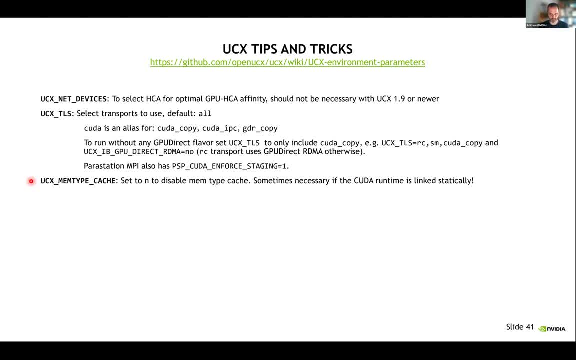 But in some cases it's not. In some cases these tricks don't work out And then the cache can become stale And that can, for example, result in segmentation falls or errors like that or, in worst case, corrupted data. 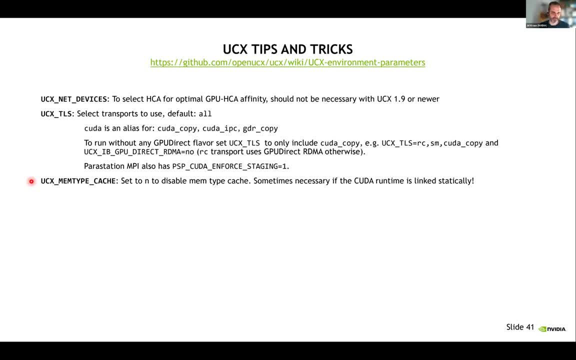 And to rule out issues with the cache, it's sometimes helpful to disable the memtype cache by setting UCX memtype cache to null. Another thing to debug and do a performance experiment is UCX TLS, which is the list of transports UCX is allowed to use. 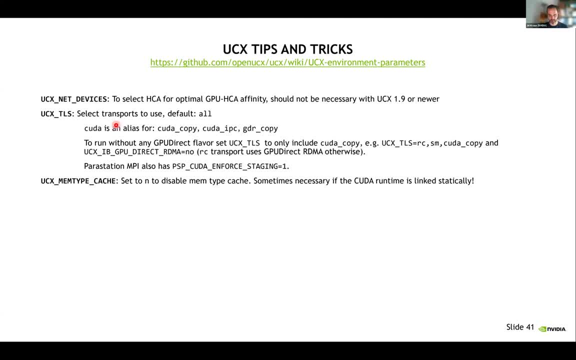 The ones I want to point out are the ones related to moving data in and out of the GPU, And these are CUDA copy, CUDA, IPC, GDR copy, which are summarized under the CUDA TLS. So CUDA copy is the staging pipeline I've shown. 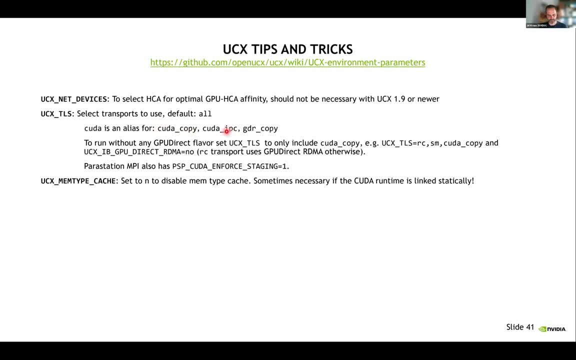 CUDA IPC is using CUDA IPC CUDA Interface and CUDA IPC. CUDA IPC is using CUDA IPC CUDA Interface and CUDA IPC. CUDA IPC is using CUDA IPC CUDA Interface and CUDA IPC. CUDA IPC. CUDA IPC is a for load latency communications. 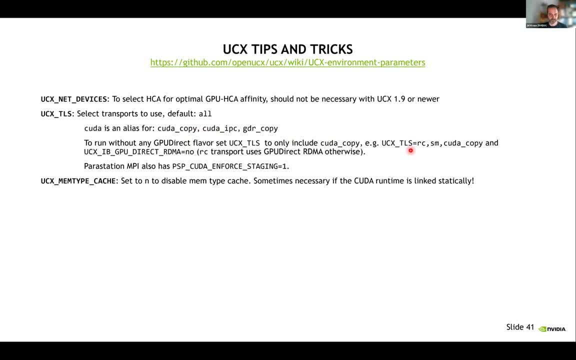 In addition to that, the typical for internode, for example, on an Innowbring, you usually use the TLS, RCDC or DC And then you can play around with, sometimes to the back, performance issue issues or understand performance better or correctness issues by disabling certain 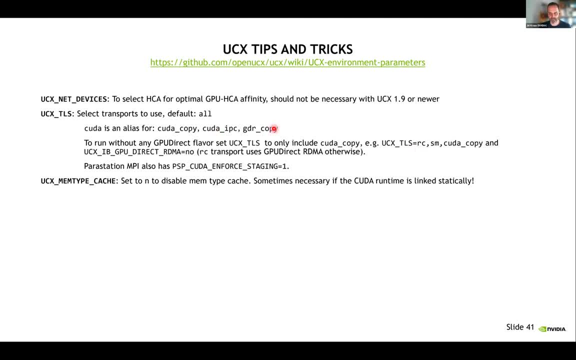 transports. For example, you could exclude CUDA IPC GDR copy from your list of UCX TLS and also set UCX IB GPRECT RDMA to no, to disable all variants of GPRECT RDMA and see how it impacts your performance or maybe solve a problem because something is miscomplicated on the system you're. 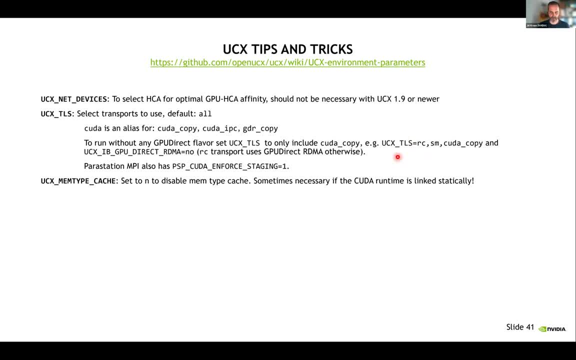 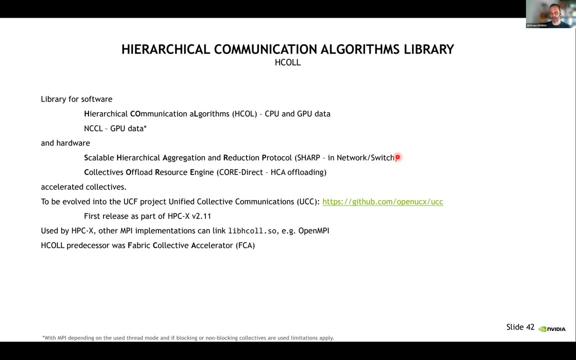 using. This is a combination I've used to run the experiments with GPRECT RDMA enabled or disabled. I've shown before. Okay, let me switch gears and go to collectives. Brief introduction of the Hierarchical Communications Algorithms Library, which is a library already mentioned in the 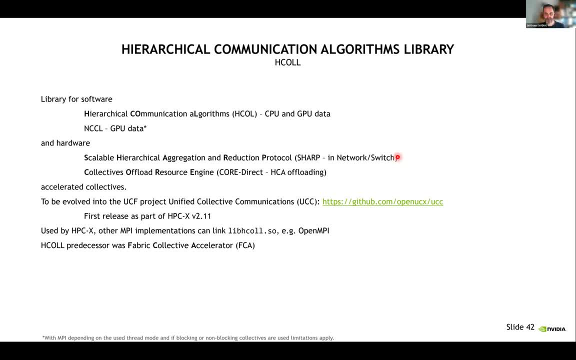 beginning for software and hardware accelerated collectives. So it can leverage, for example, a NICL backend for highly tuned LATCH data collectors in GPU memory. but it also comes with its own highly tuned communication libraries for CPU and GPU data And it can also leverage hardware acceleration. 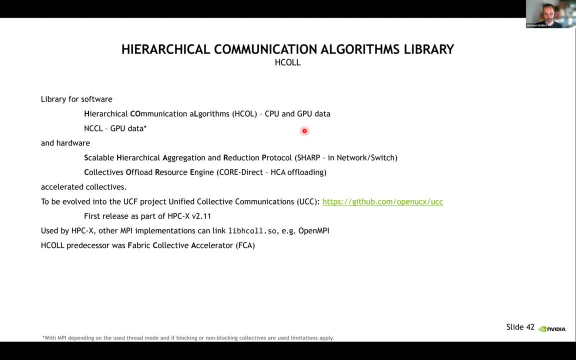 for example, this scalable hierarchical aggregation and production protocol SHARP for in-network switch computing and co-directing. The first it actually. I'm using that for my experiments, but this project actually just evolved into a successor project, unified communications, which is under the UCX umbrella. 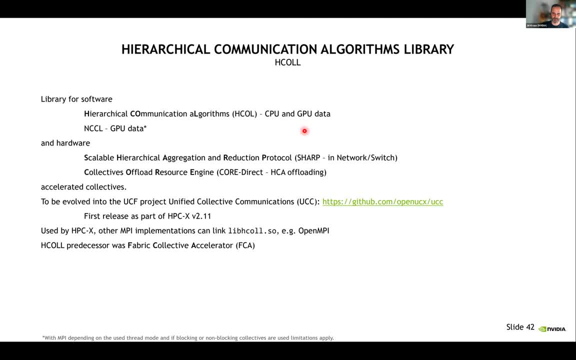 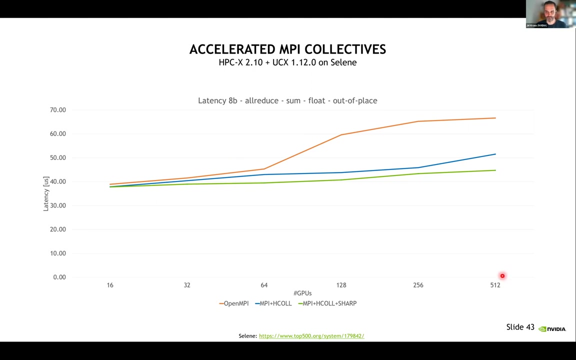 and was the first release was done with HPCX 2.11 released this April. MPI implementations can link to UCC or H-CALL to accelerate, to improve the performance of the collectives and, for example, OpenMPI has that feature. And I've run two performance experiments on Selene with 16 to 512 GPUs, so up to 64 nodes. 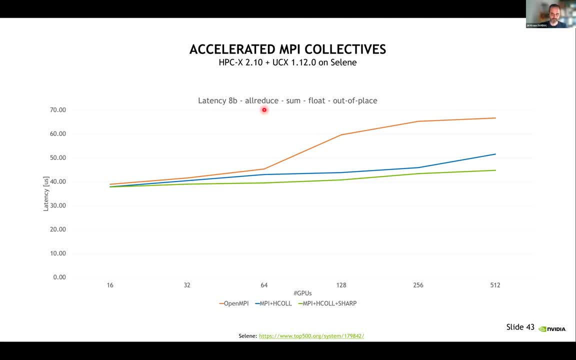 and I've looked at the latency of an 8-byte all-reduce of two float values, so an 8-byte all-reduce float out of place, And I've compared the plain OpenMPI performance just using H-CALL and using H-CALL and SHARP. 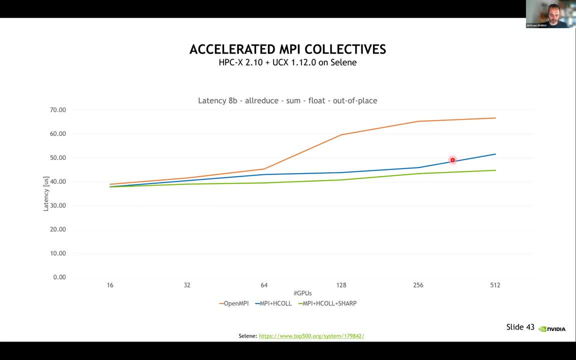 And what you see here, that with H-CALL you get far better latency and you get better latency than with OpenMPI. so that's an optimized algorithm and this is even further improved with SHARP, which gives you almost flat latency, irrespective of this case For large collectors now switching to one gigabyte. so 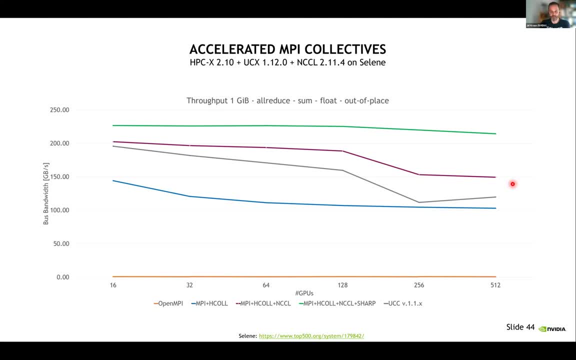 for example relevant to data parallel deep learning training, the differences get even more severe. so if we utilize H-CALL with the nickel backend and SHARP, we can fully saturate the network bandwidth and get an. even so, the per node bandwidth is actually 192 gigabytes, and so we get even an amplification factor by the network compute and get an almost. 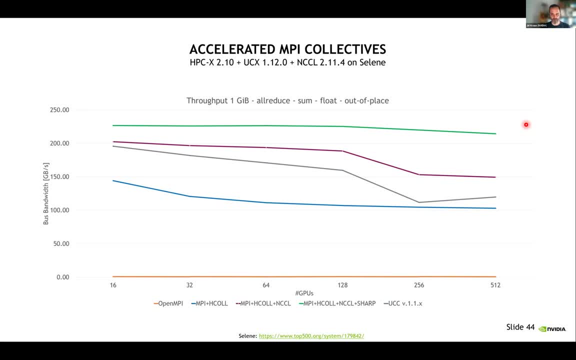 flat performance Over the number of GPUs. here the OpenMPI performance is totally not competitive. I'm just plotting it here for completeness, not for comparison, because for GPU data the plain implementation, OpenMPI, is just known to not be very highly tuned. so if you have large 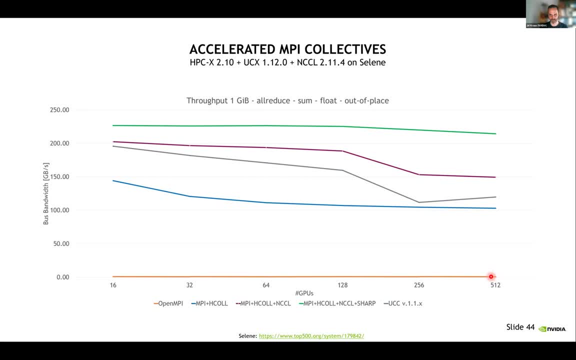 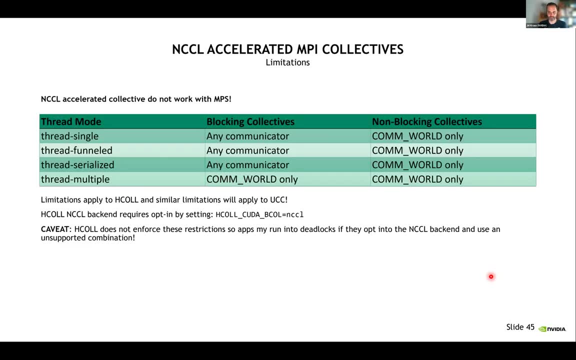 reductions to do, it's really advised to use something like H-CALL or UCC. If you want to accelerate nickel as the back end, there is some limitations you need to be aware of. First of all, nickel accelerated collectives do not work with MPS and you have to consider which. 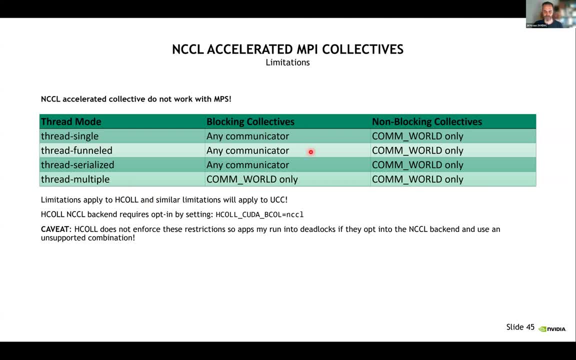 step mode to use, and if you're using blocking and non-blocking collectors, then there are some restrictions apply which communicator you can use. This is enabled by setting H-CALL, CUDA, BQ Call to equals nickel and then if the nickel chat library can be found by H-CALL, it will be picked up. 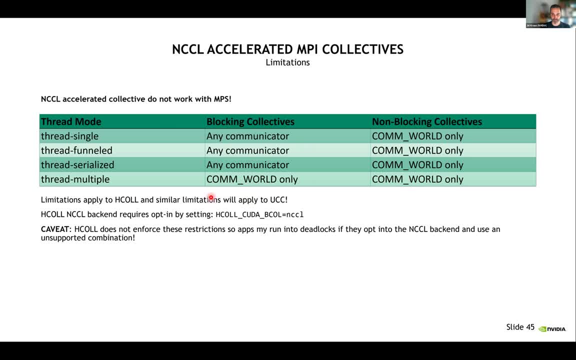 Important point out: the restrictions here are not checked by H-CALL, so and they don't enforce it. so if you violate them, you might run into deadlocks or corrupted data if you're using unsupported combination. so that's just. that's a caveat here. Okay, switching gears again going to GPU acceleration of legacy MPI apps. 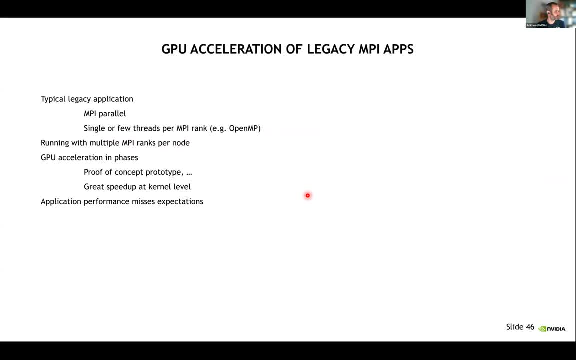 So when you have a MPI application written without GPUs in mind, so large parts of the code is only MPI parallel. but you have. you want to GPU accelerate. so you have already accelerated the hotspots kernels and now want to have an early return on your investments. you want to see a speed. 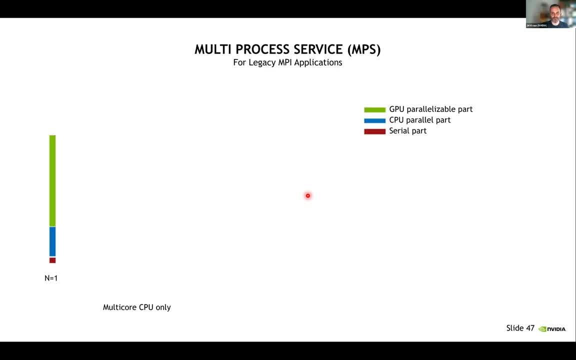 up kernel. What often happens if you, for example, have an application where we simplified structures like this, where you have a serial part that's not parallelized at all, but the rest is paralyzed with MPI and part of it you have also paralyzed with GPU. so this is not amount of code but runtime. 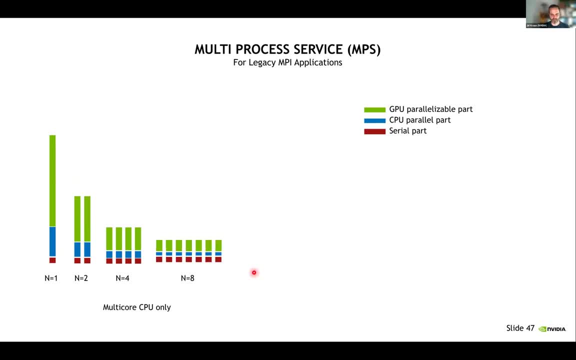 If you scale that code on the CPU it scales nicely with MPI as the original code and if you go to the GPU you also see a nice speed up of the GPU accelerated path but you don't get the output overall speedup because you don't scale up. you're not benefiting from the 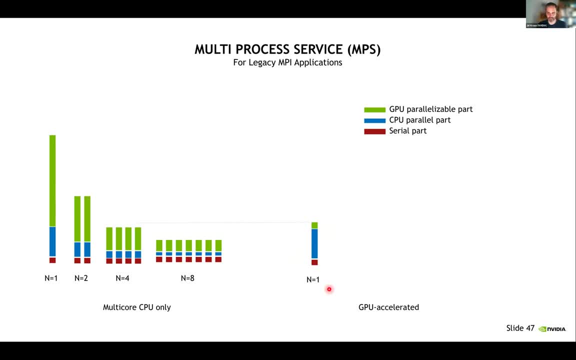 scaling of multiple MPI ranks of the not yet GPU accelerated parts. And that is where multi-process service or MPS, comes in, because you can just launch multiple MPI ranks per GPU so that they share the GPU and you can combine the GPU speedup of the already accelerated part with the MPI. 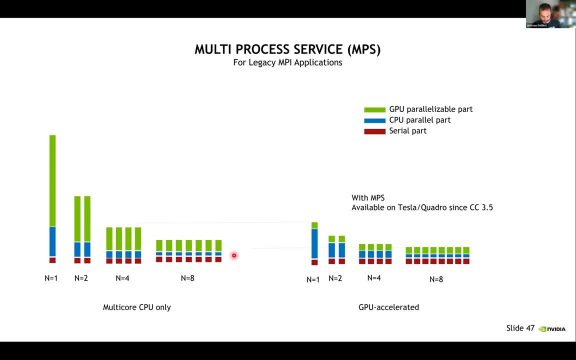 scaling of the not yet accelerated parts. So sometimes I get the question: like that's actually what I would expect it to be possible anyway. so why do I need MPS? Why don't I just launch multiple processes per GPU? Reason is that how the GPU works. 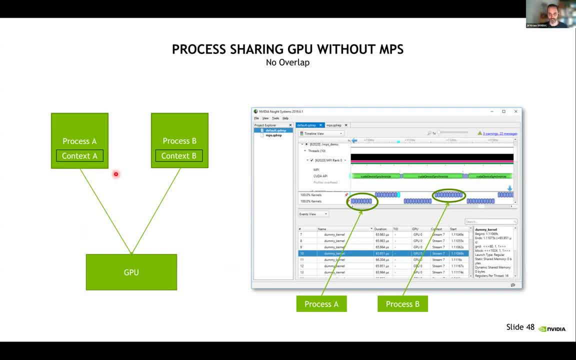 and if you don't use MPS, each process has a separate context. on the GPU Context is kind of an equivalent to a process on the GPU, And now the GPU only serves one context at the time, so different contexts can be active on the GPU at the same time, but they're time-sliced. 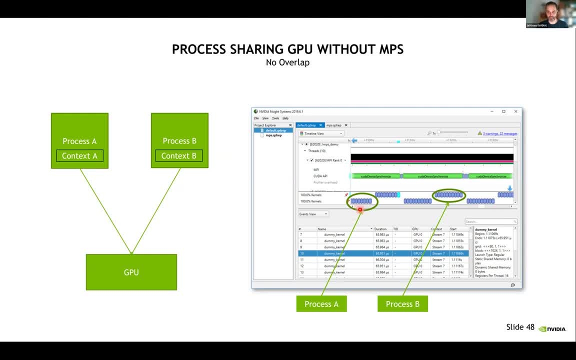 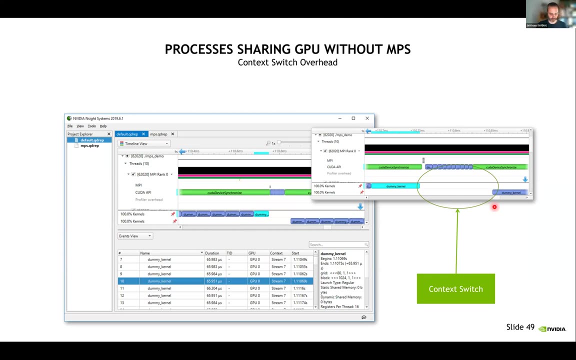 using it. So first process A executes, then process B, and so on. So we are not really using both, are not really using the GPU concurrently, even if they are free resources. And also, not only that the operations are serialized, there's also a relatively costly 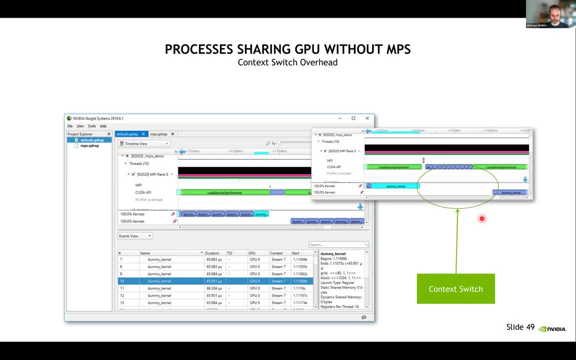 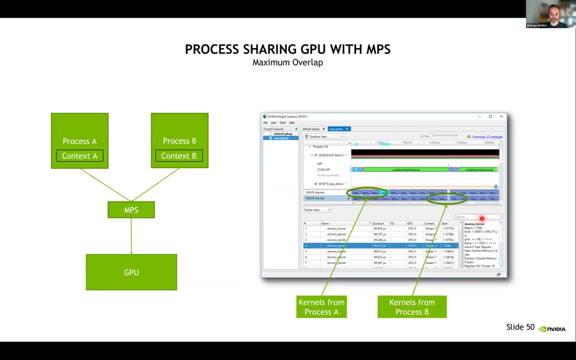 context switch overhead between when work is switched between one context and the other. Both can be avoided by using MPS. Then both processes can submit work to the GPU concurrently and this work can execute concurrently if there are free resources And we also avoid the context. 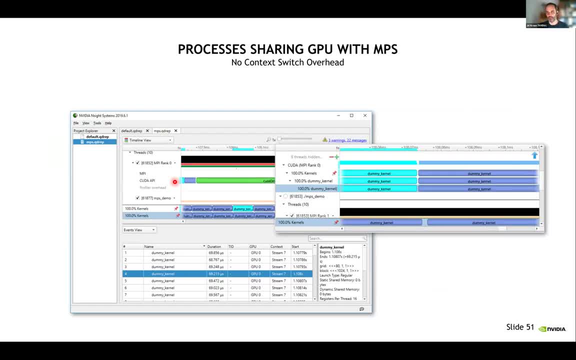 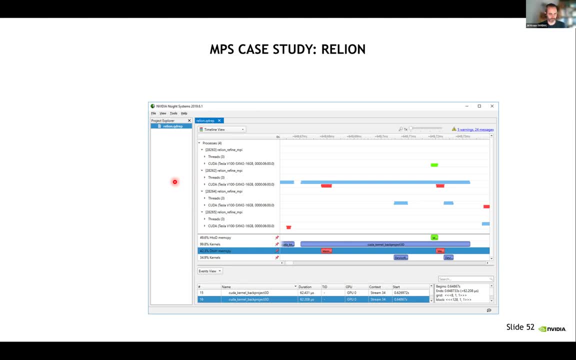 A real word. example is RelIAM, which is a cross-processing tool for crystallography imaging, And it benefits from MPS, And there the oversuscription enables multiple things. So it enables, for example, overlapping the copy with the compute of a different process. 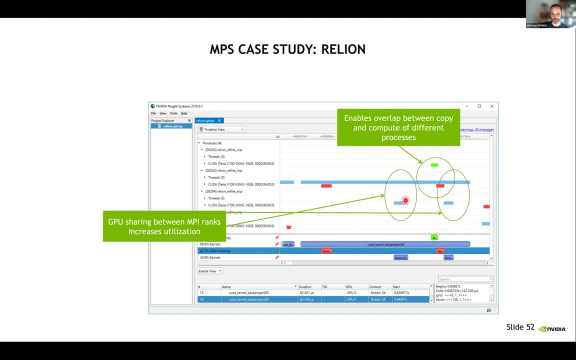 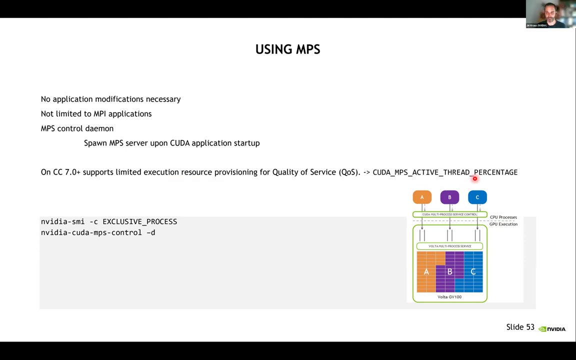 It enables overlapping of compute of different processes, so these small, small kernels from one process overlap with the longer running kernel from another process, not using the whole GPU, and therefore provide a more efficient execution. Using NPS is easy. No application modifications are necessary. It's not limited to NPI applications. 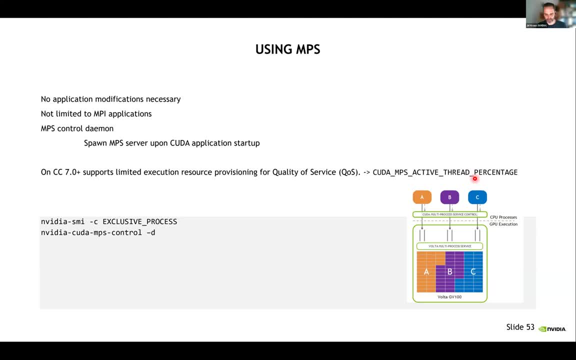 so you could also use it, for example, to pipeline, to use multiple instances of your cross-processing tool, where then the file IO of one instance is overlapped with the GPU computer of the other using the same GPU. Everything happens with the NPS control daemon, which just 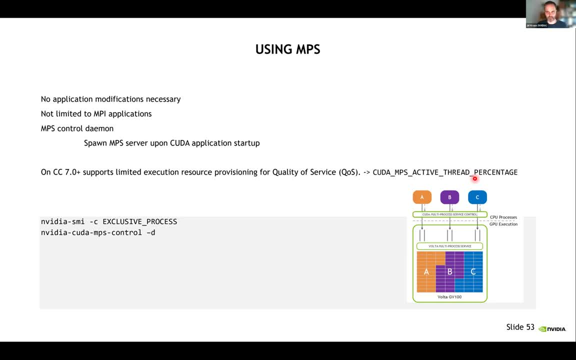 needs to be spawned, started before the application startup and then takes care of spawning NPS servers. And what I also want to mention, that with the Volta architecture or Compute Capability 7, there have been some improvements with NPS, Both in terms of overhead and isolation, but also with provisioning and quality of service. 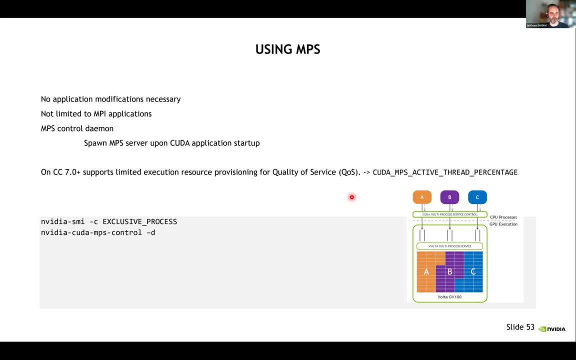 So you can set. Oh yeah, that's a good point. Sometimes you're done by Daniel On, I would say, on most systems reasonably admitrous, that you don't need to. You need to take care that NPS is started, but you don't need to do it. 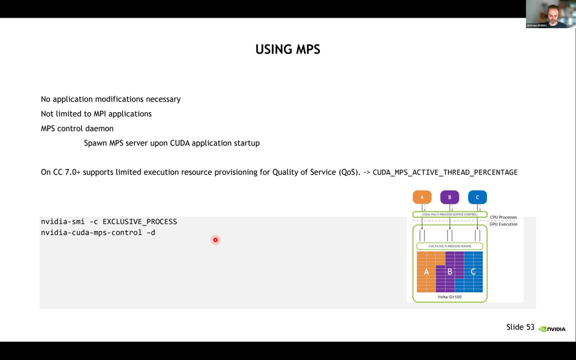 and then you just need to update, because it is not in topics that you are working with. So I want to leave it to you. Daniel, if you would like to comment on the two ways to do this. Yeah, I mean we can, I'm afraid, but there's. 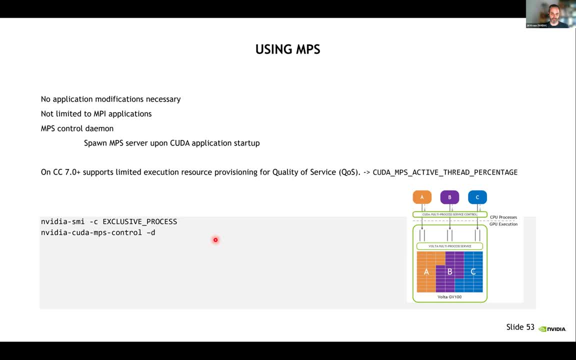 more aspects here. So I think you know it's pretty good to point out that the main process is a kind of a crucial component of the NPS model With the manual process I'm pointing out here, but rather with a common to the to. 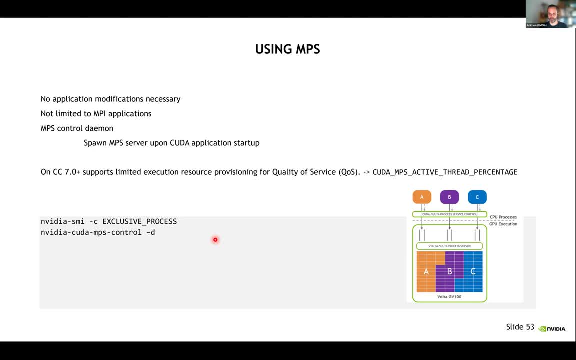 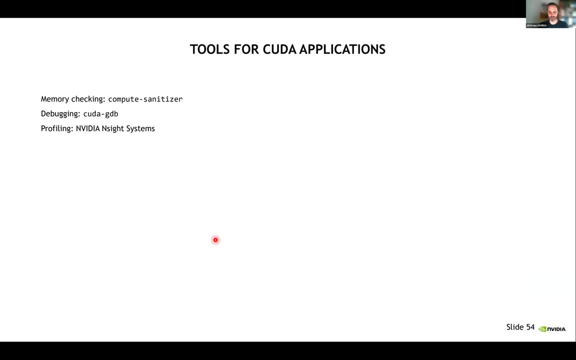 how to allocate your job. Okay, so switching gears again looking into tools for CUDA applications and how to use them in an NPI environment. I've seen from the agenda you have already got an introduction to tools In this series of talks. 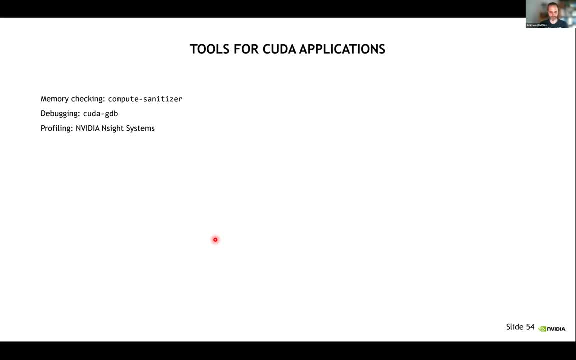 Yeah, I'm not going to introduce, reintroduce the tools. I might repeat some parts because they'll fall into that one, but mostly focus on how to use the tools listed here in combination with MPI programs. so i'm covering memory checking with computer sanitizer, debugging with put a gdb and profiling with such. 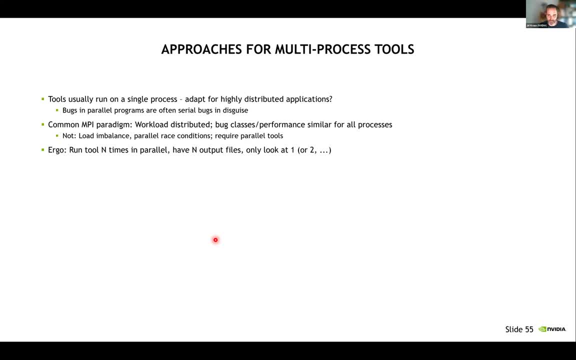 Generally the approach or multi process towards this that They were. they're all for work on a single process and what we are leveraging here, that many box and performance issues and power programs are actually cereal box. so it's not necessary to look at the whole picture, it's just necessary to look at the to debunk a single rank of it. 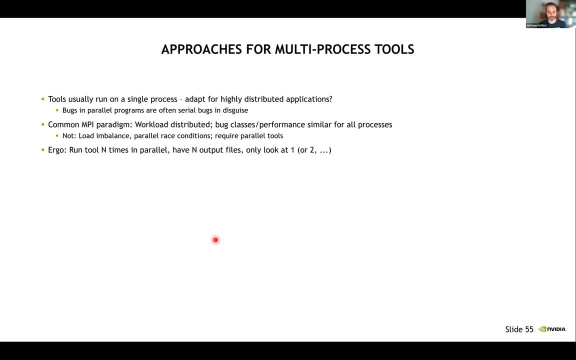 And So the basic idea is: we were just run the tools and times and power, one for each MPI. And how does it work? it works because the tools and allow to specify output files with a special, all the tools support to Put a special syntax into the out, into the output file: name specification, percentage Q and then curly brackets and then, when generating the output file, evaluate that the environment variable named in the colleague. 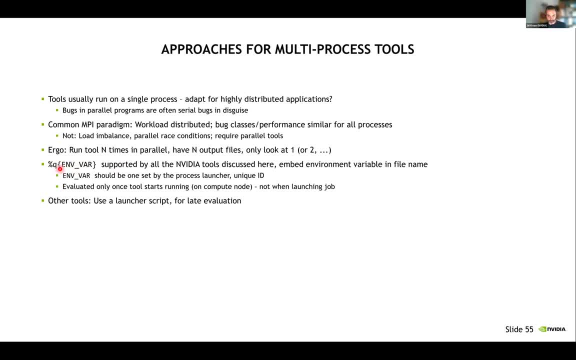 And, And, And, And. here then the environment where we should be replaced by something used by the process launcher, so that a unique ID per output done. no worry, I will show some examples And just One thing you could, for example, use: if you use an open MPI based launcher, you produce or MPI homework rank, but to put into this one, or if you just learn, based launcher through property. 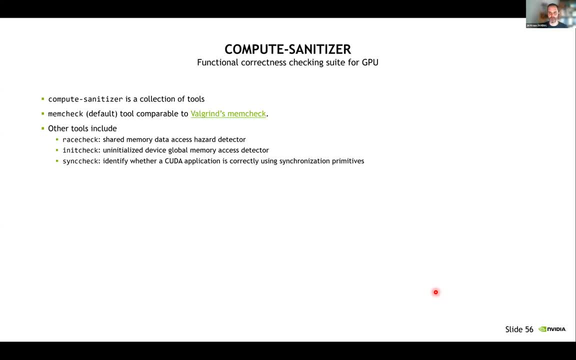 what does that mean? Okay, let's look concretely what this means for competing skies. Just recap: compute, sanitize us. a collection of tools- were men check that? just that before tool, this comparable to while Grünen check. but they're also other tools to check for a shared memory to data access hazards. 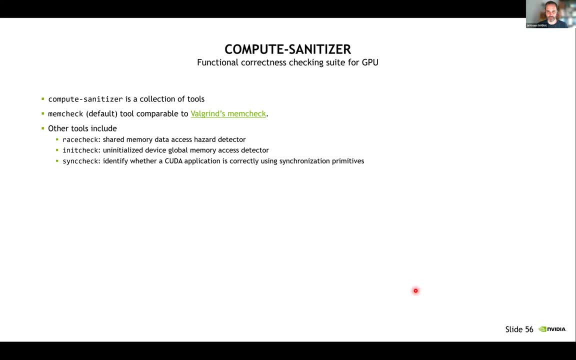 On Initialized initial cherish device memory or go into the details of these tools, just how to use compute sanitizers with multiple MPI rings, And that works, as already explained, in a Mapstrike way by launching one instance per MPI ring. So after our, for example S run, 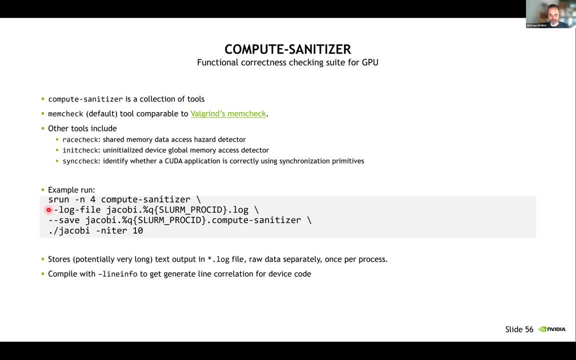 we put compute sanitizer And then we make sure that every instance of compute sanitizer writes to a different output file by using this percentage, queue, curly brackets, syntax, And then finally, of course, our application, And that, in this case, stores two output files. 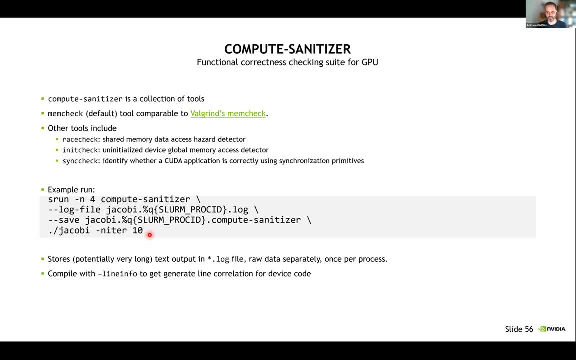 one textual output in the log file and one raw binary data output for process, And then we can inspect this: either take a look at the log file or inspect the binary output by reading it with compute sanitizer. One tip here, most probably to repeat: 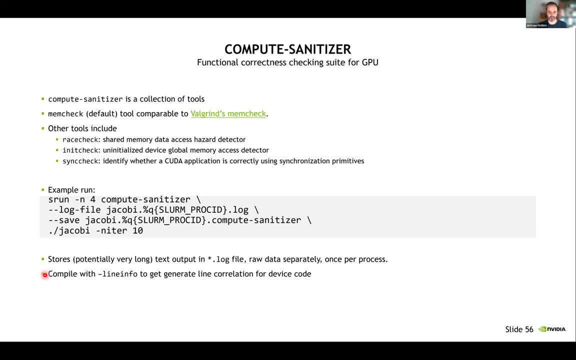 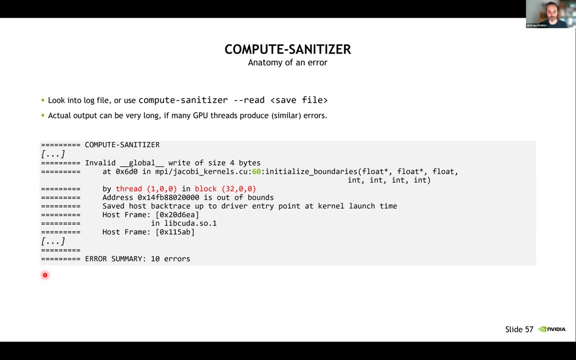 if you use compute sanitizer, compile your code with dash line info to get line correlation for device code without getting the full overhead of debug information enabled with dash capital G. Yeah, then if you look at the individual output files, the output looks less familiar. 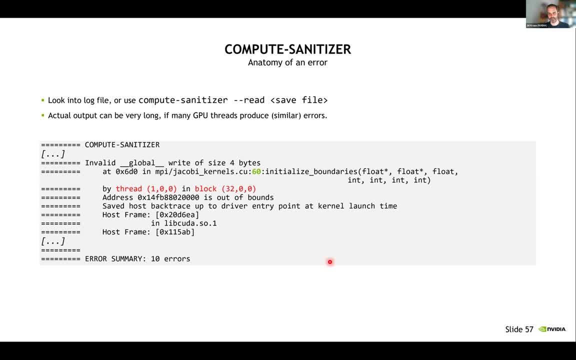 as you know them, with compute sanitizer, for example, an out of bounds access, for example in this line, would look like that We have an invalid global read and then the threat is pointed out and which, if compiled with dash line info, 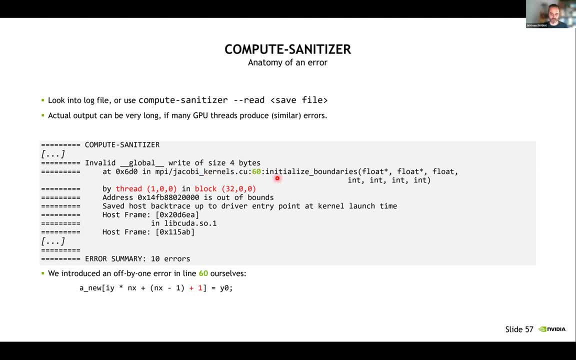 the source code, the source file and the line info of the line where this actually happened. Okay, that's often. I would say this tool can solve already a lot of bugs and you don't need to dive deeper. but sometimes you need to dive deeper with CUDA GDB. 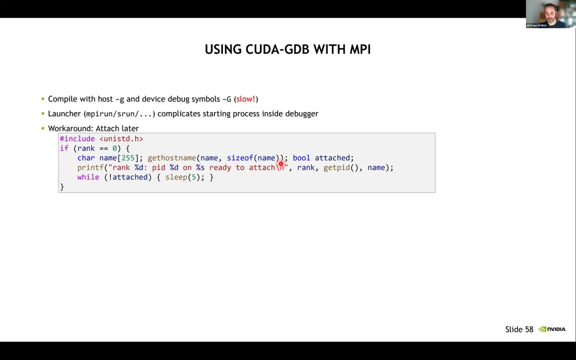 And CUDA GDB also works with MPI, for example, with the usual tricks that you can use with GDB. Of course, you need to compile with debug symbols not only on the host with dash small G, but also device debug symbols with dash capital G. 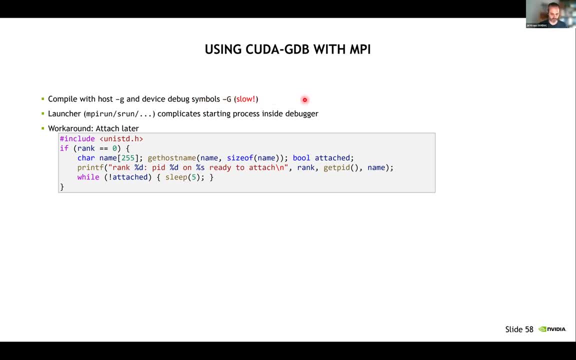 Be aware this really slows down your application. So you only want to do this for debugging runs and probably want to size down your problem where the problem greep produces. And yeah, the first trick to work with GDB, with MPI, is just a general GDB trick. 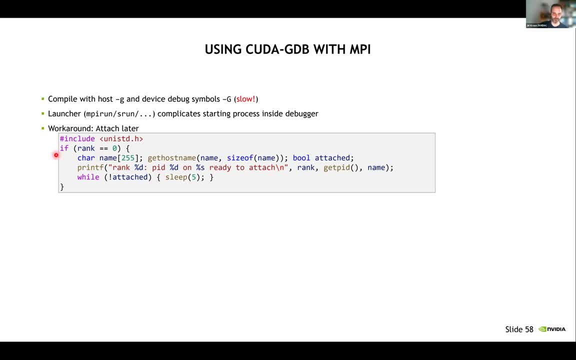 You just attach later, So you add code like this: that the rank you want to debug prints it's the host name, it runs on and the PID, and that it's ready to attach, and then enters an infinite loop so that you can rock into the node. 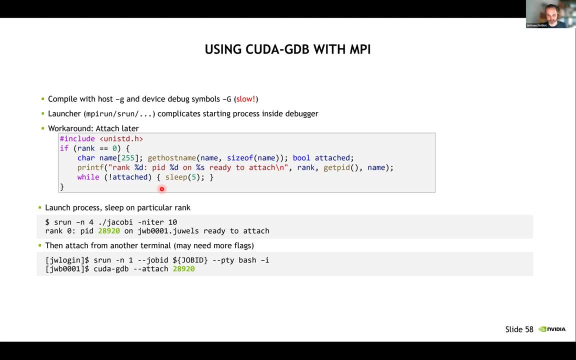 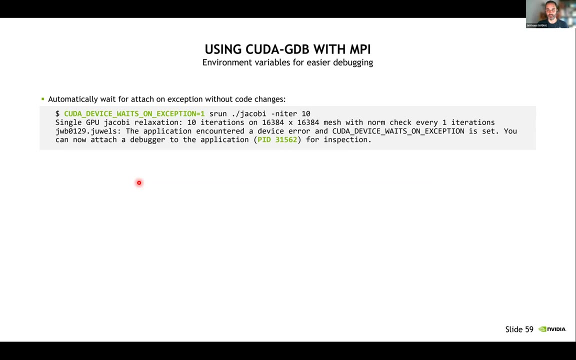 where this MPI rank then is stuck. where this MPI rank then is stuck, Attach with CUDA GDB and change the variable so that the rank exits that loop and then you can start debugging your problem and hopefully identify the issue Next. but there are some things. 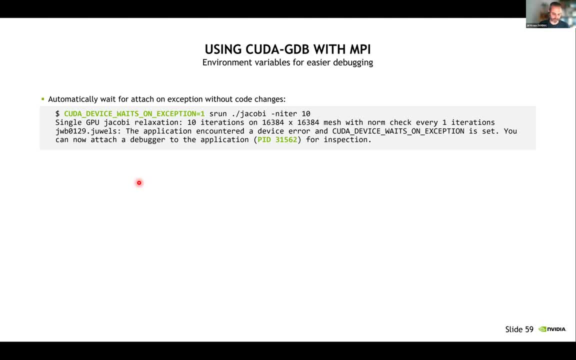 that makes it more convenient. For example, what I just shown in case of exceptions, this process is actually automated by the CUDA drive. By setting CUDA device weights on exception, the CUDA driver does exactly what what the code I've just shown does. 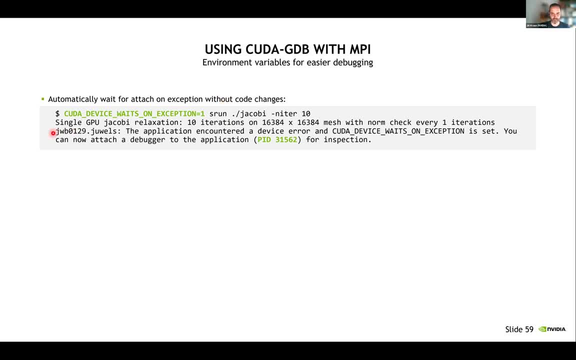 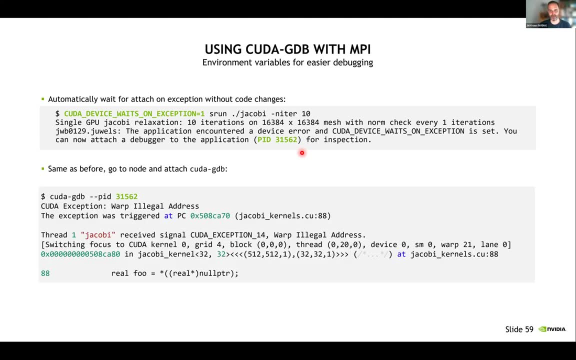 in case a device exception appears, It prints the host name where it happens and the PID and holds the processes so that you can use that information to lock into that node and use CUDA GDB to attach to that process and inspect the program state to hopefully root cause the error and then fix it. 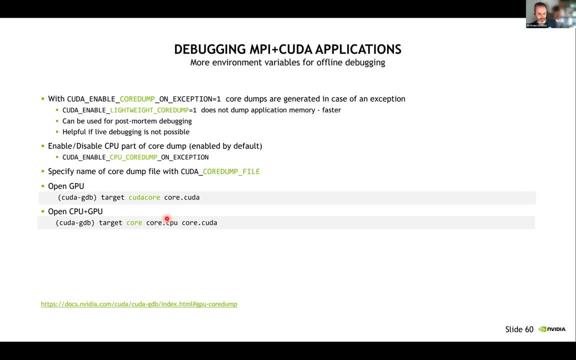 And sometimes- this is this interactive debugging- just doesn't work because the scale where the problems occur is too large, And in this case you can also generate quadrants And the environment variable to set for that is CUDA and then the quadrant on exception. 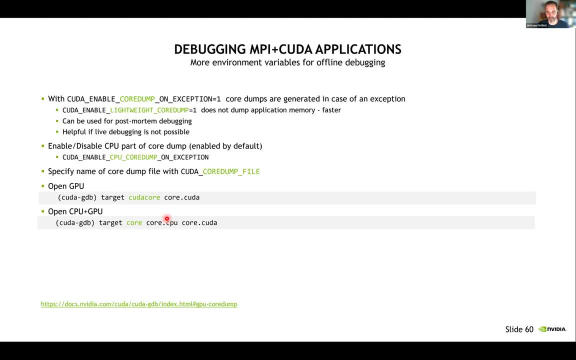 And then there are two other relevant environment variables to name out. First of all, you can include a CPU coder or not, and you can avoid dumping all application memory to make it faster by setting CUDA and then the lightweight equals more. Then, after your error, are reproduced. 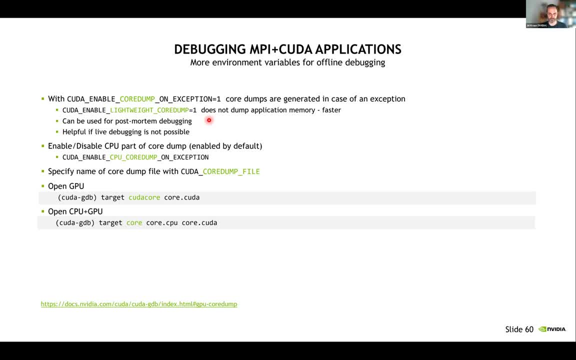 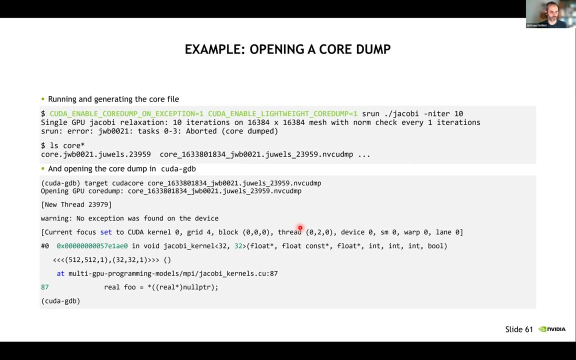 and you have the codems. you can just start CUDA GDB and open your codem as you're used to. You open in codems with GDB and inspect the state of the CUDA codem and to hopefully root cause your error and fix it. 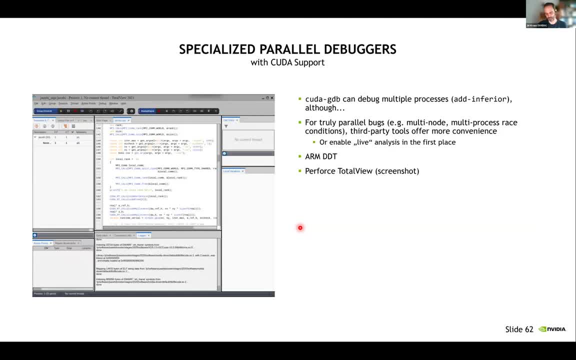 And of course, there are specialized parallel debuggers, which far more convenient interfaces and more powerful features. So yeah, in this case. so if you have access to those, yeah, really use those. For example, ARM DDT or Perforce TotalView are very powerful parallel debuggers. 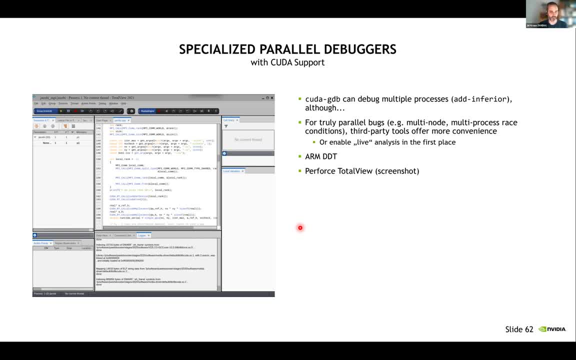 also with support for CUDA. Okay, now you understand- should hopefully understand- how CUDA WMPI works in principle, why it works, how to correctly launch this, how to fix application bugs. So next thing is to look at performance, and that can be done with the 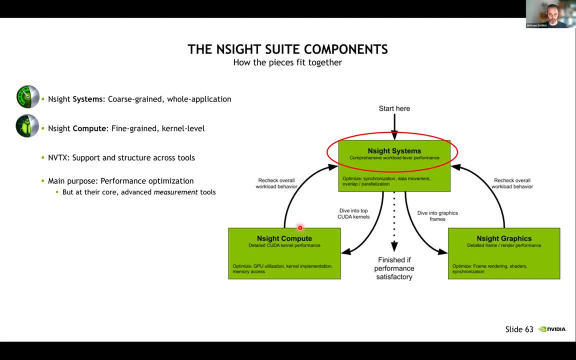 inside systems profiler, which looks as the whole application in conscious to inside compute. So in case of MPI, so the per kernel optimizations with inside compute would happen on a per rank basis. We're not covering that here. We are focusing really on the timeline behavior. 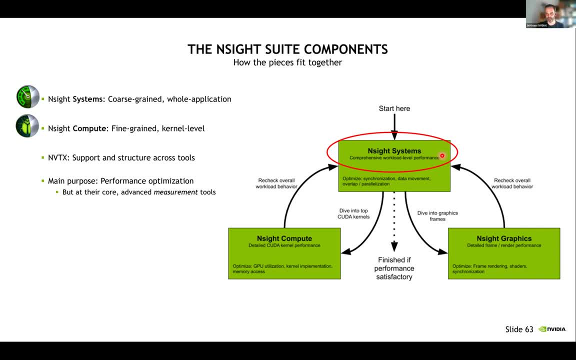 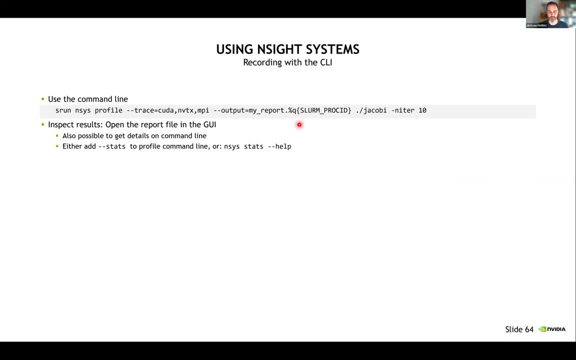 which is relevant for parallel applications. inside systems, Similar to the debug tools, we use the percentage queue So we can do a syntax and generate and launch one instance of inside systems per MPI rank to get one application trace per MPI rank And then we inspect the results. 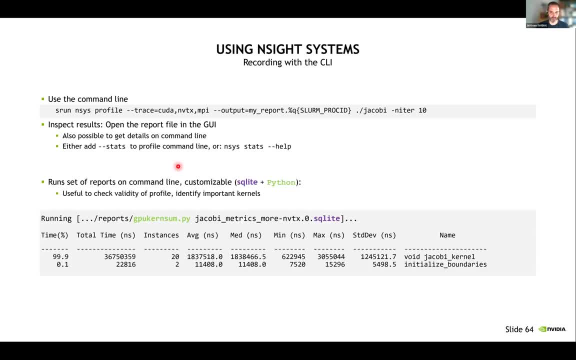 by opening the report file in the GUI, or use the or on the comment line, for example with the stats function, which gives you an output like, for example, this initial high level overview, where most of the time it's spent. So we can do that. 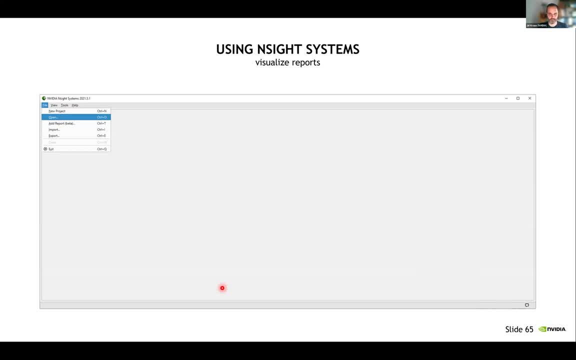 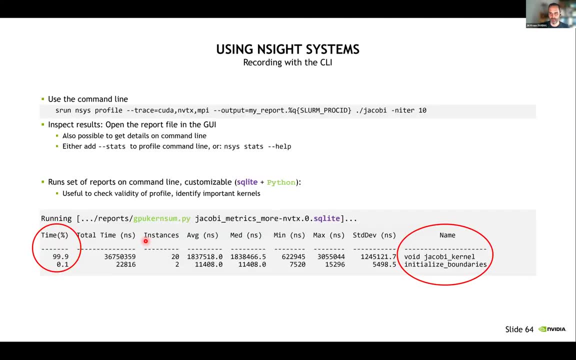 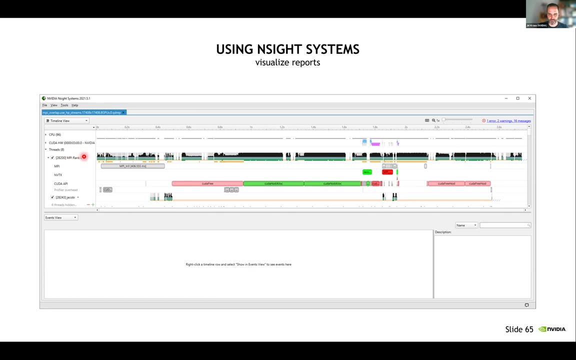 So we can do that. So we can do that, And inside system, you're just open and then you're get a timeline. This way, you then see if you profile with MPI tracing enabled once you get extra information, like labeling of processes with MPI ranks. 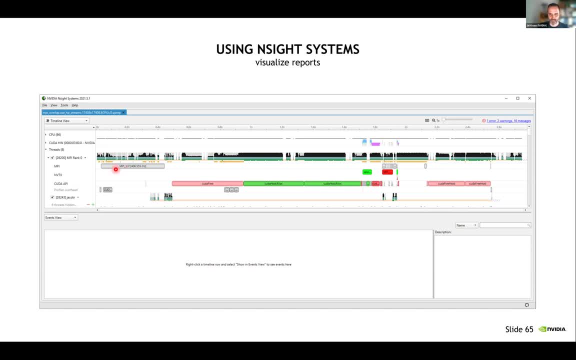 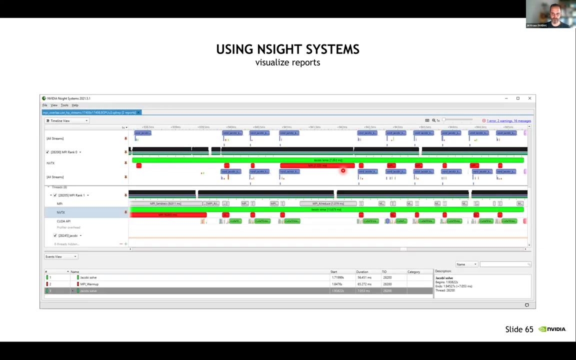 labeling of contexts with MPI ranks. you get MPI traces overlaid to those and, yeah, all the familiar features of inside systems. So you can really also inspect the communication behavior And you can also add multiple reports to one single view so that you can see. 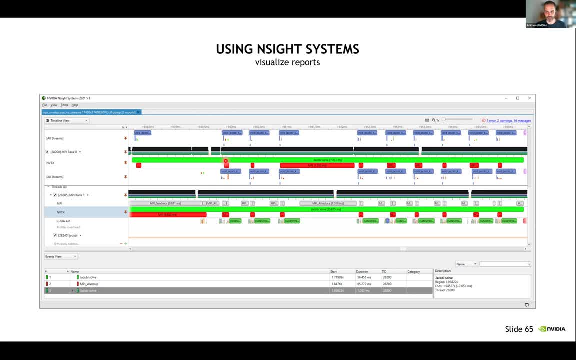 can correlate the behavior of different MPI ranks And for example, here see that this already use probably takes longer because something is delayed And on rank one because something is delayed in rank zero, And also if you click on the individual MPI buttons. 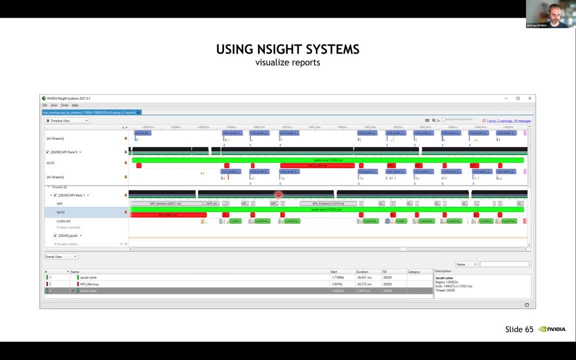 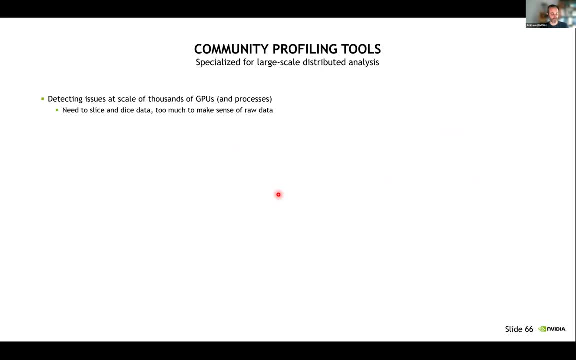 it gives you an MPI sections. It gives you some information like: what is the source rank, destination rank, How much is the message that was exchanged? As with debugging, there are also other tools which are more powerful for large scale profiling and with And which might be necessary because, the same as with debugging, detecting issues at scale of thousands of GPUs is really complicated. 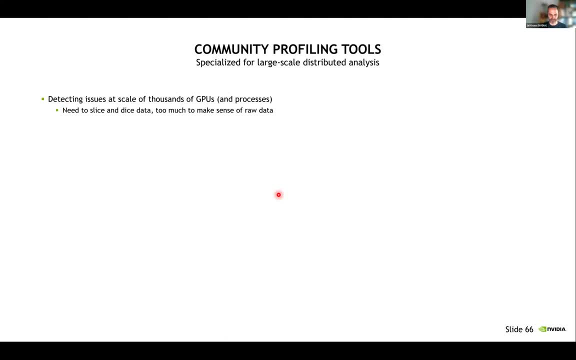 So you need to slice and dice data because there's just too much data to make sense by looking at the timeline as NSAT system presents you The community tool, a very popular community tool, which is CUDA. we have Scopee So you can use Scopee to instrument your OpenACC or CUDA or standard language parallelism application and generate a Scopee trace. 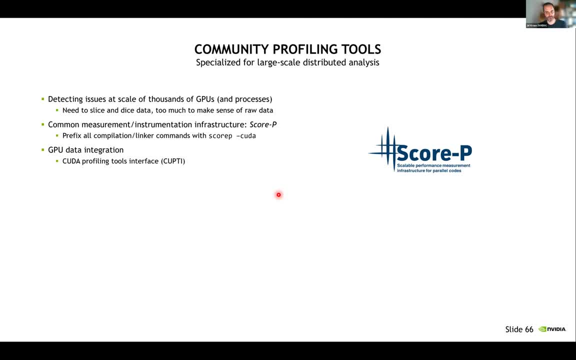 Scopee internally use the CUPD CUDA profiling tools interface API to get information also about GPUs. Then you collect that trace and then you can analyze it with all the performance tools that go Scopee, for example Vampir, Tau and so on. 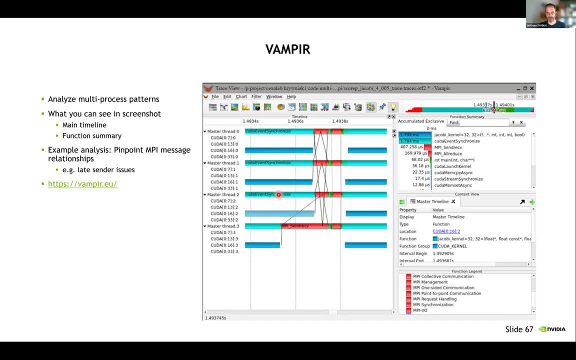 So here's just one example of a Vampir screenshot with a CUDA timeline of four processes. Okay, so what do you do with? I want to close the talk with some optimization tips to work around common MPI performance issues. First, I've run a scaling experiment. 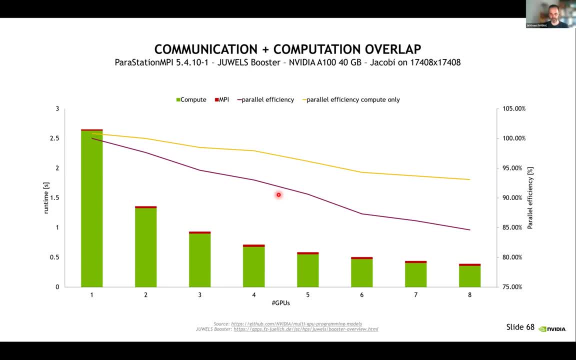 I've run a scaling experiment of the simple Jacobi solver. I have shown you And I've plotted the time to compute and the time to communicate. If we use only a 1D domain decomposition, which I did here in this case, not a 2D, then the time to communicate stays flat because we always need to communicate the same amount of data. 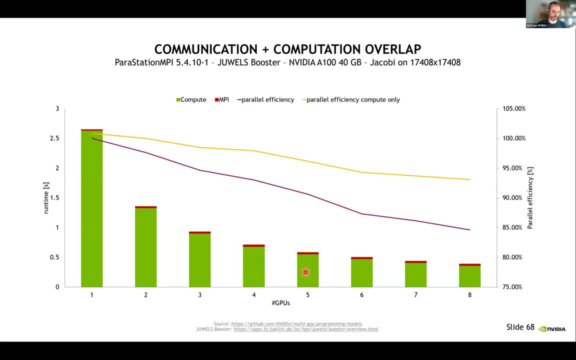 But the time to compute, of course, decreases, because if I add more GPUs, each GPU computes less and less, And that is what we see: that the runtime increases, decreases. If we plot then the power efficiency, we see that this decreases with a number of GPUs added. 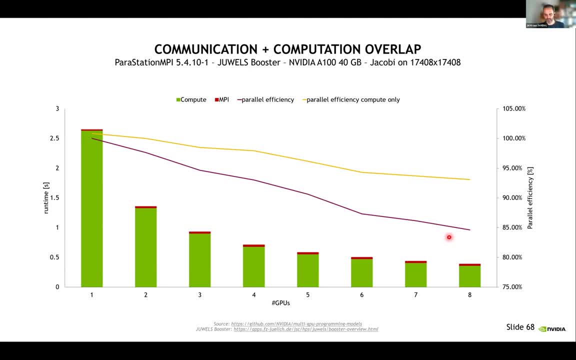 And that's for two reasons. First of all, there's some overhead of coordinating communication at all, But mostly because the absolute time to communicate stays constant, but our time to compute gets smaller, So the relative of time to communicate gets larger. So to highlight that fact I've also plotted the parallel efficiency. 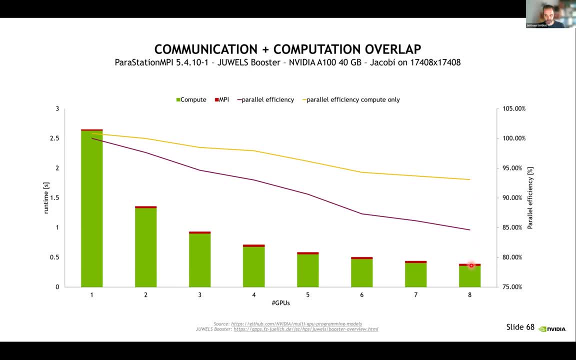 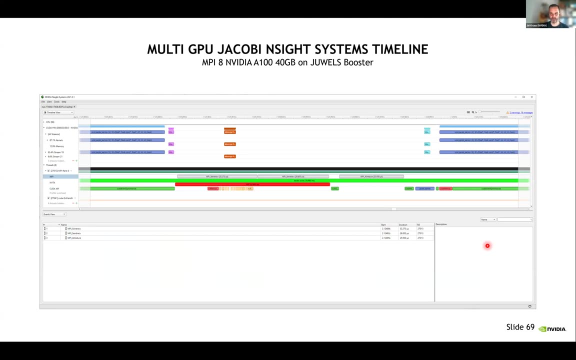 if we would just ignore the time to run to communicate. So that is obviously almost 10% higher. so some performance gain we want to have And looking at inside systems profile of an MPI rank we also see that effect. So we have our communication and then we have our compute. 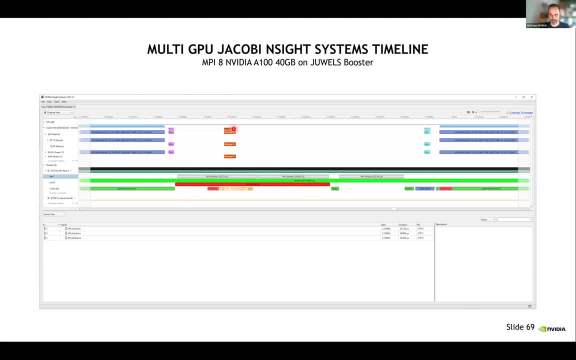 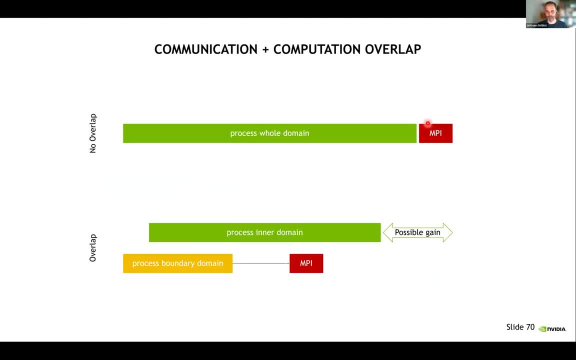 and, after that finished, we exchange our halos and we see that this is done with peer-to-peer copies here. So what we're effectively doing, we process our whole domain and then we do MPI. However, in many cases, and as in this, we can process the domain in any order. 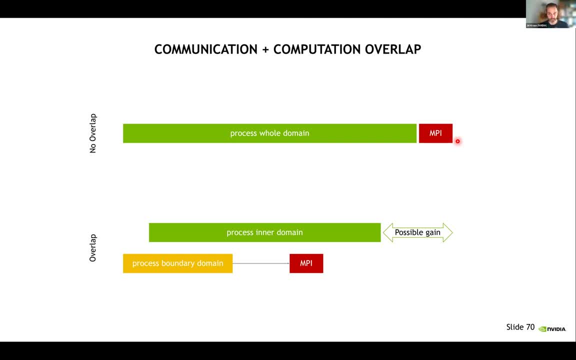 It's our choice which grid point we calculate first. So what we could do is we could split up our domain into the part that only processes boundaries, so that we need to communicate with our neighbors. We are MPI. do that first and as soon as that has finished. 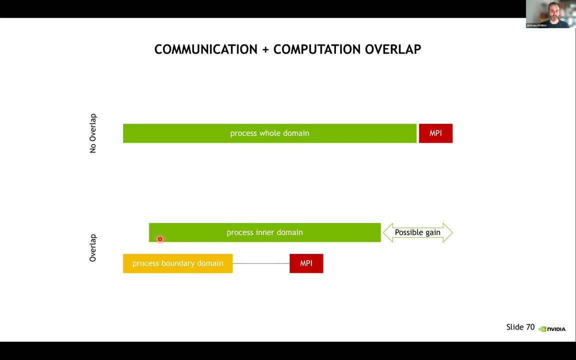 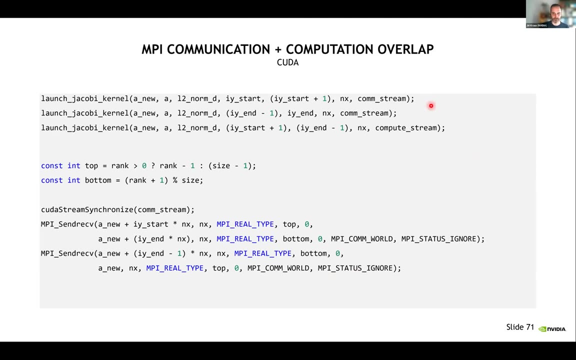 we can kick off our MPI communication early and do it also in parallel with processing the remainder of the domain, effectively hiding the time to do the communication. So how does it work? We just launched three kernels: one kernel and two kernels. 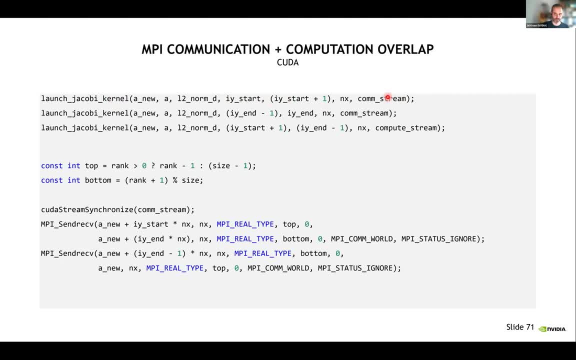 That just computes the first row of our domain into a communication in the communication stream. one kernel that only computes the last part of our domain in the communication stream and after these two are launched we launch the kernel that does the bulk of the compute. 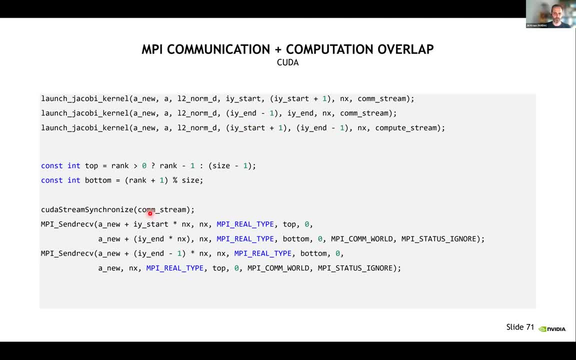 leaving out the first and the last row, And then we only wait for the work in the communication stream. so leave that running, because that is the one that needs to be finished before we can start communicating and then communicate. So, in this way, this 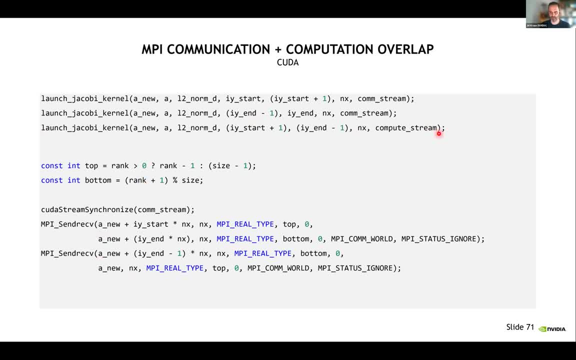 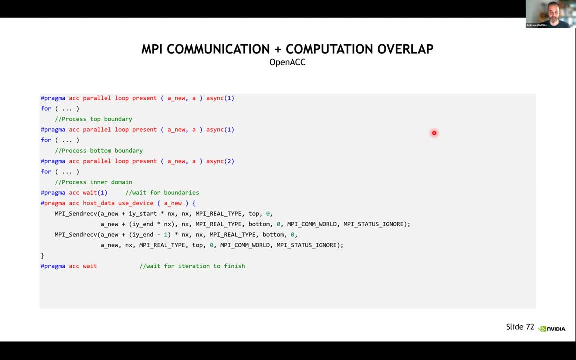 is the way that we can start communication and overlap with this kernel compute. This is with CUDA, With OpenACC. concept is the same, just that we are now using directives to generate, let the compiler generate our kernels. and do we use? instead of streams, we use Bayesian. 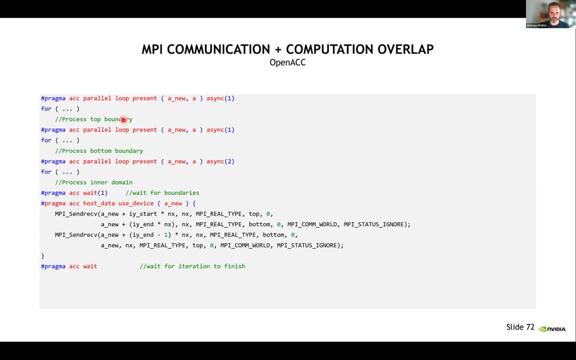 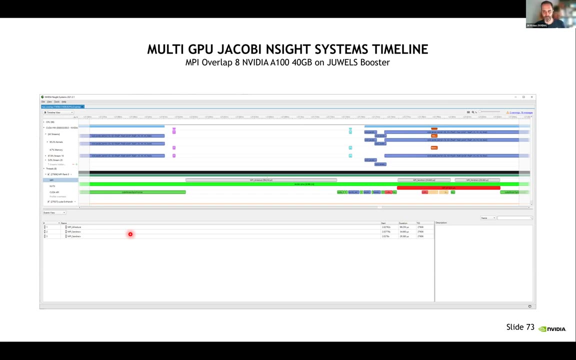 Q identifiers. So Q1 for the computation of the boundaries and then wait for that, and Q2 for the computation of the bounding. So we see that our compute can overlap with our communication. Looking at the timeline, we see that this works now between two iterations We only have our 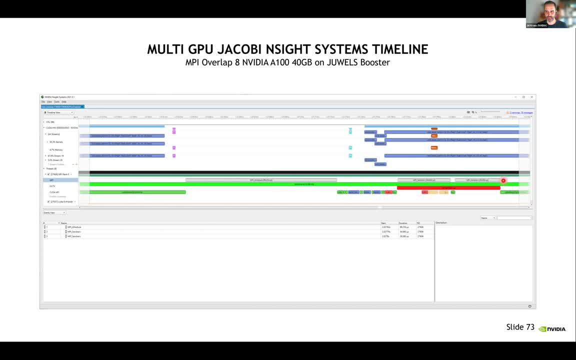 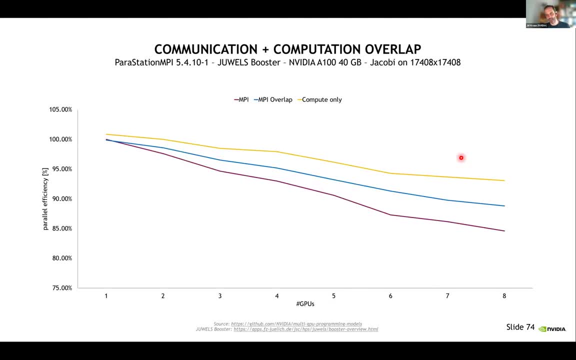 onReduce left. We have our two boundary condition boundary processing kernels and we see that the MPI compute is overlapped with our bulk compute And we still have some parallel overheads so we didn't really achieve the compute-only parallel significant improvement in parallel efficiency by overlapping communication and computation. 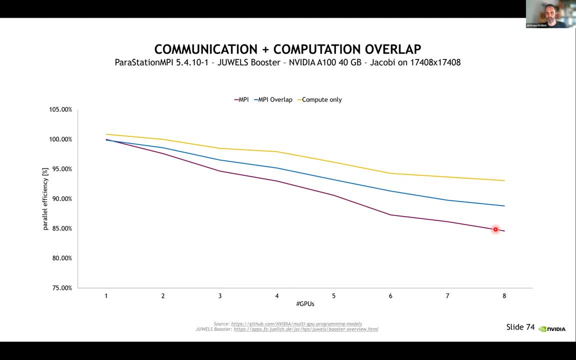 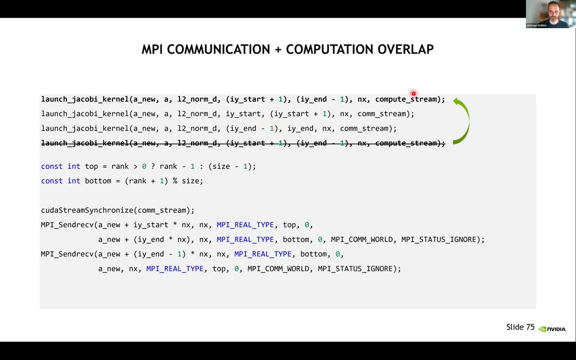 Can we improve that further? One thing is: maybe we have seen some time to launch these kernels and maybe if we launch them first- launch the bug compute- we could maybe also find the time to launch and synchronize these extra kernels by just launching them first. 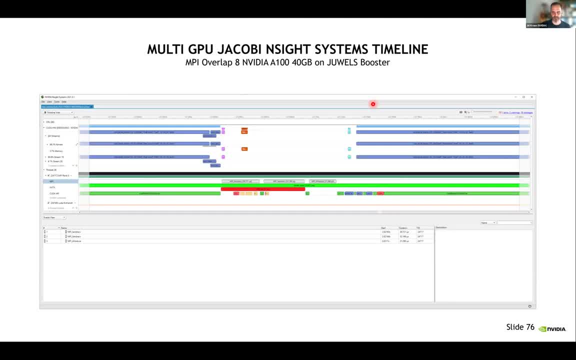 I've tried that. I've captured an inside system profile and unfortunately it does not work. So because the tiny kernels to compute the boundaries where we have the MPI dependency on simply don't get resources on the GPU, because the bug kernel occupies all these resources. 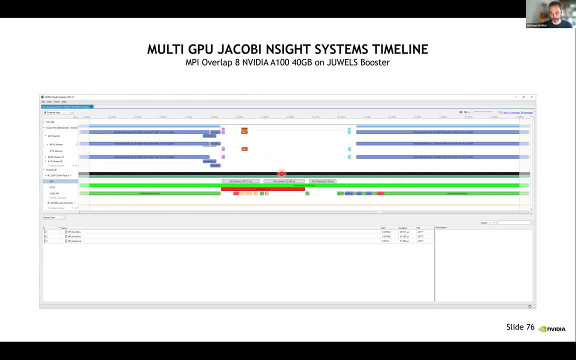 So we are back at the non-overlap, effectively back at non-overlap. So, but of course, I, probably you would, as expected, probably I would not expect this. if there's presented this way, if there's no workaround for it, and it is because we can. 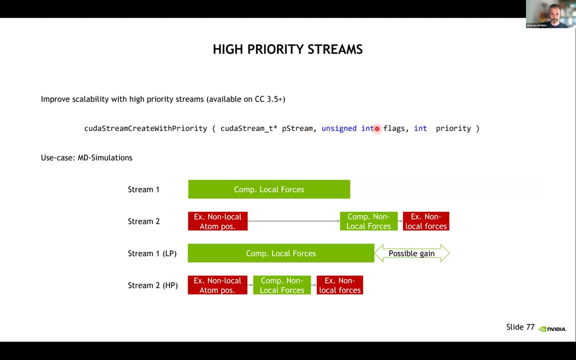 create streams with high priority, And there's also another use case where this is critical to overlap communication and computation, and that is, for example, that is, it occurs in molecular dynamic simulations, where you have to do communication before you can do the compute on the data that needs to be communicated, again Without high priority streams. 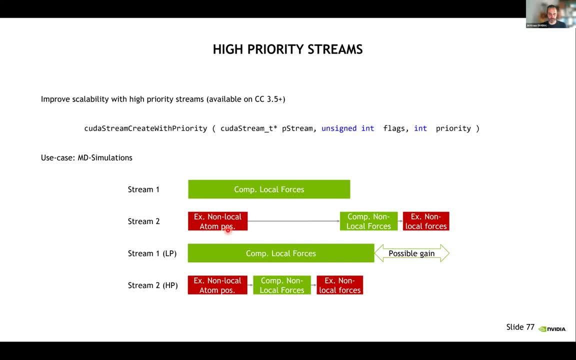 you would end up in this situation: You overlap the communication you need to do first with the com, your main compute, but then you can't overlap the computation that you need to communicate again and therefore your second communication is fully exposed With high priority streams. you can launch this compute- non-local forces kernel into. 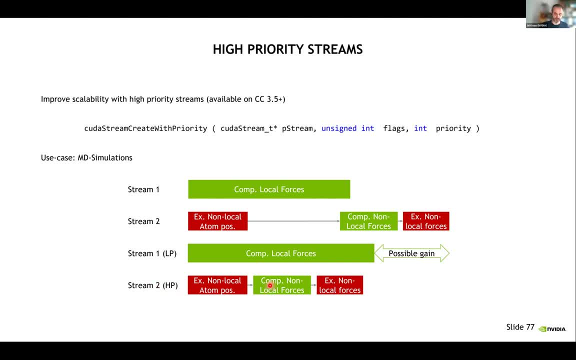 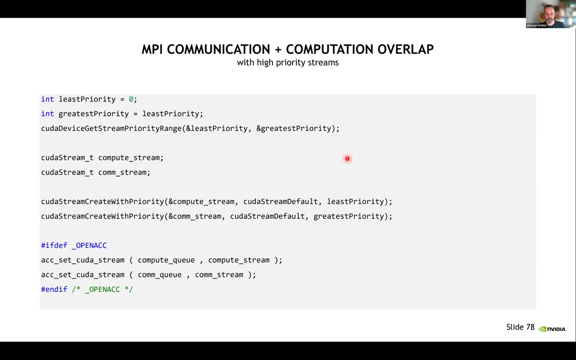 a high priority stream so that the GPU prefers work on that one, to schedule over the local lower priority stream work and also get overlap of the second communication step. How does that look in code? So first you need to query the priority range of the GPU supported. 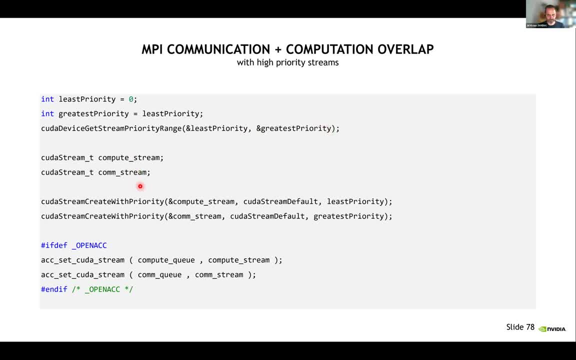 and then you create two streams. We only need two priority labels. so I just for simplicity I've just taken least priority for the compute stream and highest priority for the communication stream. This also you can also leverage that in OpenACC by using the ACC set CUDA stream. 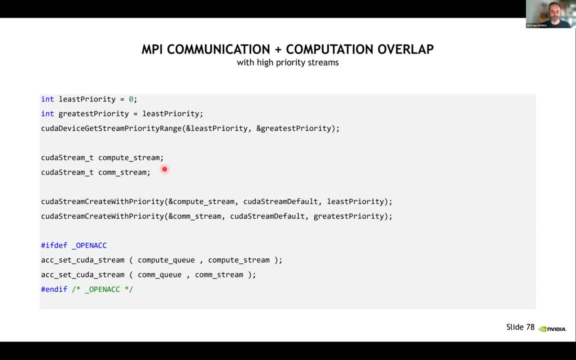 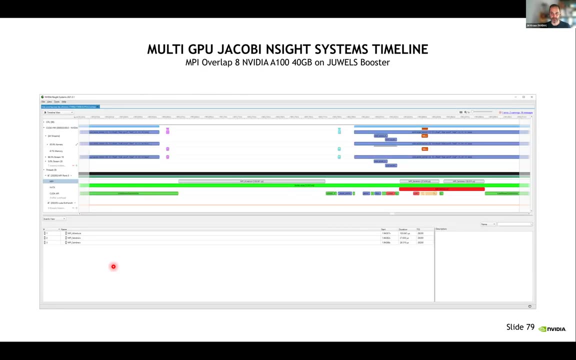 OpenACC API to tie a high priority stream you have created to a Q identifier of OpenACC and then use that Q identifier in your async losses. And yeah, if we do that, we see we get an end communication computational overlap of your communication with the power compute. 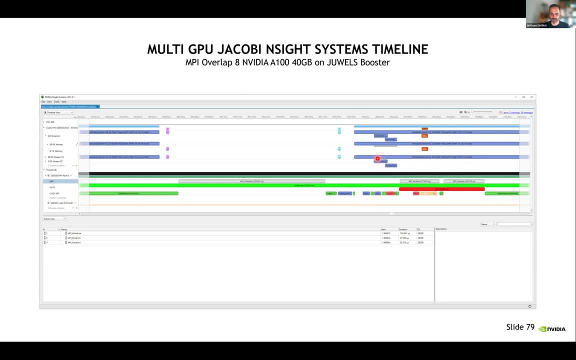 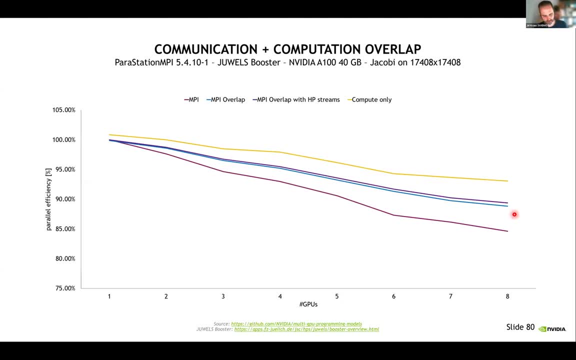 Also the launching of our tiny kernels overlap with the bulk compute and we get a slight increase. In this case it's not that significant. it's only a slight increase, but depending on cases that might be larger in performance. Okay, Last but not least, one last trick. 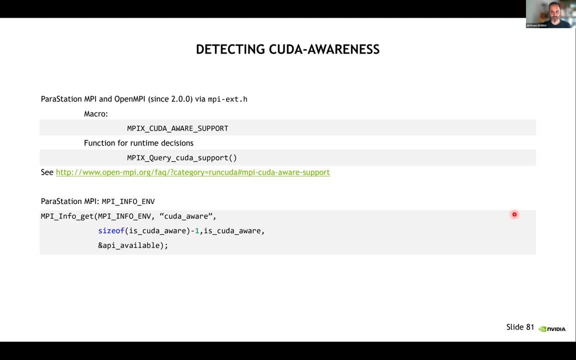 Detecting CUDA awareness, which might be helpful for your build system. PyroStation and OpenMPI expose, via the MPI-x header, some macros and the runtime function to query CUDA awareness at runtime so that your application can warn error out or choose a different application path. 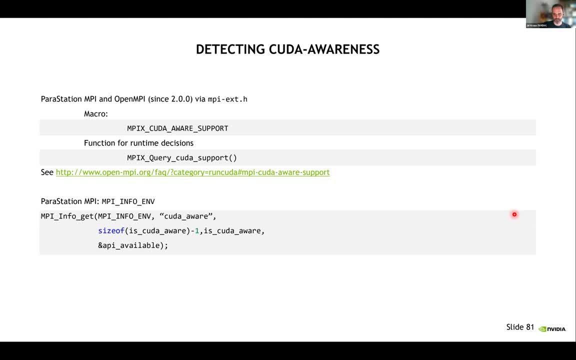 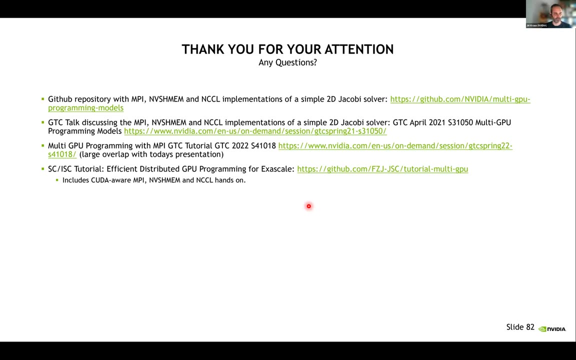 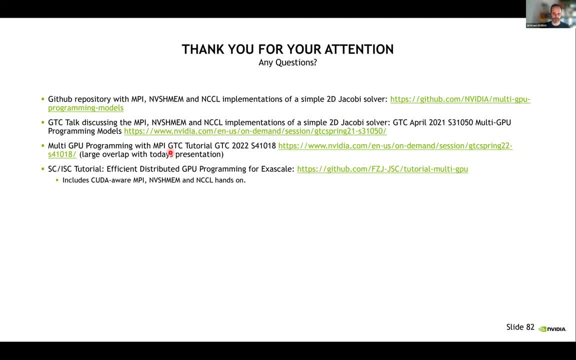 Pointing out a few more resources. First of all, multi-GPU programming with MPI, GTC tutorial, which is available on the NVIDIA on demand. This is, as a large overlap with today's presentation, just a little bit more. And there's a GTC talk where I go a bit more detailed in comparing MPI. 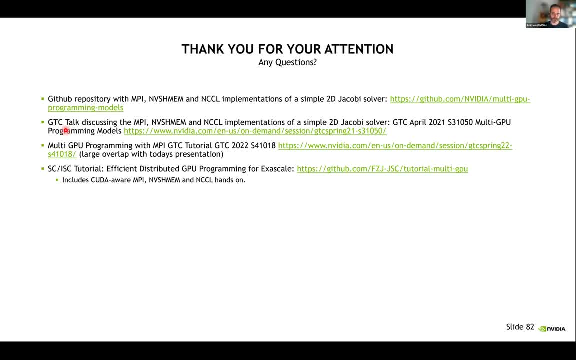 and the Schneider-Nickel for a simple, by using a simple 2D Jacobi solver to really compare the models performance-wise and do a bit more detailed comparison. how to express the same algorithm with all three variants? The one presented here is also available on GitHub. 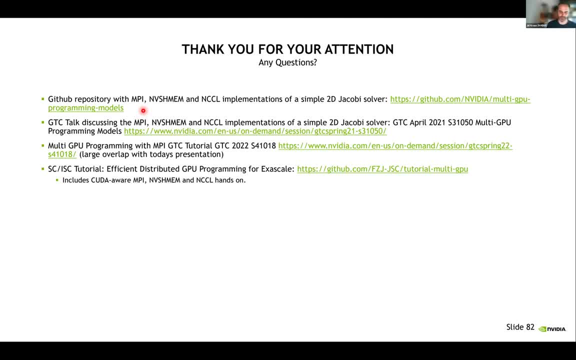 which tends to be a very simple code written once in MPI- MPI with overlap, Nickel, Nickel with overlap. and so that you really can compare the different models And the Schmem and Nickel use MPI. These are similar in terms of interoperability and, for example, 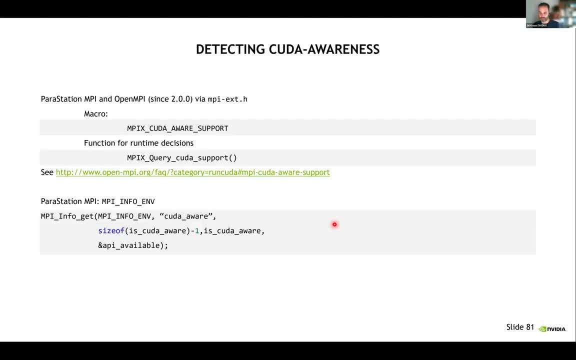 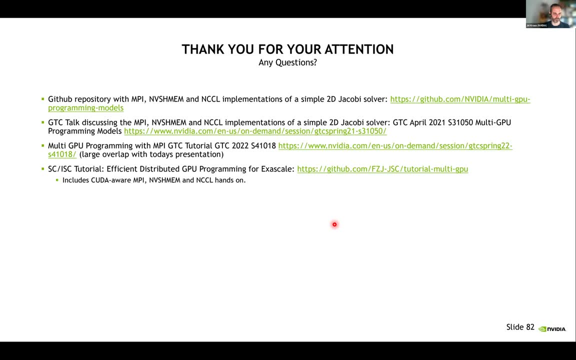 the MPI version here also has examples of handling GPU affinity or detecting CUDA wins. I hope this was useful for you and time to take some questions. Thank you, Jerry. Any questions, feel free to submit them into the chat or raise your hand and we can answer the most recent. 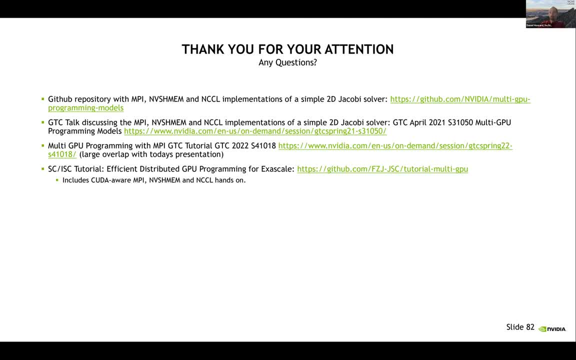 Thank you, Jerry. feel free to submit them into the chat or raise your hand and then we can answer them very quickly. submitted them in the chat or raise your hand and we can answer them very quickly. live over voice, I guess I can have an initial question. 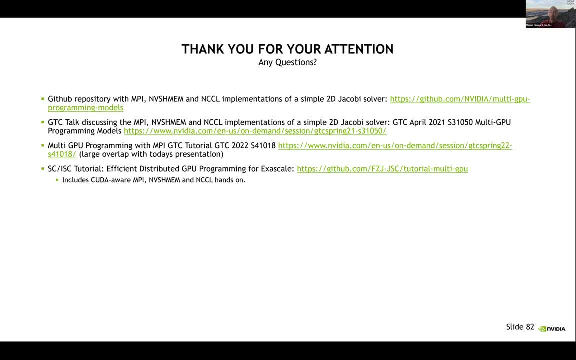 You presented multiple approaches for implementing multi-GPU communication. Do you have a preferred library that balances, say, performance and say time for implementation and effort needed to implement those different libraries? No, I don't really think that there is a general recommendation to make. It's really application, I would say, depending on the developer community. so what kind of portability is needed between different systems? What kind of programming models, what kind of expertise is in the developer community? Then? how large are the performance gains and where the best implementation maps optimally? 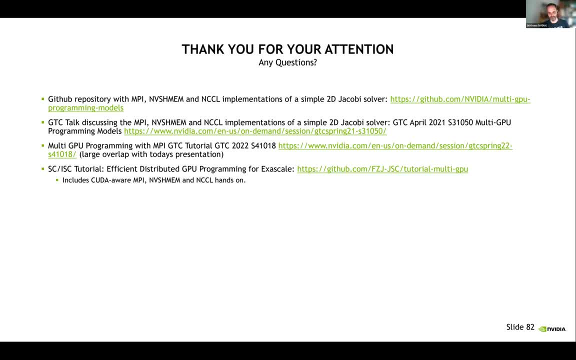 to. For example, there could be cases where the performance benefit of NB-SMEM is relatively small and then it's not helpful to introduce an additional dependencies, but there could be also cases where the performance benefit is really huge, like with CUDA or if you can. 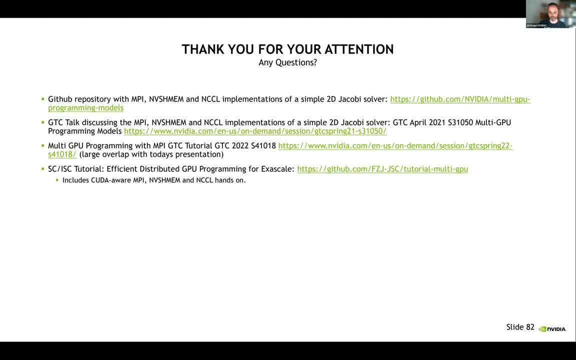 use it to fuse kernels and then achieve a 2x kernel speedup because you can stay closer to the multi-processor. But nothing really is something case-by-case That makes sense. Go ahead, Helen. You're welcome to unmute and ask your question. 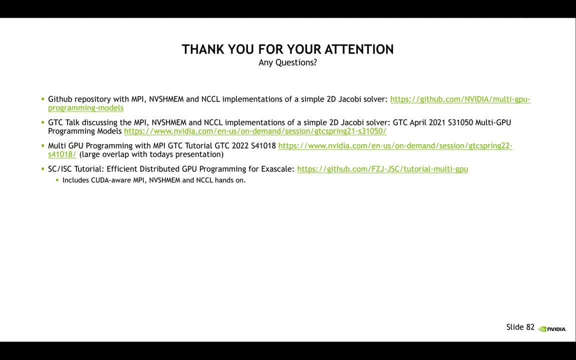 Okay, great, Great talk. I guess my question's more on. so just making code portable across machines, so like one machine might want to use nickel, another that's not available, Is it quite easy to just wrap all these calls up in an MPI wrapper and switch out nickel? 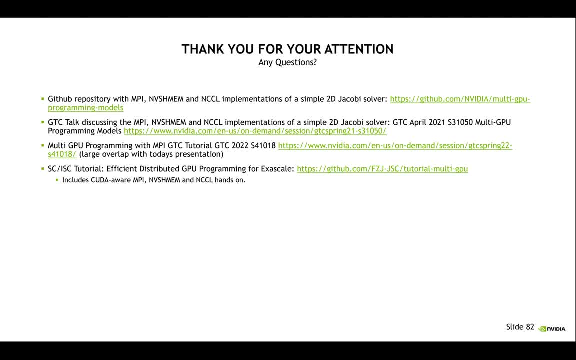 versus just regular MPI, or are there any pitfalls to worry about? if you do that, I would say for many patterns that's probably possible, But I would say that if you do that, I would question if that really makes sense, Because CUDA or MPI implementation are very efficient at moving data. 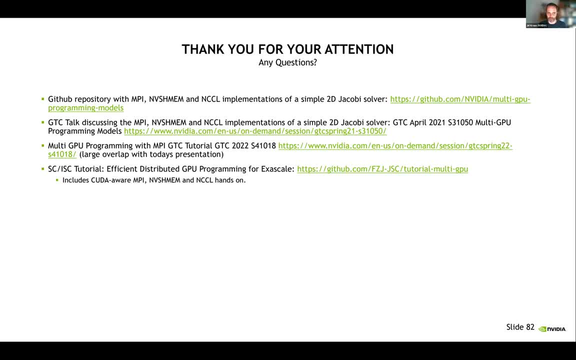 So nickel is not perceived more efficient of doing a point-to-point communication. Benefits of nickel mostly. when it comes to point-to-point communication, the benefit of nickel mostly is due to the stream-aware API And as soon as you wrap it up under an MPI one, you lose that because you're no longer 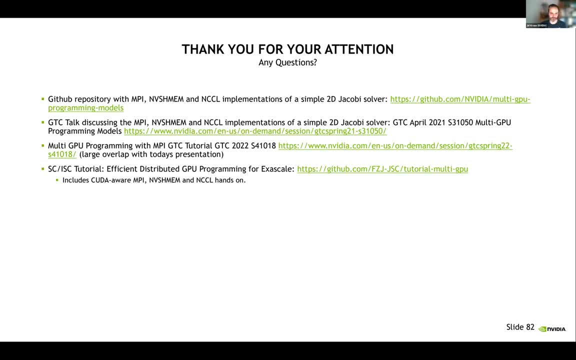 going to pass a stream in and then that benefit is gone. Okay, great thanks. Also, if you have more questions and you're attending ISC and in the tutorial program, I want to highlight that, luckily, an SC tutorial I'm doing together with a colleague and the 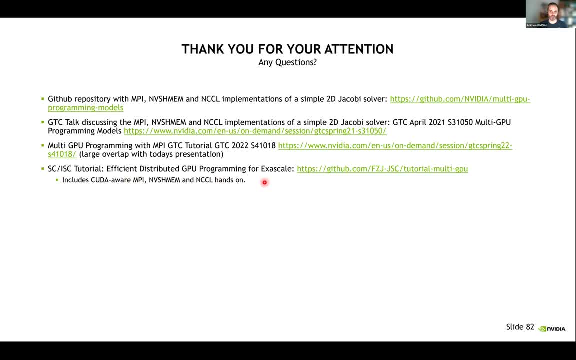 ULIC Supercomputing Center about efficient distributed GPU programming for Exascale. We already did it- last year SC and this year IC- and we will do it again at SC this year. So happy to come to that, And the material, including all hands-on examples, is published on GitHub. 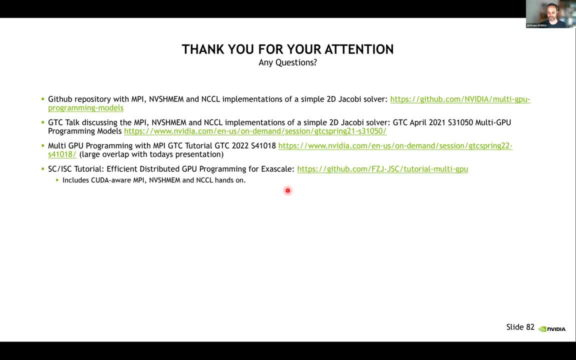 I think that's maybe also helpful for your learning. Thanks, Jiri. Yeah, certainly, the upcoming tutorials will be very useful for participants here and we'll be sure to share those with you. We'll be sure to share those with others. 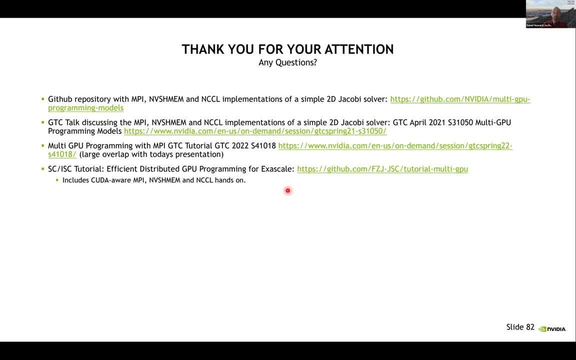 Any other questions from the group before we close out? Yeah, I had a question. I was curious, as you had the example with GPU Direct using RDMA. as you're scaling out applications, do you end up running into PCIe bottlenecks or do you have strategies or? 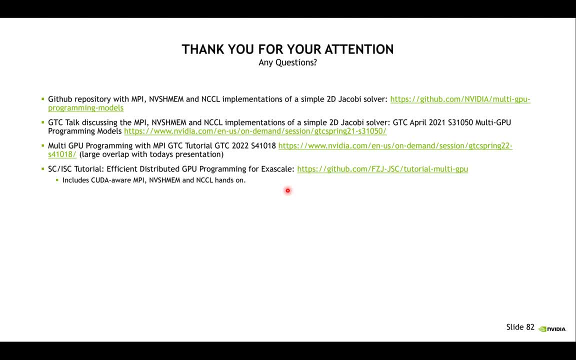 technologies to kind of get beyond if you're fully saturating channels for inter-GPU communications. Yeah, Yeah, Yeah. So with most well-designed GPU accelerated systems, PCI Express is not a bottleneck, And it's certainly not the bottleneck that increases with scale, because I mean the 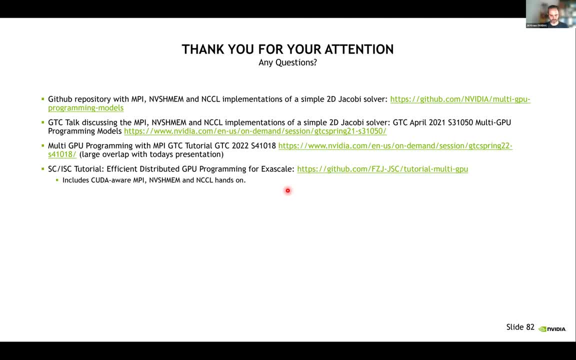 welding was like systems put an HCA close to a GPU so that it only needs to traverse a single PCI Express switch. and then, given that the PCI Express bandwidth, depending on the network technology used, is either slightly higher than the available network bandwidth or significantly higher PCI Express if GPREC-RDMA. 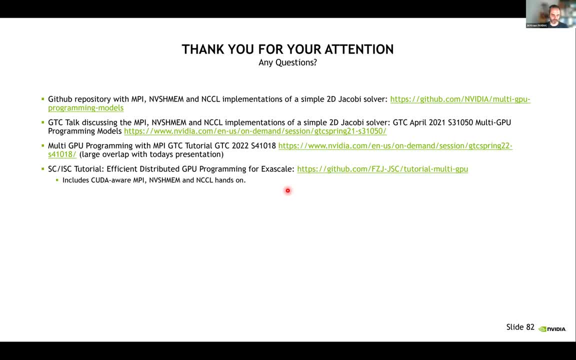 can be used efficiently usually does not tend to be the performance bottleneck, And if it is, it definitely is nothing that increases with scale. The visibility might increase, but you will see that already that, for example, you can certainly build up the PCI Express topology of a node that. 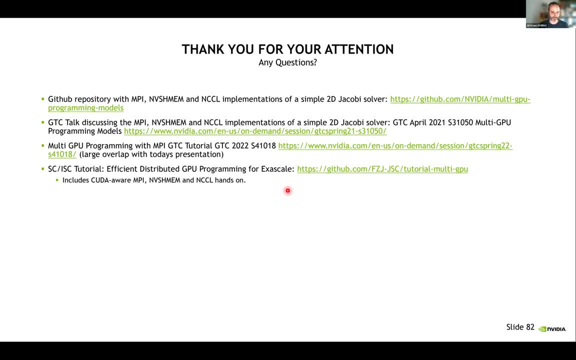 is very unfortunate for GPREC-RDMA communication And that performance effect might be visible into your end-to-end performance only at scale, but you will have the performance issue already at low scale because that is a bottleneck that will cure for every communication. 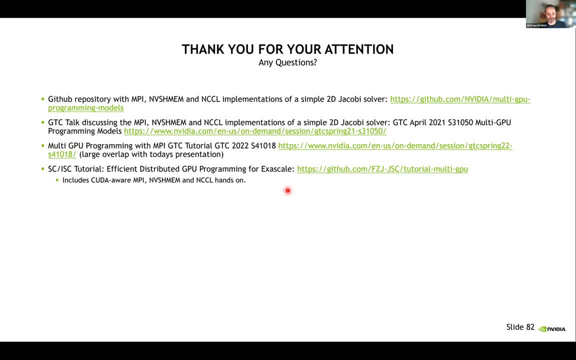 Does that make sense? Help? Yeah, that's great. Thank you, Go ahead, Tina. Hi, I was really interested in the way that Jules has that automatic boost based on topology. We've got a new system coming in. Was that something NVIDIA helped set up with Jules? 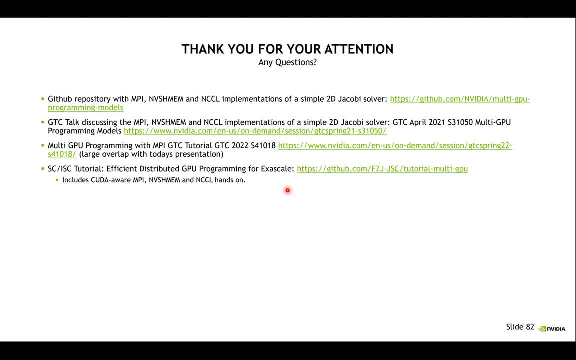 Or I guess, how did they develop it? How did they do that? I was involved in the process by advising on what the right topology is, what are good defaults, But I'm not aware that NVIDIA was involved in actually implementing it, But what effectively the system does on a very high level. 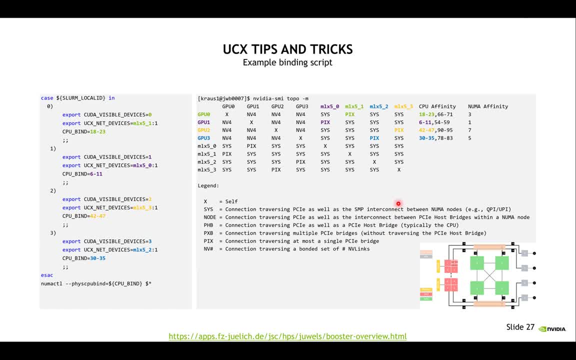 can be summarized on this slide So effectively. the job scheduler uses the NVML API, which is the library that's also used by NVIDIA SMI, to query the topology of the system, And then it just sets these environment variables in the launcher. 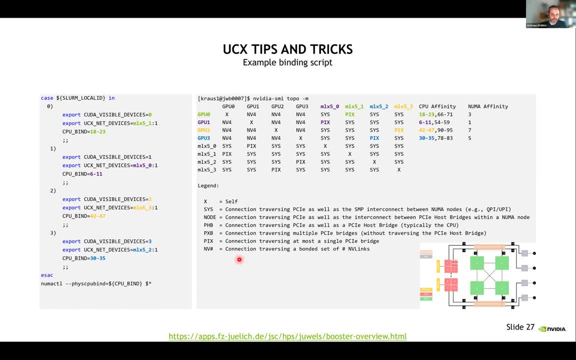 Thank you. This is a great resource. Yeah, That's effectively what the job scheduler does. It generates a launcher script like this, And then I'm not sure, And then I'm not enough into resource managers like Slurm to provide any more tips like that. 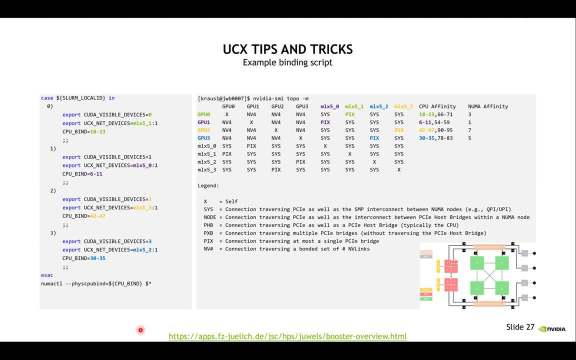 Thank you Well, barring no further questions, I want to thank Jiri for his time today and offering his expertise on multi-GPU computing, especially with the time change all the way to Germany, So I appreciate you staying on late in the day for us. 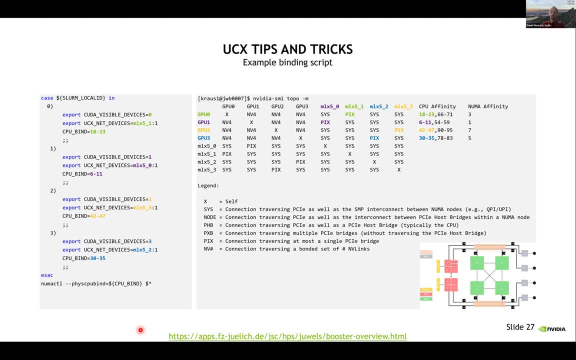 Our next session in the GP workshop at NCAR will be an interactive session focusing on some hands-on work implementing some of these techniques we learned today, So look forward to that in our next session two weeks from now, If you have any follow-up questions. 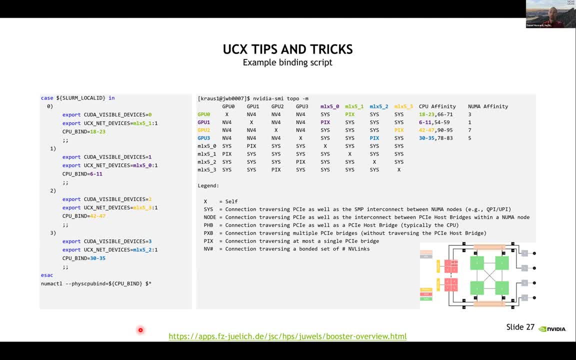 feel free to message us in the Slack, And if you would like to have a follow-up question with Jiri, feel free to send that to us. We can forward that along as needed. Thanks again for everyone's time today, And I'm going to wrap it up.